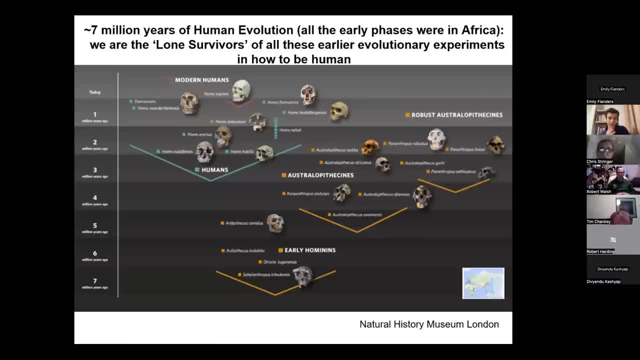 we come very late in the story, So this is from our exhibition at the Natural History Museum in London, And so we've got there. about 7 million years of hominin evolution represented the first 5 million years or so, happening, as far as we know, only in Africa, And then in the last 2 million. 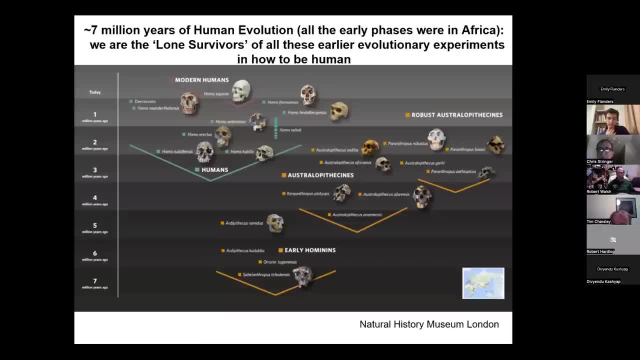 years or so we get humans emerging from Africa. the genus Homo, and our own species, of course, comes in very late in the story, arguably within the last one million years only, but we'll come on to the question of what we call Homo sapiens in a moment. So everyone agrees: there is only one. 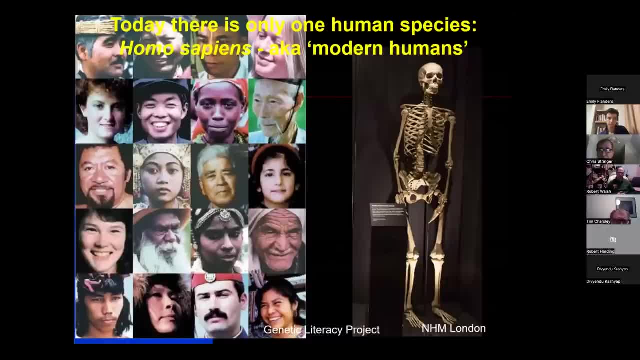 human species around today, us Homo sapiens, often called modern humans, and we come in many different sizes and shapes and colours around the world. but if we strip off those superficial features and get down to the skeleton, the bones and the teeth, we have a suite of shared features. 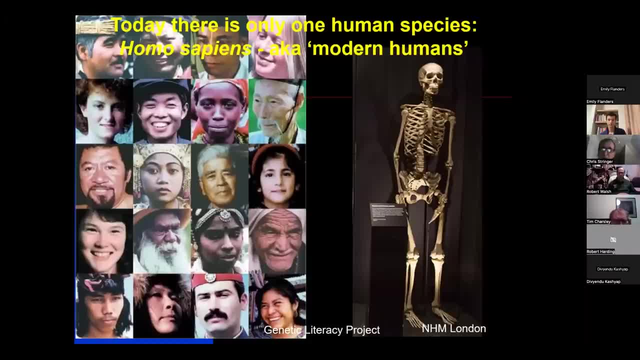 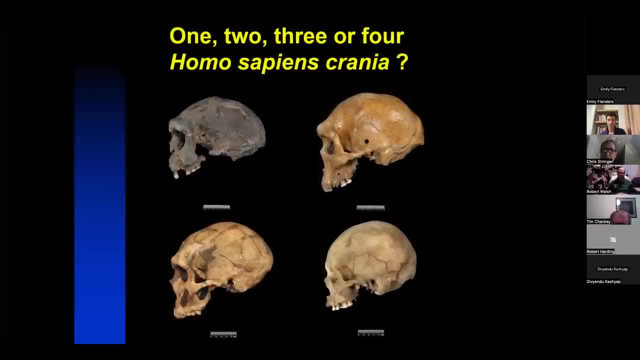 and those features are ones we can look for in the fossil record to map the evolution of these features of our species. And what is Homo sapiens in the fossil record? Well, it depends who you ask. so some people would say: only one of these craniae here is a Homo sapiens. others would say two of 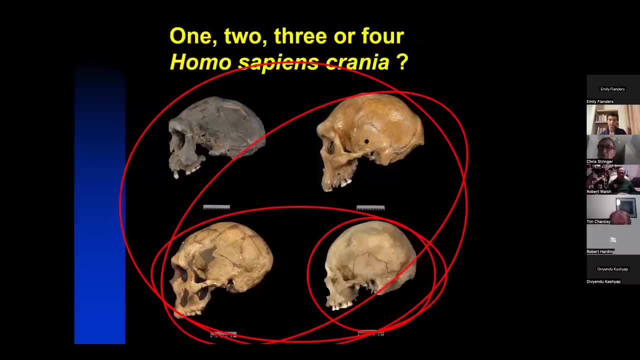 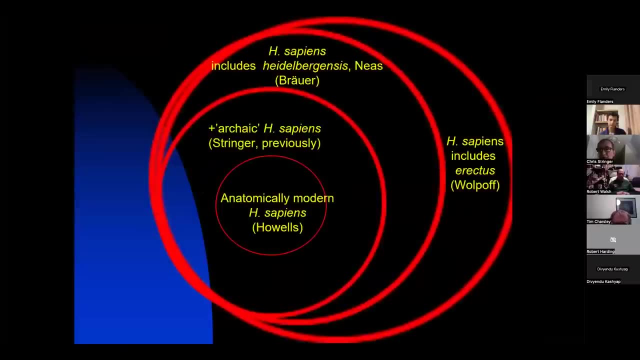 them, Some would say three, Some people would say all four should be called Homo sapiens. So this is a tricky matter even to begin with. And here are some of those different usages of Homo sapiens. The most restricted usage introduced by Bill Howells, anatomically modern. 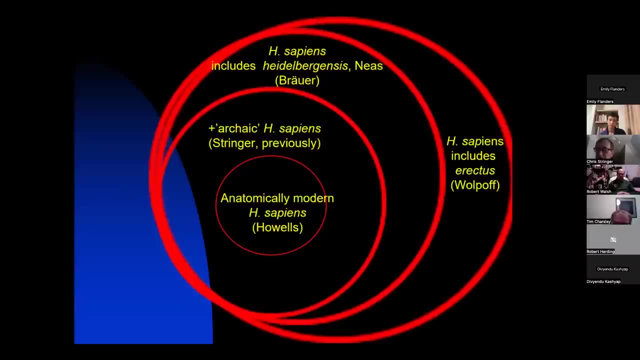 Homo sapiens At the end of his career. really he was saying that perhaps that should be the only Homo sapiens ones that really closely match our modern skeletal pattern. today I've tended to enlarge it further and including Homo sapiens, what I used to call archaic Homo sapiens. I'll come on to that a bit later. 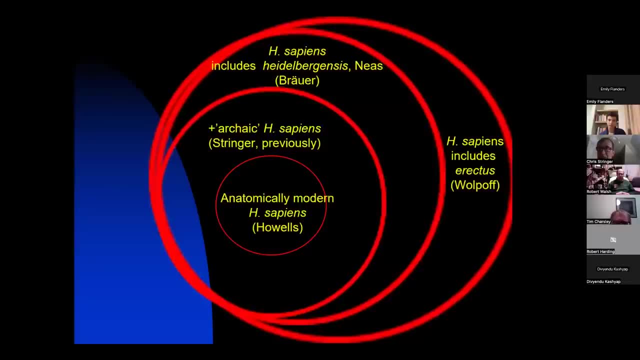 So a slightly larger definition of Homo sapiens. there Gunther Breuer has had an even wider definition, where he actually includes things that I would call Homo hydropagensis and Neanderthals within Homo sapiens, And then an even wider usage for people like Milford Walpoff. 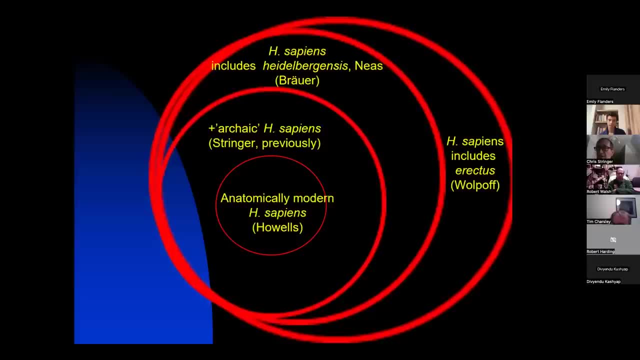 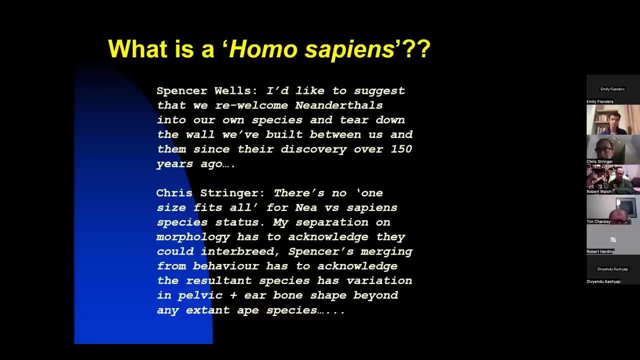 Of including things that that many of us would classify as Homo erectus. So a very wide definition covering most of the last 2 million years of the fossil record for people like Milford Walpoff And he. just to encapsulate some of that difference of opinion, This was a discussion. 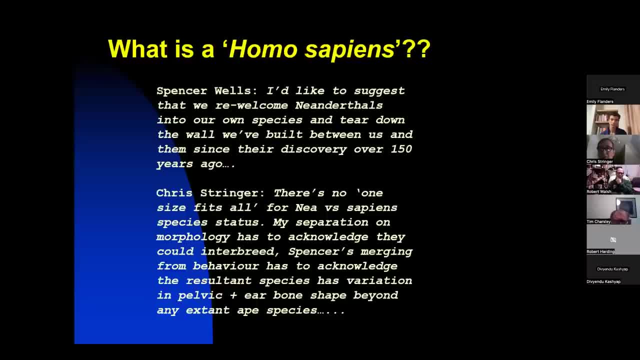 I had with Spencer Wells and I just transcribed it here. So Spencer Wells, the geneticist, said: I'd like to suggest we rewelcome the Neanderthals into our actual beleEDIE能 own species and tear down the wall we've built between us and them since their discovery over. 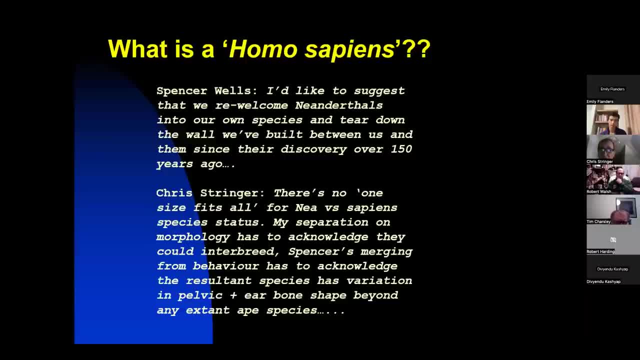 150 years ago. and then i've answered. well, there's no one size fits all for neanderthal versus sapien species status. my separation of them on morphology has to acknowledge that they could interbreed and spencer's merging from behavior has to acknowledge the resultant species has variation. 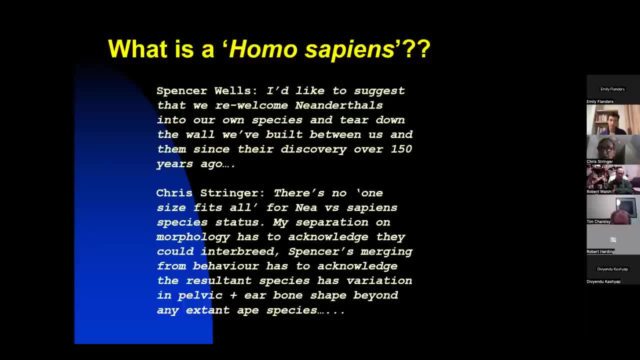 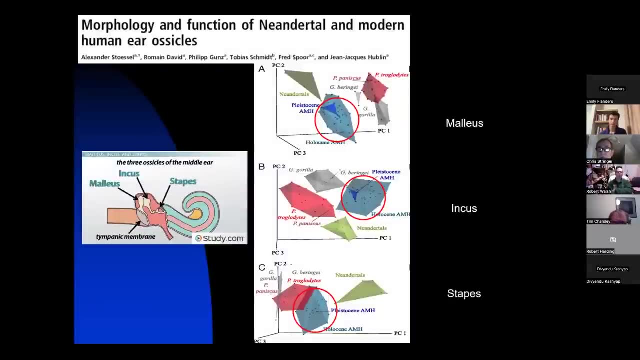 in pelvic and ear bone shape beyond that of any extent, ape species. so different ways of looking at how we define a species and how we apply that to homo sapiens, and just to focus on that point about ear bones. so here's a data from a paper by stursell and colleagues looking at the middle. 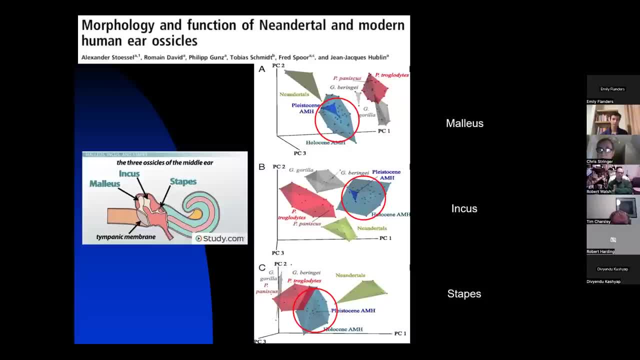 ear bones, three, these three tiny ear bones that help us in our hearing: in the middle ear: the malleus, the incus and the stapes. and here's a data from a paper by stursell and colleagues. here's their data showing the variation in homo sapiens, in neanderthals and in two species of 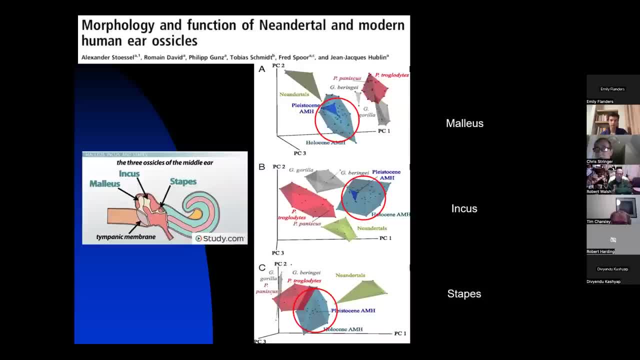 chimpanzee and two species of gorilla. so i've highlighted for each of the bones in in the red circle there: the homo sapiens group in blue, the neanderthal group is in green, the chimpanzee groups are in a sort of reddish color, the gorillas are in gray and you can see that. 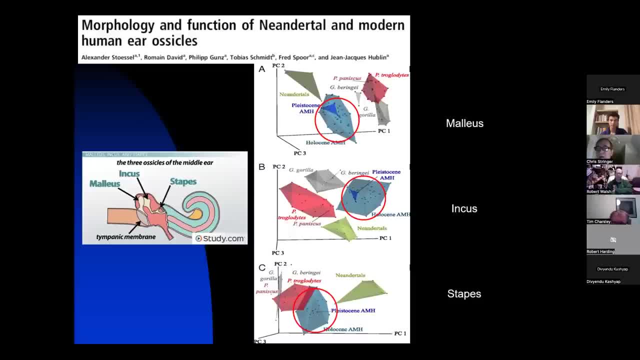 if we decided to merge the neanderthals and the homo sapiens groups for these inner, for these middle ear bones, um, not only would that variation exceed the variation we find in any single species of gorilla or chimpanzee mapped on there, but it would exceed the variation of all of them. you. 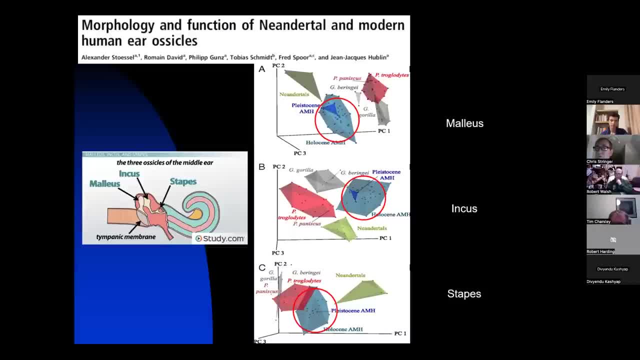 could merge bonobos, pantroglodytes, the two gorilla species, into one great big super species, and the variation of their middle ear bones, uh, would be only the same, or perhaps even smaller, than if we combine neanderthals and homo sapiens. so the variation in just these tiny little bones? 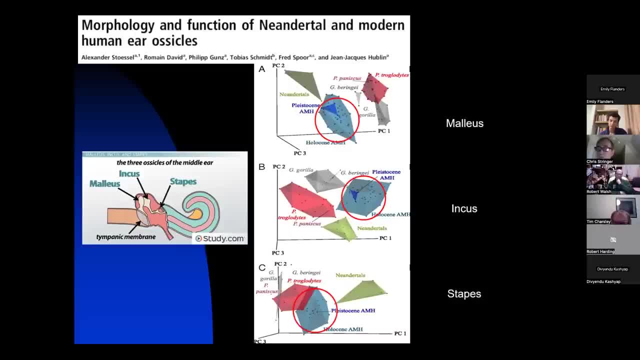 shows us that neanderthals are distinct from homo sapiens, and we've got even fossil homo sapiens in that group as well. pleistocene homo sapiens are also in that blue grouping there. so, yeah, even on these tiny little ear bones, um, we've got a lot of homo sapiens in that group as well, and we've got. 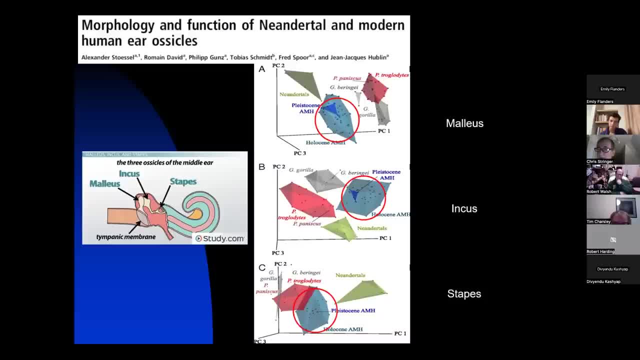 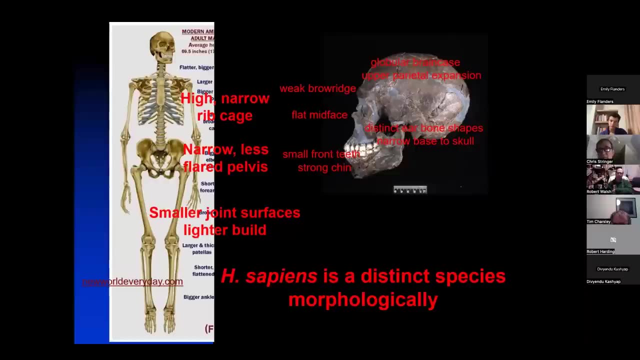 you really would create problems. if you merge us and the neanderthals together as a single species, the variation will be greater than we are finding in any of these ape species. so i would say we are a distinct species. morphologically, we can see that in our skeleton features, such as the high narrow rib cage, a narrow, less flared. 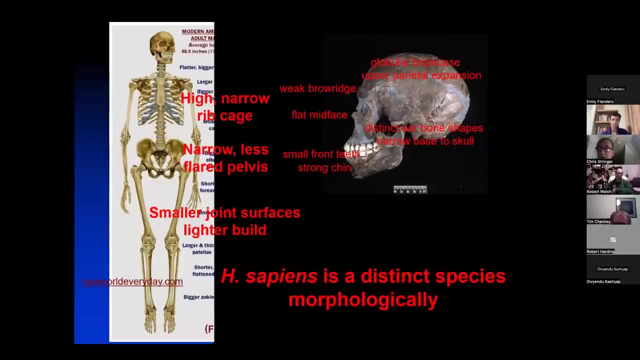 pelvis, a lighter build in the skeleton generally and also a number of features in our craniums and mandible. you can see there that the globular brain case a weak brow reach or non-existent brow reach, a flat midface, those distinct ear bone shapes we mentioned, a strong chin on the lower jaw, even in 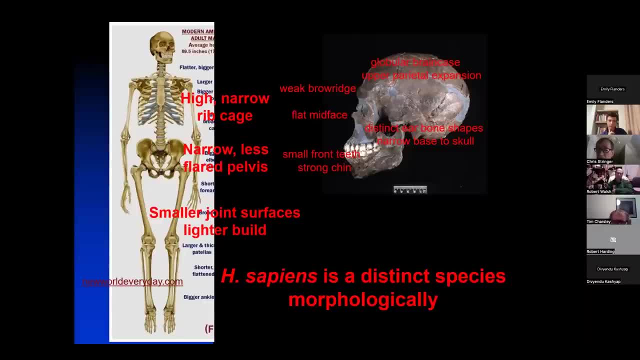 very young children. so i would argue that this, this suite of features we can look for in the fossil record to try and recognize our lineage, homo sapiens. a bit of ancient history now, going back to the time i was doing my phd in 1970, i was doing my phd in 1970 and i was doing my phd in 1970. 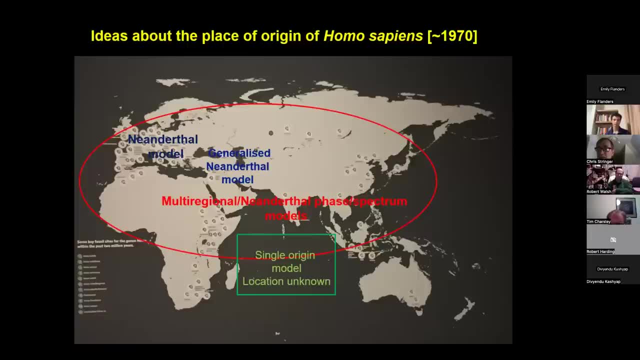 i was doing my phd in 1970 and i was doing my phd in 1970 and i was doing my phd in 1970 and i was doing. There were many different views about where Homo sapiens had originated, but none of them really argued that Homo sapiens had originated in Africa. 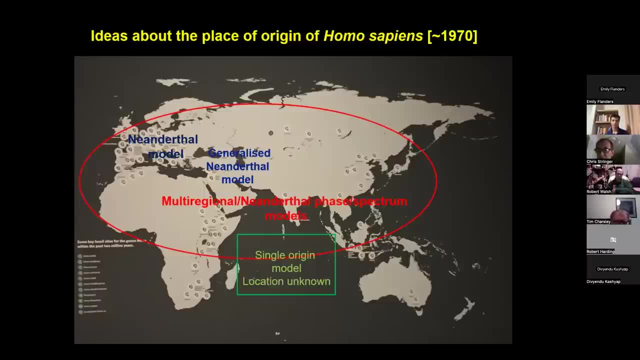 There was obviously a view that ancient the human line may have originated in Africa, But for Homo sapiens the origin was usually placed outside of Africa. So we had models such as the Neanderthal model of people like Hrlicka arguing that it could be a European origin for Homo sapiens. 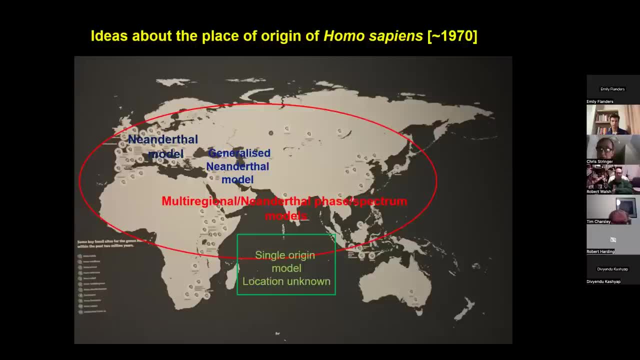 Clark Howell. in the 1950s Clark Howell argued that the generalized Neanderthals of Western Asia could have been the source of Homo sapiens evolution, And then they migrated from there into Europe and to other regions, So a sort of Western Asian model. Christy Turner on dental data. 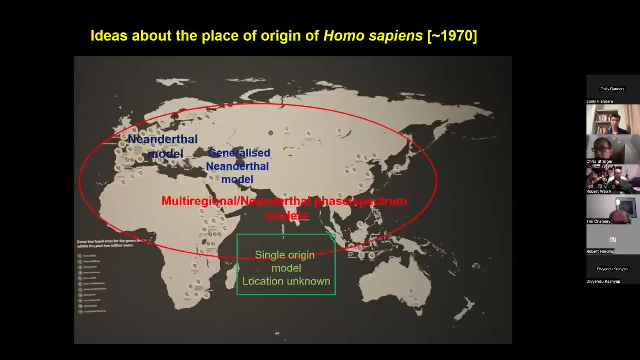 Around 1990 argued that we had a Southeast Asian origin for Homo sapiens. There were multi-regional or Neanderthal phase models which argued that there was really a global origin for Homo sapiens across the whole of the inhabited world during the Pleistocene. 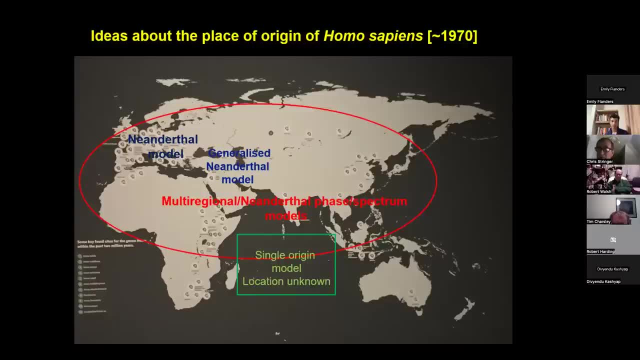 So there would be local ancestors for Homo sapiens in Europe, in China, in Indonesia and in Africa. So many different views. There were a minority of people who argued that Homo sapiens had originated in Africa. There were a minority of people who argued that Homo sapiens had originated in Africa. 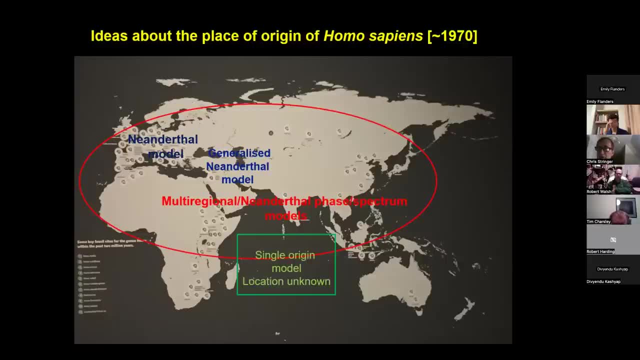 There was even a few people who argued for a single origin model with a location that was unknown, So Bill Howells was one of these. He argued that Homo sapiens morphology was so distinctive that it probably did have a fairly recent and local origin. 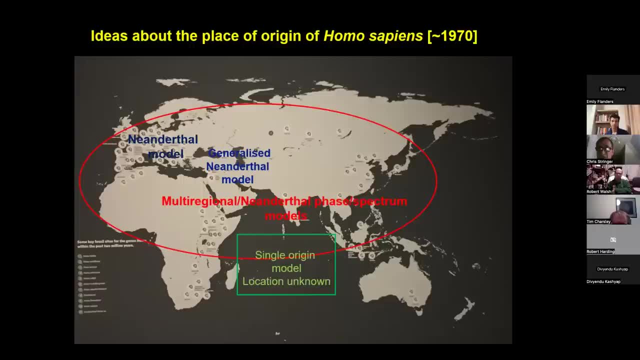 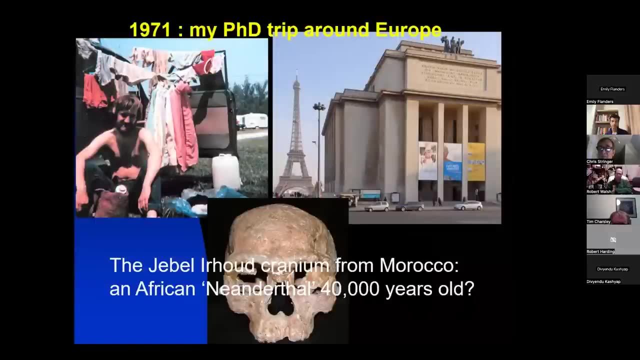 But he certainly couldn't place in the 1960s and 70s where that origin was. And for me, as I began my PhD trip around Europe in 1971, I was going to compare Neanderthal crania and Homo sapiens crania and by the time I got to Paris there was this, at that time, wonderful. 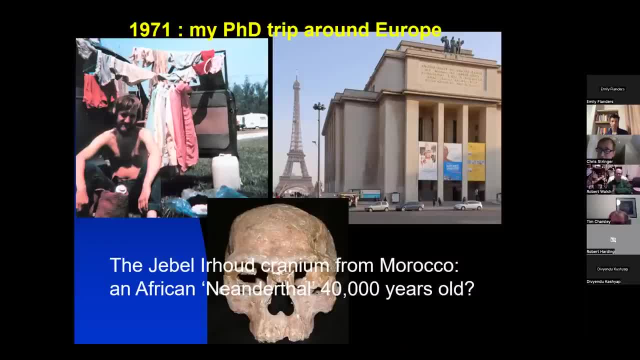 fossil in Paris from Jebel Ehud in Morocco- now back in Morocco. but at the time, you know, when I saw it, I'd been told that it was an African Neanderthal and I could see that it certainly wasn't at all Neanderthal like, but at that time it was dated at about 40,000 years old. 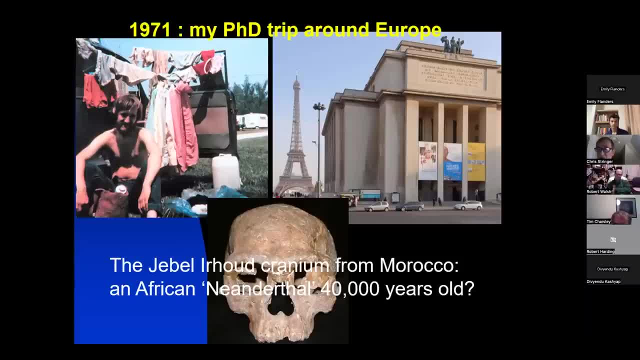 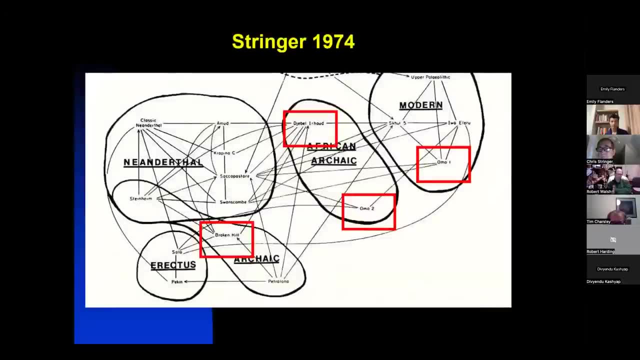 so it really didn't make a credible ancestor for Homo sapiens when it seemed to be so young in age and my PhD results- and this is a diagram summarising those results- in 1974, so I was able to show that Neanderthals and Homo sapiens were quite different in cranial 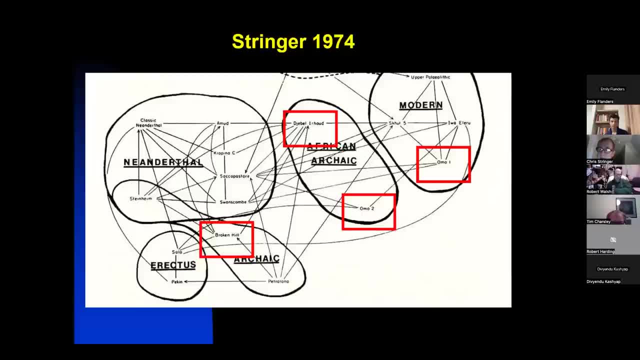 morphology, cranial shape, and the Neanderthals seem to be going off in their own evolutionary direction in terms of cranial shape, compared with Homo sapiens, but the African fossils, as you can see, are not, and they're in these red rectangles- were quite diverse in their 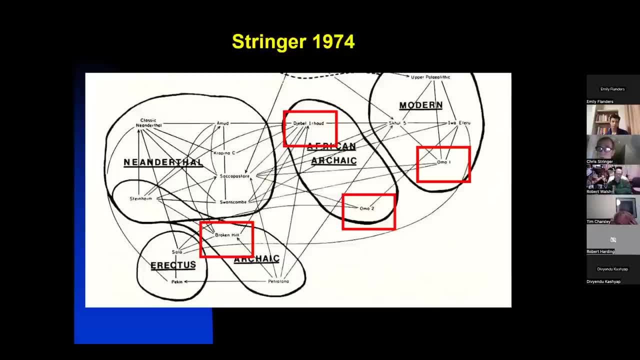 evolution in their, in their cranial shape and in their affiliation. so the broken hill fossils seemed quite primitive. the omokibish one specimen, on the other hand, was really seemed to me a homo sapiens, even modern type, on the data i had. and then there were fossils such as jebel, ikhud and omokibish. 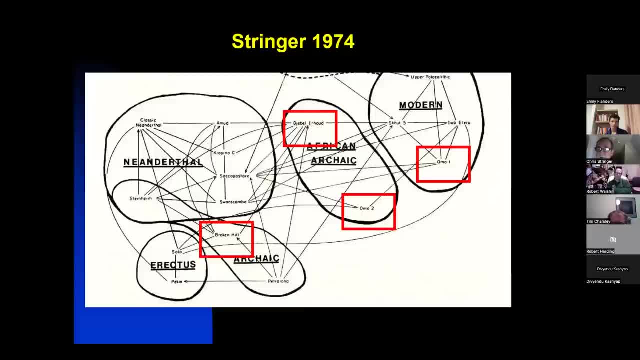 two which didn't really fit into any of these other categories. in some ways they look kind of intermediate between the more primitive fossils and homo sapiens. but, as i mentioned, a fossil like jebel ikhud at 40 000 years old didn't seem to be. it didn't seem it could be a credible. 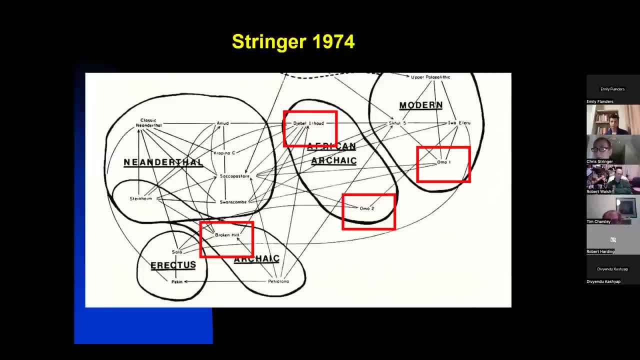 ancestor of homo sapiens, with homo sapiens fossils such as the ones from shkul in mount carmel in israel, apparently around the same age and looking much more modern. so in 1974 i certainly couldn't make an argument for a recent african origin for homo sapiens. 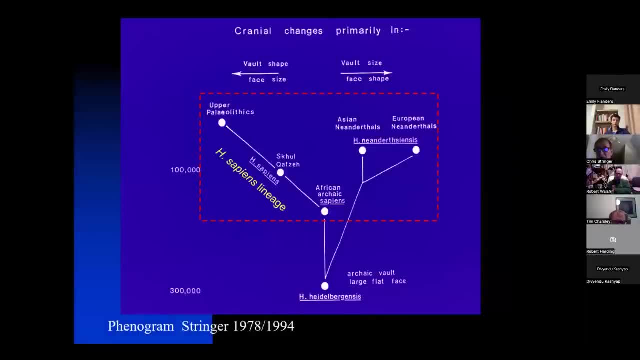 but i started to develop that view along with other people, such as gunter breuer, and here's a diagram, a version of it in fact, from 1994, where i developed this view of kind of two main trends in in later: plasticity and human evolution from something like homo heidelbergensis. 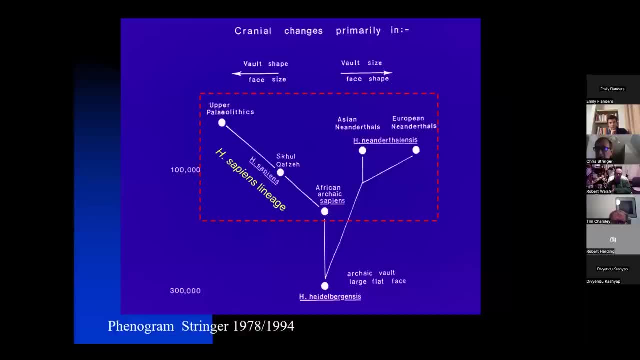 we have a a trend towards the neanderthals, with the main changes being in things like facial shape. and then we have a trend towards the neanderthals, with the main changes being in things like facial shape, and then we have a trend towards homo sapiens, beginning in africa, then proceeding. 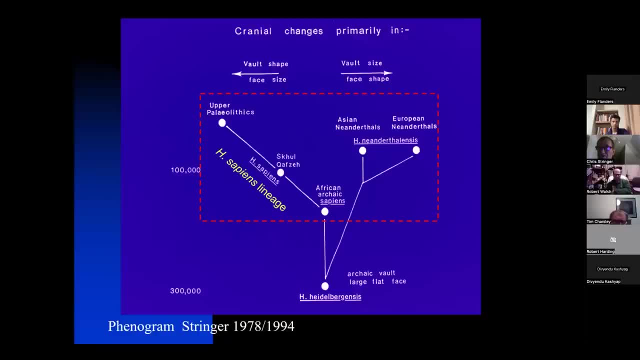 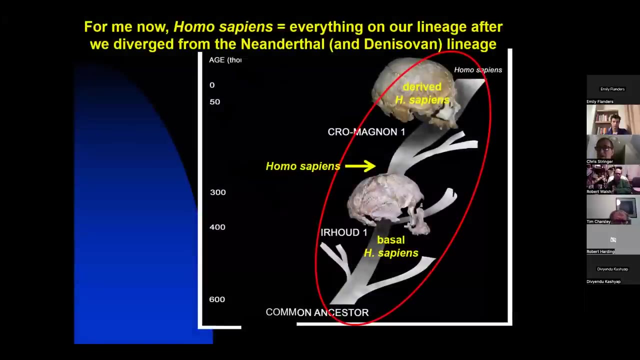 through fossils like shkul and kafse to the later versions of homo sapiens. so there is a homo sapiens lineage going back in africa more than a hundred thousand years. so in my current view, um, yeah, i, i regard homo sapiens now as being this lineage. 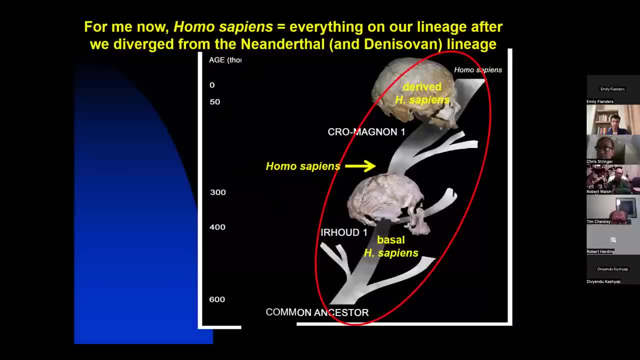 after we split from the neanderthal and denisovan lineage. so for me, jeb leahood is probably a homo sapiens, an early homo sapiens, but because there's evolution along this homo sapiens lineage, um, rather than now say you know, archaic and modern. 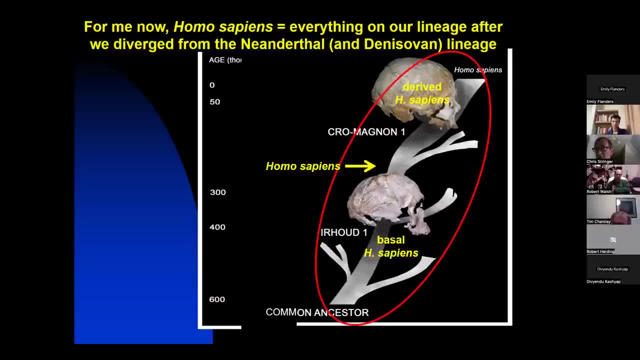 i've you try and use a new terminology, which is to argue that the later forms of homo sapiens are derived. they show evolutionary novelties, whereas the early forms, such as jeb, leahood- i call them basal. they're closer to that split with the neanderthals and denisovans. they show more primitive features. 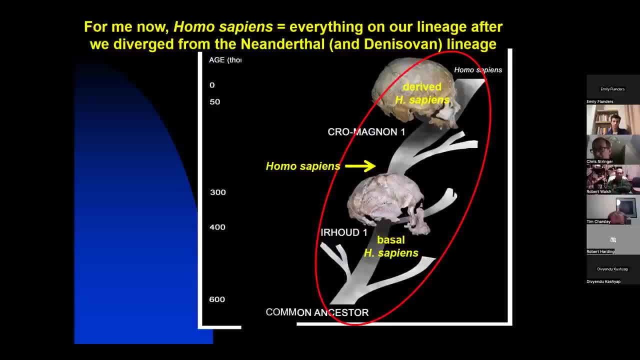 and of course this is, you know, these are, these are relative terms. how do you decide what's basal and what's derived? and you have the same problem with deciding what's going to be archaic and what's going to be modern. but at least for basal and derived, you know, i can sort of point to a phylogeny. 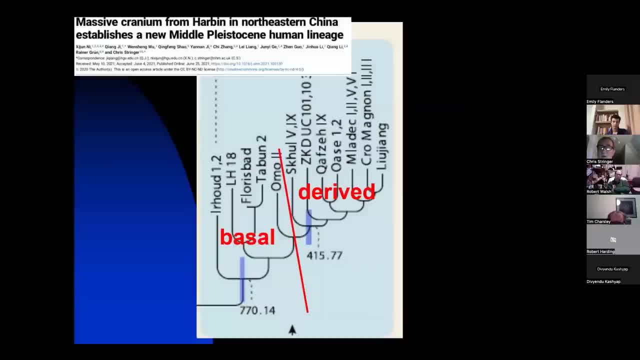 such as this one from my paper with colleagues on the harbin cranium from a couple years ago, where we developed a phylogeny based on cranial traits, and this is the one for homo sapiens. and here i've made a division. again, it's a subjective one. my opinion of where i would place this basal derived. 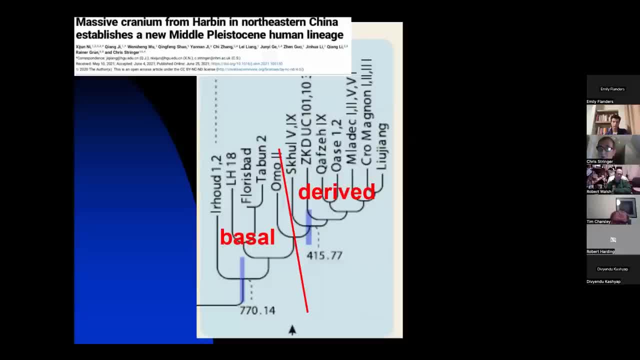 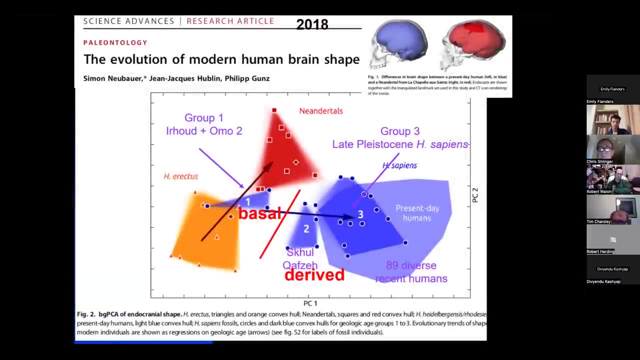 division on this phylogeny. so fossils like ehud and homo2 are basal in the homo sapiens evolution uh, fossils like kafse and mladech and so on are derived homo sapiens and you can make the same sort of division on this uh study from neubauer and colleagues on modern human brain shape. so here we've got a. 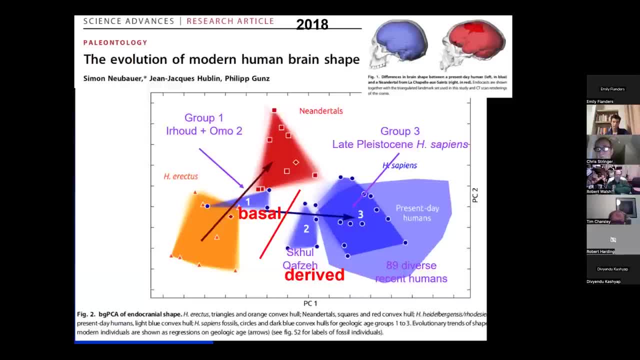 group of fossils and recent samples. you've got the erectus fossils in orange, the neanderthal fossils in red, the present-day homo sapiens in mauve on the right-hand side there, and we've got three groups of fossil homo sapiens: one, two and three and you can see that ehud one and uh sorry. 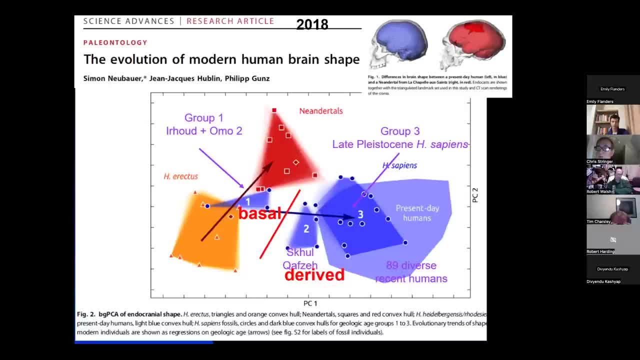 neanderthals in the upper left-hand side, in the lower right-hand side of this picture and below that, in this case one and two are more close to the neanderthals in having a long, low endocranial shape and a lot of bumblebees. 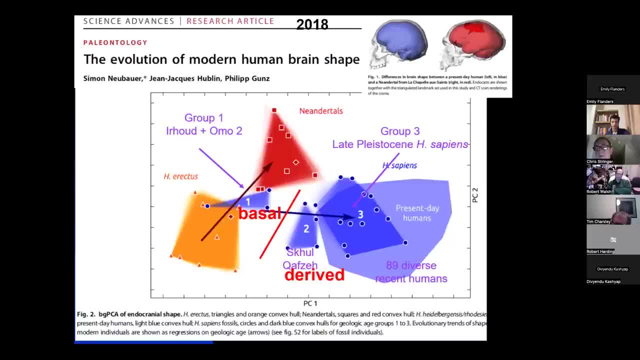 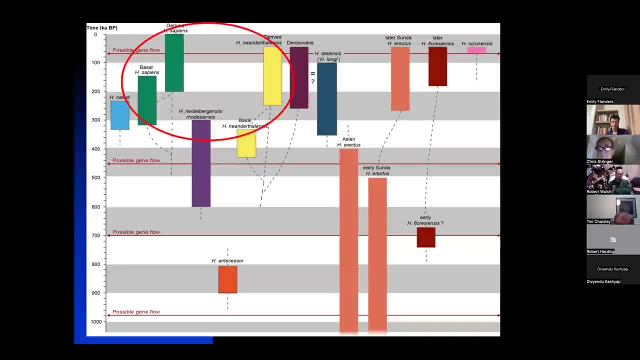 we're. Yang guo and ramo 2 are much closer to erectus and neanderthals in having a long low, and Hublan and Gunz is group one and group two, So let's home in on that sapiens-neanderthal relationship. 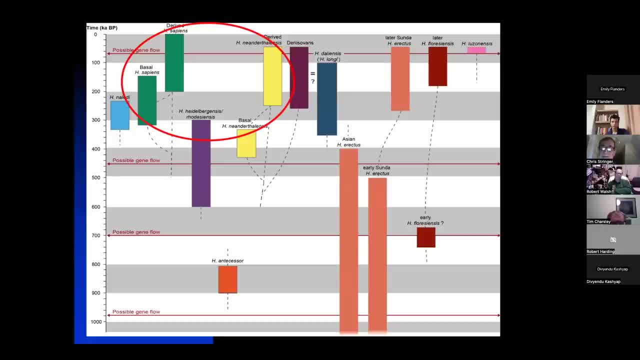 Of course we've got here a representation of the last million years or so of human evolution, So a number of different coloured bars here representing different lineages through time. I would argue that many of these are different species, But in green we've got the Homo sapiens representation. 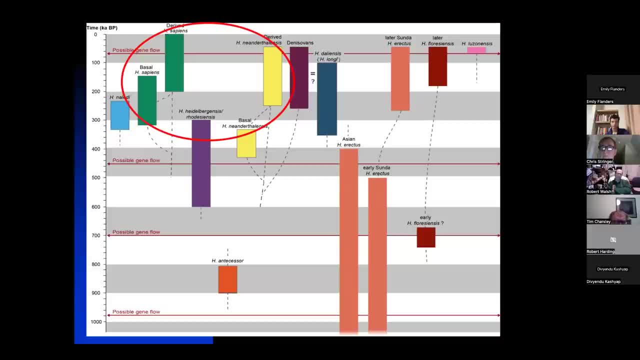 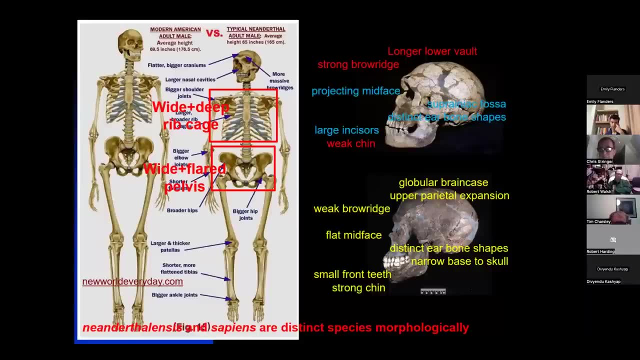 and in yellow we've got the Neanderthal representation. So for Neanderthals, yes, I would say that morphologically there's very good evidence that they represent a distinct species. We mentioned the middle ear bones, the inner ear bones. 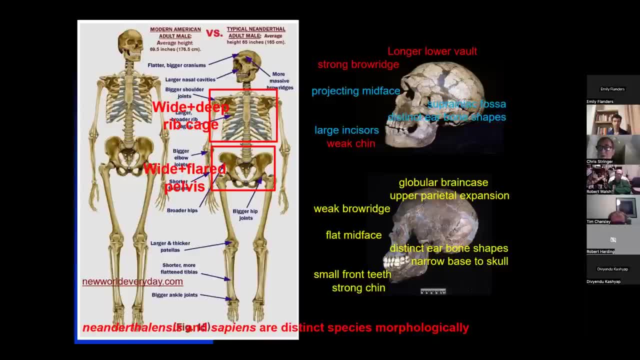 show the same distinctions. In the skeleton we've got distinct ribcage and pelvic shape. In the cranial vault we've got primitive features that are shared with earlier humans, such as that longer low brain case, a strong brow ridge above the eyes. 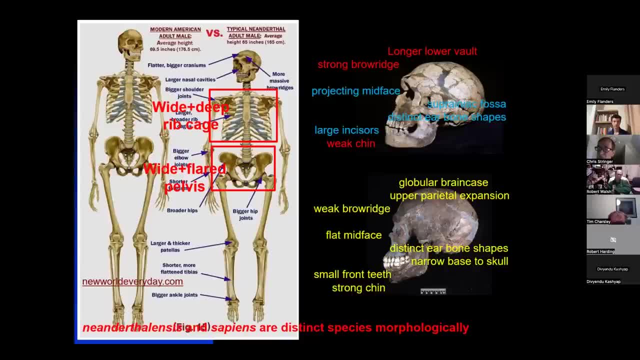 a weak development of the chin. But also they've got their own distinctive features, such as that projecting midface, a superiniac fossa on the occipital bone, distinct ear bone shapes- we've mentioned that already- large incisors at the front. 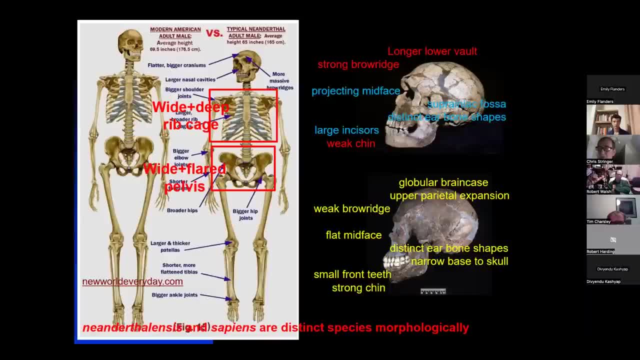 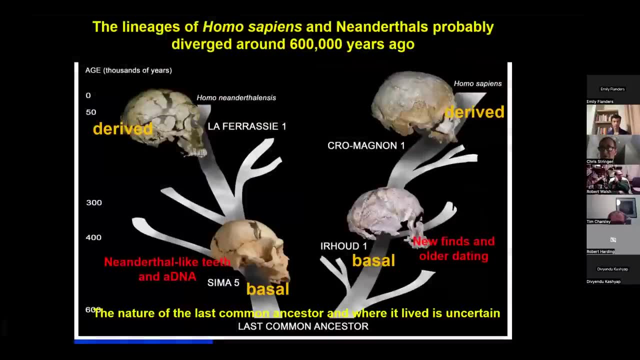 So for me there's enough data here to place the Neanderthals as a distinct species morphologically, And we can trace Neanderthal evolution through time as well. So here a simple representation. we've seen the Homo sapiens lineage on the right-hand side there. 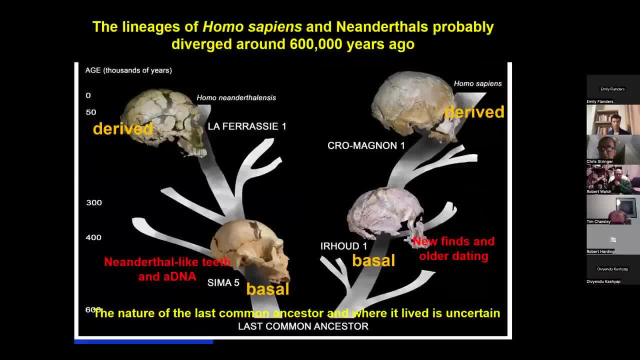 and we can trace the same sort of evolution back in time for the Neanderthals, back towards a common ancestor with the Homo sapiens lineage. So fossils like the Seminal Huesos ones for me are basal Neanderthals. 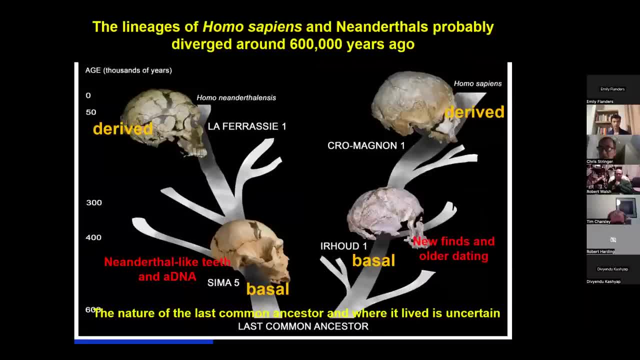 They have some very Neanderthal features in their teeth, for example, and we even have ancient DNA from a couple of bits of fossil from the Simondel Huesos, dating from over 400,000 years old. It's the oldest human DNA yet. 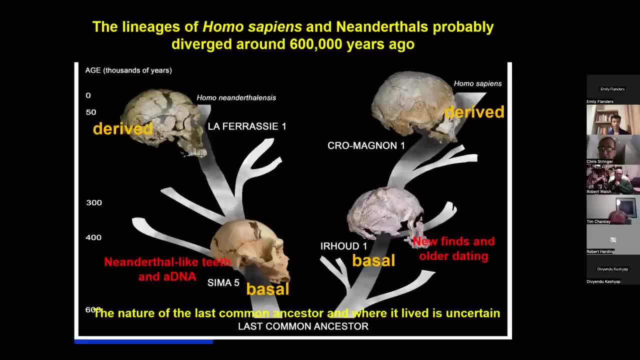 recovered, and that places them also on the Neanderthal lineage. And I'm now much less confident about who that common ancestor was. I used to think it was Homo heidelbergensis. Now I don't know who the common ancestor is, and I don't even know where that common ancestor lived. 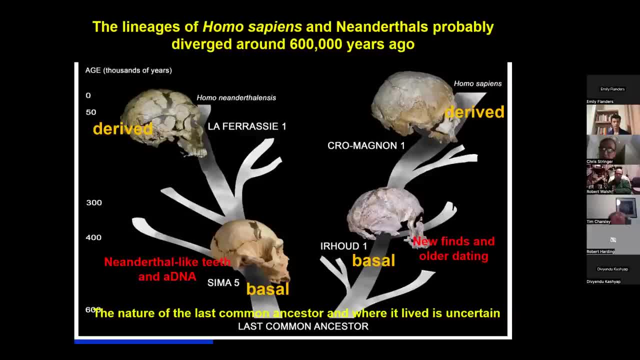 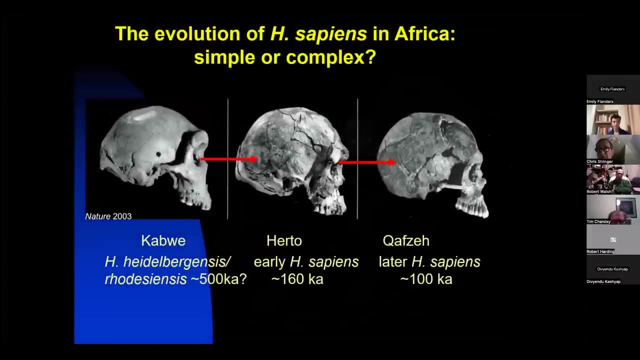 The ancestor may have lived in Africa, but equally it could have lived in Asia, could have even lived in Europe. So I think this is work for the future. Geneticists estimate the common ancestor probably lived around 600,000 years ago. So in the past we've had these really quite simple views and I at times subscribe to them. 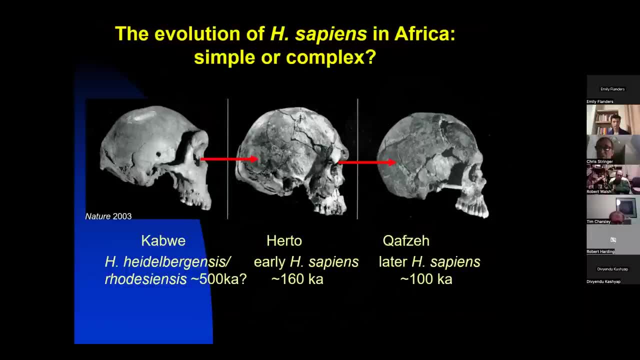 as well, that we had a gradual evolution of the Homo sapiens lineage, perhaps even in one, just in one area of Africa, probably East Africa, And here is a representation of that from nature from about 20 years ago when the Herto fossils were published. You can see there. 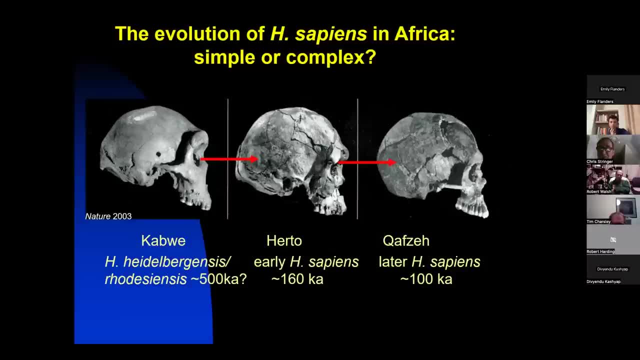 Cabway, the Broken Hill fossil there on the left representing Heidelbergensis or Rhodesiensis, estimated to be about 500,000 years old. We've got the Herto fossil, Herto 1- there, about 160,000 years old as an early Homo sapiens, and then one of the Capsa fossils as a later 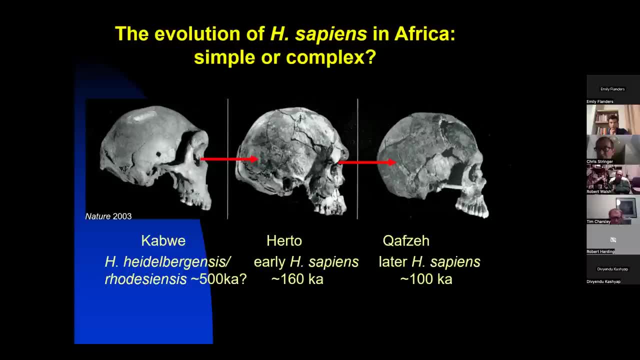 Homo sapiens. And here the suggestion of a gradual evolutionary change, with Herto being sort of in the middle of the Neanderthal lineage, and then one of the Herto fossils, and then one of the Neanderthal lineage, and then one of the Herto fossils and then one of the Herto fossils. 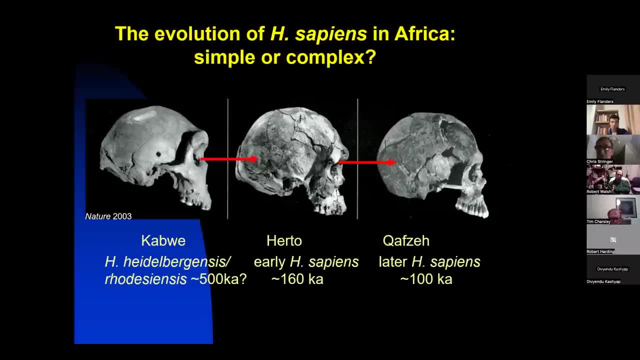 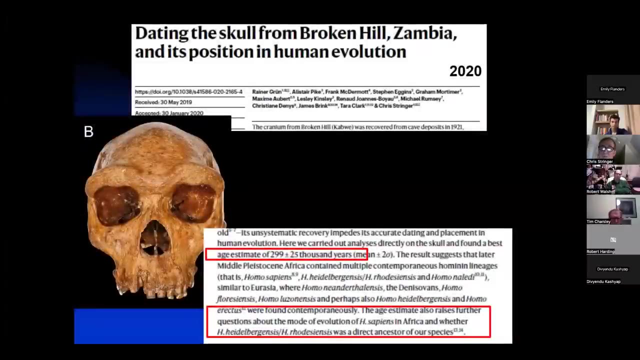 intermediate in some ways between the Heidelbergensis Rhodesiensis fossils and the later Homo sapiens fossils. So this view of a simple, unilinear, gradual evolution of Homo sapiens fossils- But something like Broken Hill- now has been reassessed and this is work. I did a couple of. 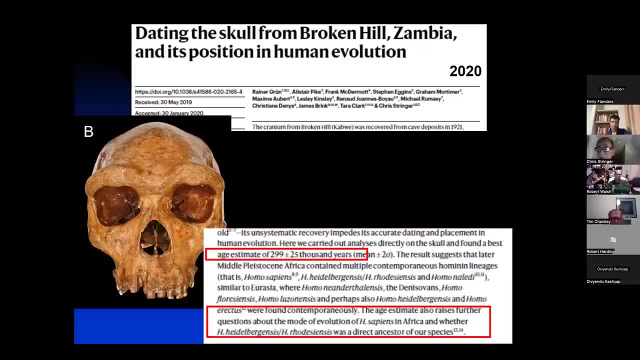 years ago with Reiner Grill and colleagues, where we attempted to date the fossil And of course, unfortunately, the original find site has been completely mined away. So we had to go back to the cave and we had to dig into the ahead of the cave and then dig in a bit more and then dig in a 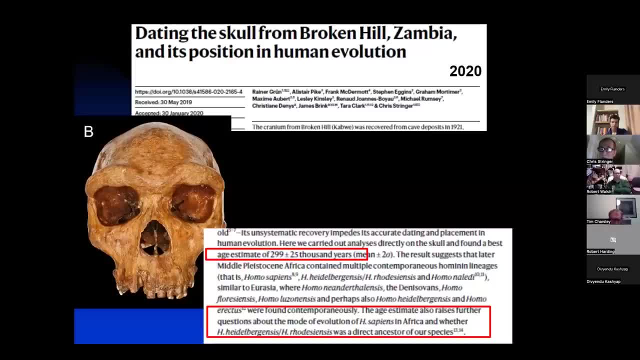 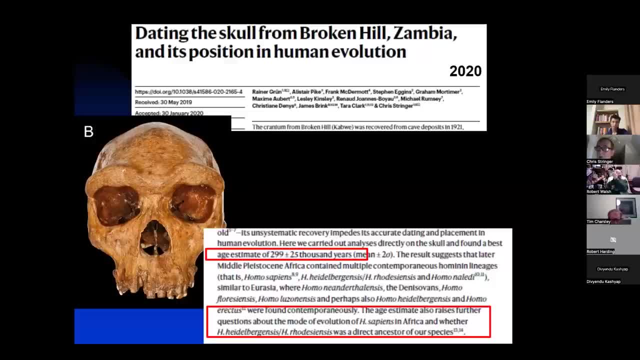 sediments from the cave and fossils of animals and the human fossils from the site. to try and date it- And this is the conclusion of our paper- We found a best age estimate of about 299,000 years for Broken Hill 1, for this fossil and, as it says here, this age estimate raises further. 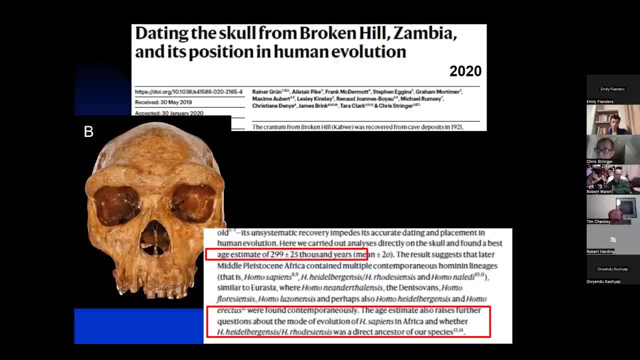 questions about the mode of evolution of Homo sapiens in Africa and whether the Hedobergensis Rhodesiensis was a direct ancestor of our species and as we'll see these. you know this doubt comes about because we have a younger age for heidelbergensis fossil, but also because we have older ages for homo sapiens fossils, but also 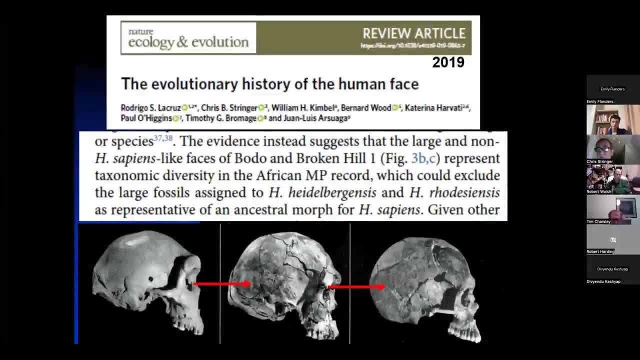 morphologically because work. i was involved in studying the faces of these fossils. this was published in 2019. looking at the evolutionary history of the human face and, as we say here, the evidence instead suggests that the large and non-sapiens like faces of bodo and broken hill. 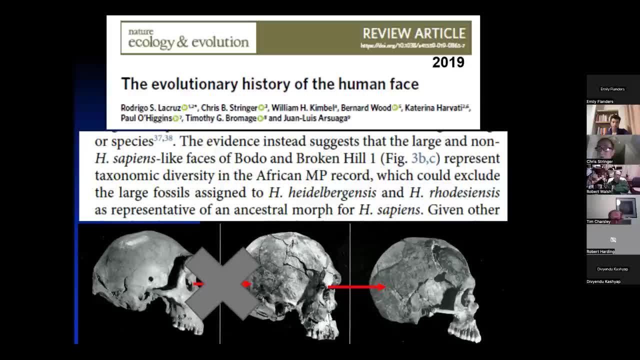 represent taxonomic diversity in the african middle pleistocene record, which could exclude the large fossils assigned to heidelbergensis and rhodesiensis as representative of an ancestral morph for homo sapiens. so there are derived features in the faces of these big heidelbergensis. 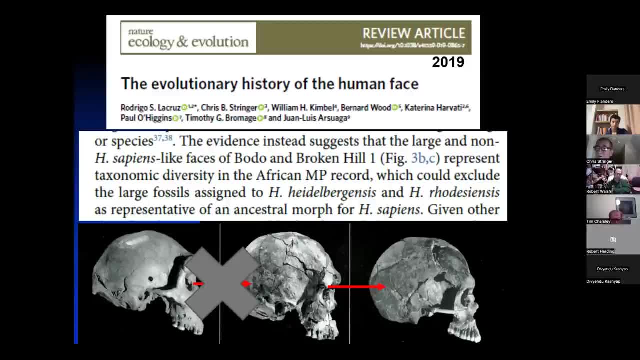 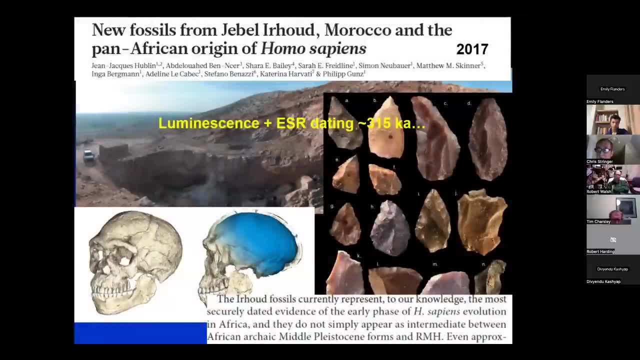 or rhodesiensis, specimens that take them away from the inferred ancestral position for us and the neanderthals, and we've also got earlier dating of the homo sapiens lineage. so this is this great work that was published in 2017 by hublan and colleagues- in fact, two papers published on 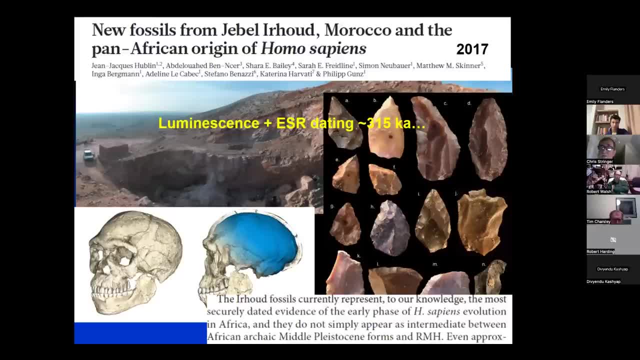 the morphology of old and new fossils from the jebel ihud site in morocco and new dating of those fossils and the associated archaeology- so beautiful middle stone age archaeology there and the evidence now that from luminescence in esr dating that these fossils are about three hundred thousand years old, so not forty. 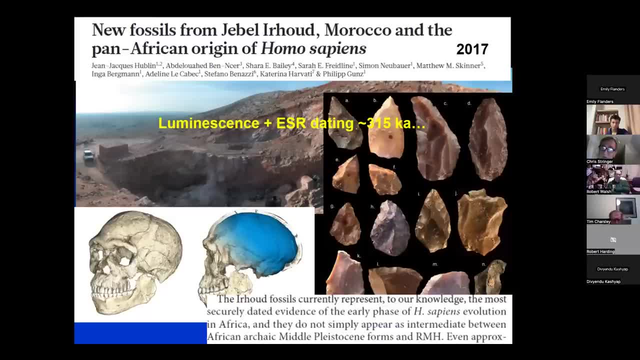 thousand years old, as uh as as people believed in in 1970, and so at that date this certainly could be an early member of the sapiens lineage. and, as it says here, the ehud fossils currently represent, to our knowledge, the most securely dated evidence of the early phase of homo. sapiens evolution in africa, and they do not simply appear as intermediate between african, archaic and egyptian fossils. the ehrid fossils represent, to our knowledge, the most securely dated evidence of the early phase of homo sapiens evolution in africa, and they do not simply appear as intermediate between. african archaic fossils or Order of the Homo sapiens and other first ever forms of Japanese evolution through their general evolution and their evolution throughout the 20s and 30s, and みたい to the literature that these fossils indicate a change in a way that is alien to the 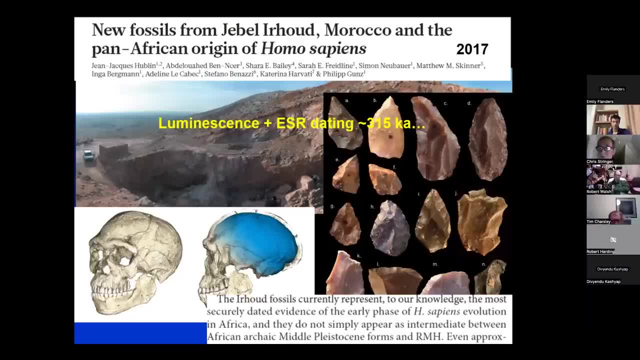 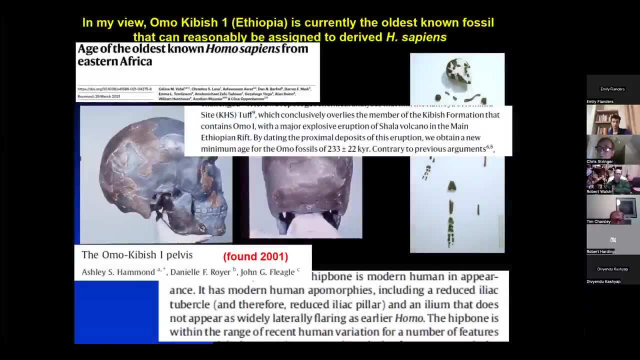 african archaic middle processing forms and recent modern humans, and even the morphology of what i would call derived homo sapiens is going back in time. so this uh, partial skeleton from omokibish, omokibish one in ethiopia, um, found back in. 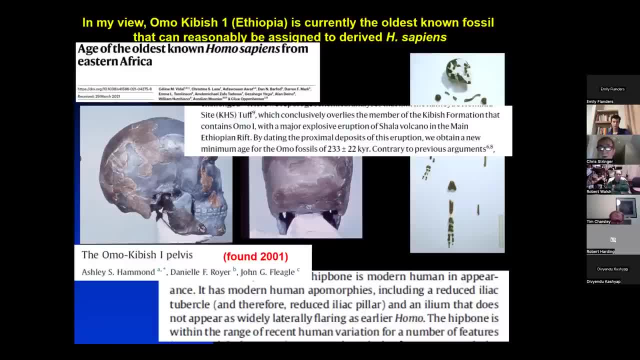 the 1960s by a team led by richard leakey um and recognized from even from my phd work and michael day's work, as representing what seems to be a something close to a recent homo sapiens pattern in the shape of the brain case. it's certainly incomplete, but the back of the cranium. 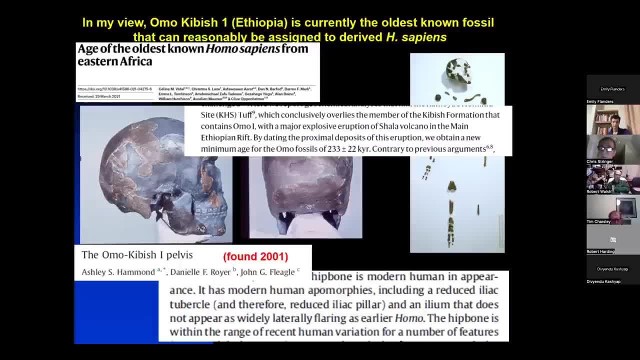 is high and rounded. there's a small divided brow ridge. there's a chin on the lower jaw and more recent work has discovered more of the skeleton, including parts of a pelvis, and, as it says here in this paper by hammond and colleagues, the pelvis has modern human apomorphies, including 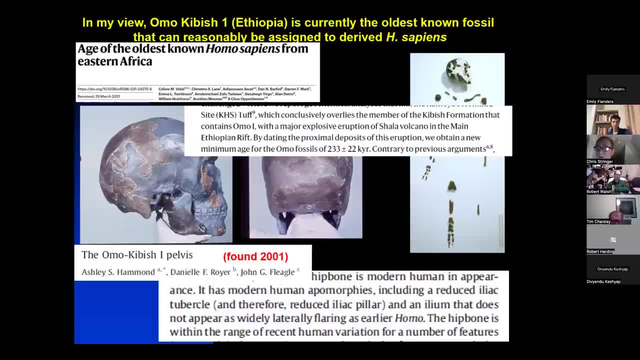 a reduced iliac tubercle and an ileum that does not appear as widely laterally flaring as earlier homo. the hip bone is within the range of recent human variation for a number of features, and recent dating work has pushed the dating of this fossil back even further. as it says here, by dating the 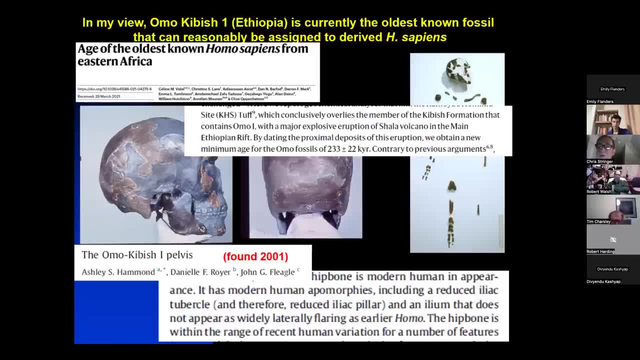 proximal deposits of this eruption, we obtain a new minimum age for the homo fossils of about two hundred and thirty three thousand years. so this fossil is pushed further back in time and therefore the homo sapiens lineage and the derived features go further back in time. but when we look at the whole of the african record for this period from about 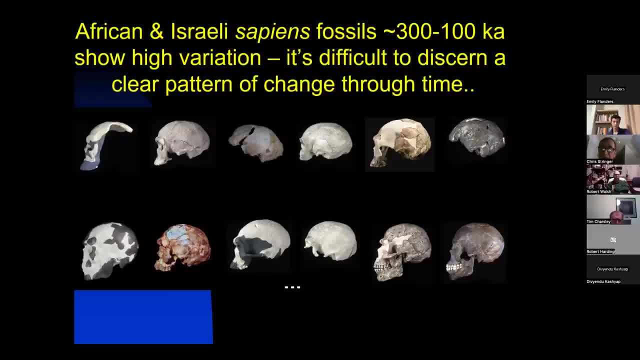 one hundred thousand to three hundred thousand years ago, and we add in the israeli fossils from school and cafe. when we look at them as a whole they do not show a nice, neat, coherent pattern of change through time where we see the gradual appearance and accumulation of these. 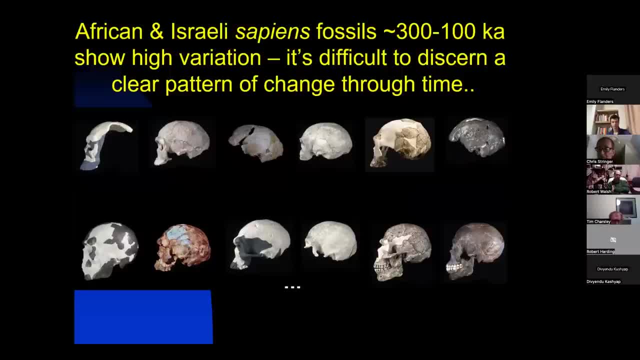 derived homo sapiens features. the features seem to be scattered around and we have fossils with mosaic morphologies, different mixes of basal and derived features, and it might be that maybe these fossils are not all in the well dated. and if they were well dated maybe things would form. 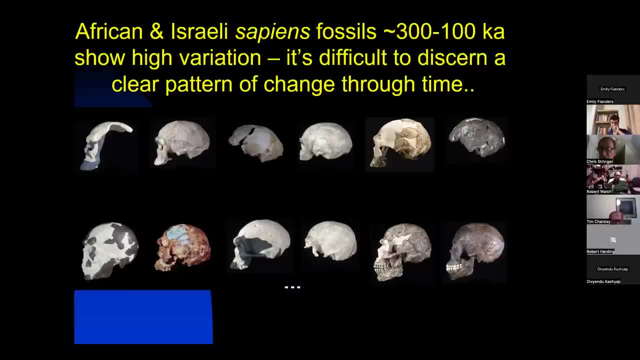 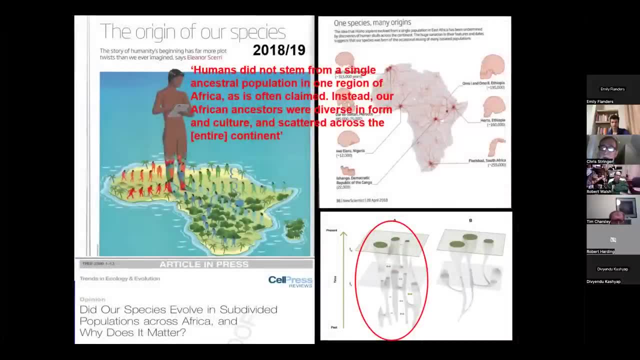 a more orderly sequence of the evolution of homo sapiens features. but at the moment it doesn't look that way, and so i and colleagues join with uh eleanor sherry in developing this idea of a pan-african origin for homo sapiens that we did not evolve just. 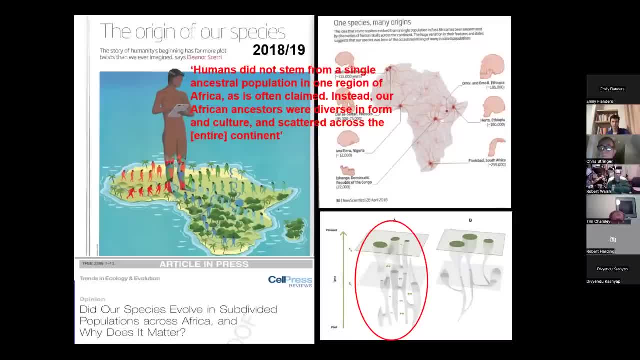 in one area of africa in a gradual way, but homo sapiens was assembled from populations over much of the african continent. so here's a quote from ellie. humans did not stem from a single ancestral population in one region of africa, as is often claimed. instead, our african 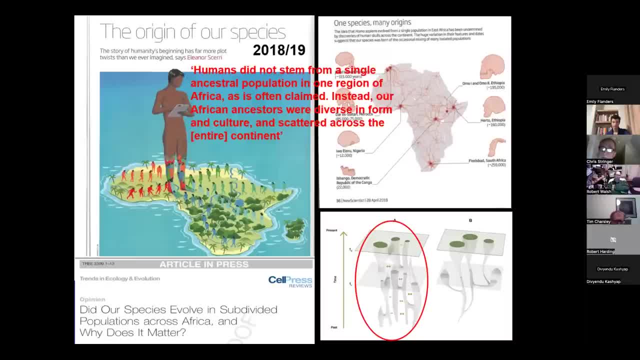 ancestors were diverse in form and culture and scattered across the- well, she says- entire continent, about entire, but certainly much of the african continent, and the model we're talking about is shown on the bottom right there that we have these lineages going through time. some of them go extinct. 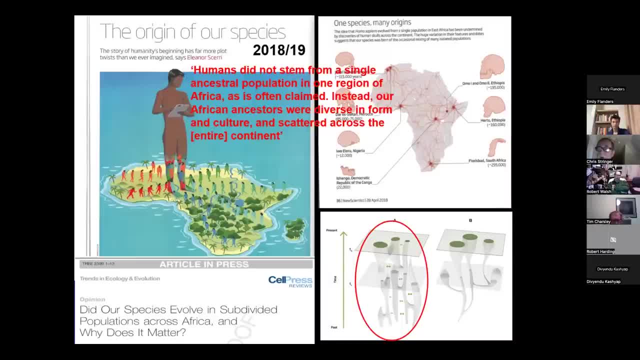 some of them go off in their own evolutionary directions, but when the climate of africa changes and allows mixture, these lineages exchange genes, probably exchanged ideas as well, and what we call derived homo sapiens is actually an assemblage emerging of these different lineages coming together from across different parts of africa. 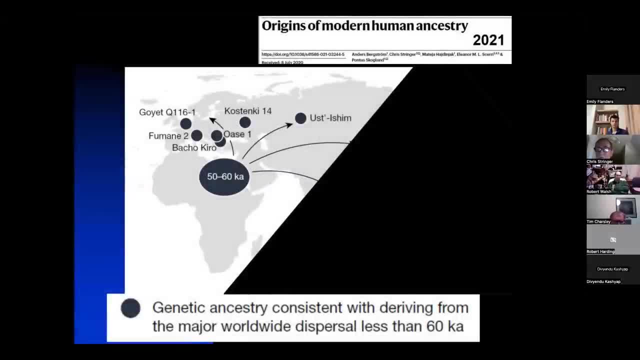 and there was a major event around 60 000 years ago, according to much genetic data, where homo sapiens undertook a significant dispersal from africa, stayed behind in africa as well, of course, and that dispersal out of africa formed the basis of the genetic 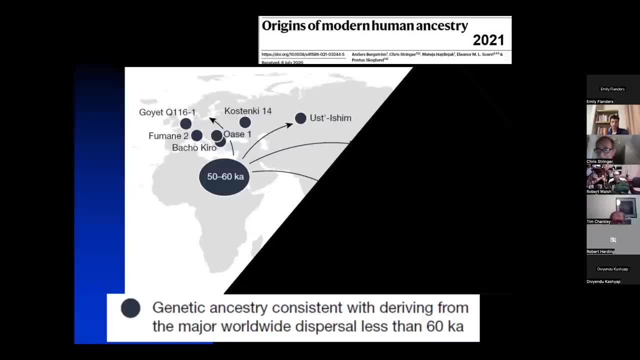 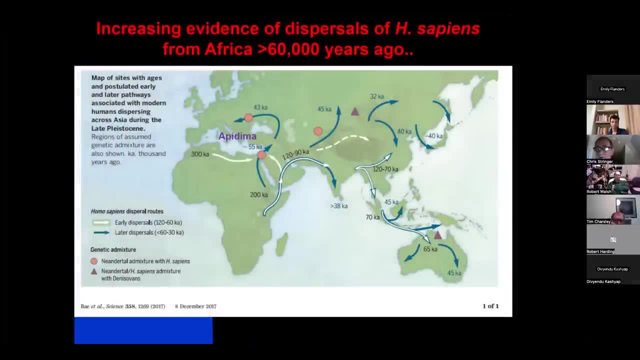 variation we find outside of africa today. but of course there's evidence that maybe there were earlier dispersals than that and here's some of them from a diagram by christopher bay and colleagues from 2017 in science and you can see here: yes, there is a dispersal, maybe 55 000. 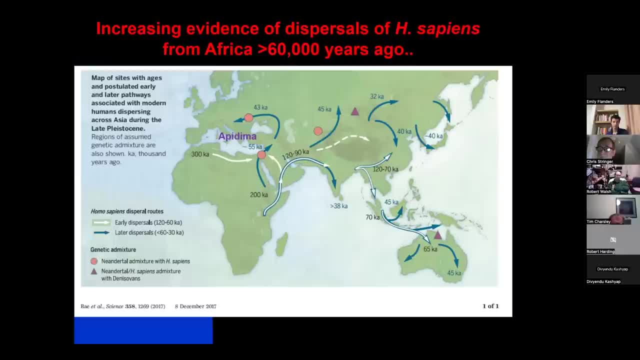 years ago from africa, but there are potentially earlier ones mapped in places like china and australia, and i've added in here um a fossil from epidema, which i was involved in studying with katarina havarti and colleagues, where we found what we think is the back of a homo sapiens. 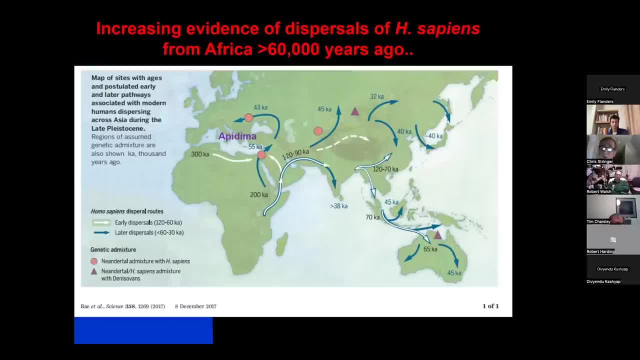 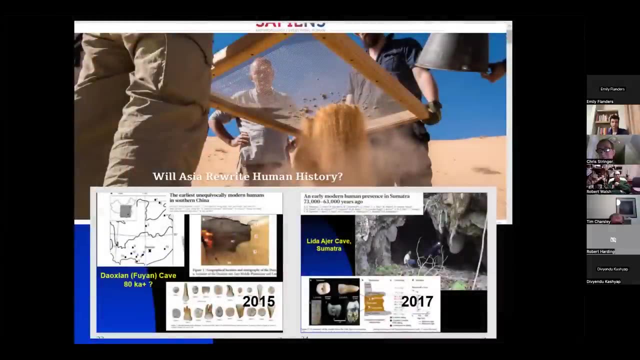 cranium from greece that dates to over 200 000 years ago. so that really would be a very early dispersal and very poorly known dispersed of homo sapiens much further back in time around over 200 000 years ago. so, yes, there's evidence. then, from places like china and sumatra we can see evidence. 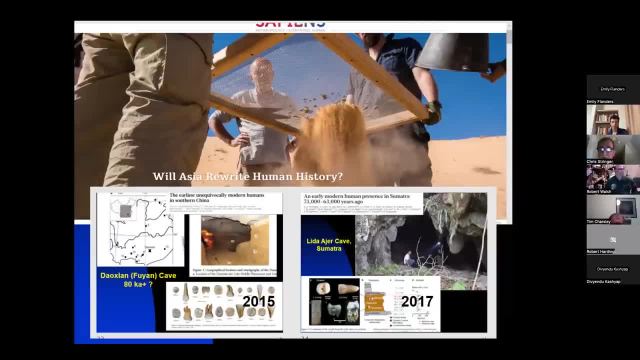 here from china at least 80 000 years old. we've got teeth from uh fuyang cave which certainly look like homo sapiens teeth and yet they're dated at least 80 000 years old from sumatra. i was involved in this publication uh with kira westaway and colleagues uh leader agio cave, where we've got. 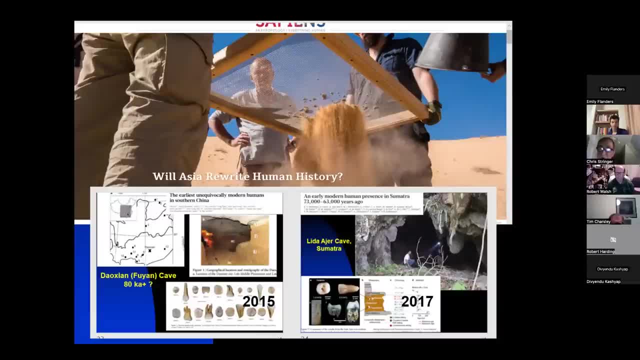 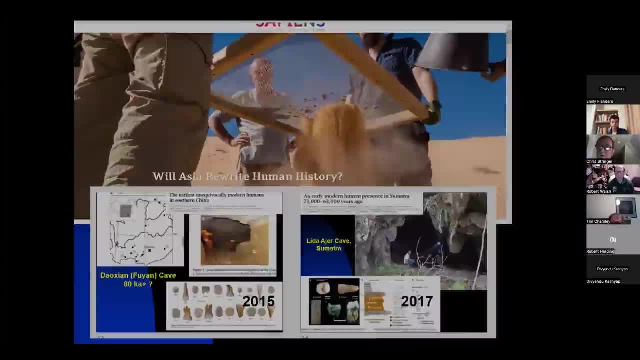 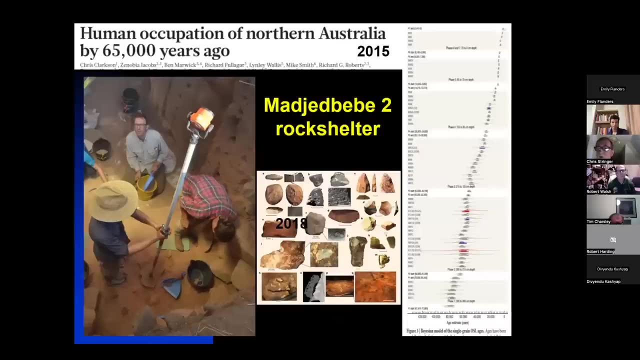 a couple of homo sapiens teeth which seem to be about 70 000 years old, so both of these over that 60 000 year threshold of a major, significant dispersal from africa and evidence from australia too of complex behavior in sediments at magia bebi ii rock shelter. 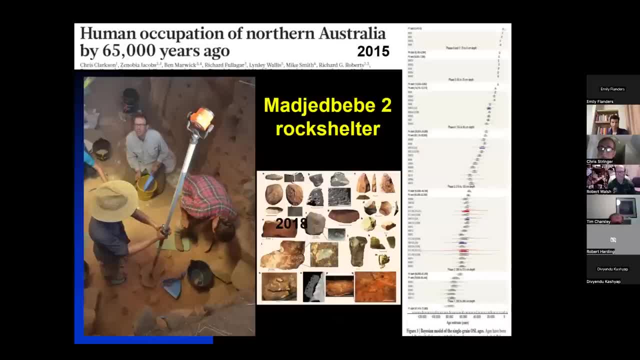 dated by a long sequence of luminescence dates. and this complex technology, complex use of pigments occurring around 65000 years ago, assumed to be the work of homo sapiens, and again beyond that sixty thousand threshold, uh placed on the main exit of homo sapiens from africa. 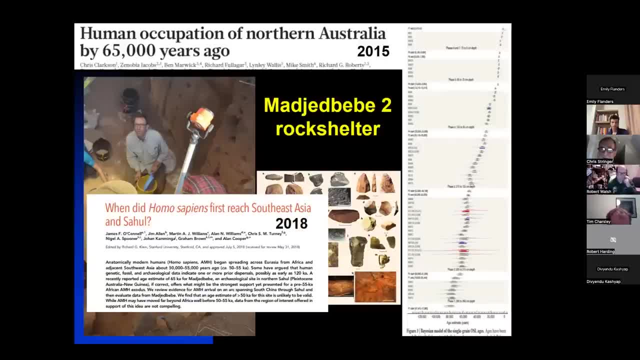 so how to explain it? well, some people don't believe it. they they argue that these dates are wrong and that the site actually dates from a maximum of about 40 000 years old, 5,000 years ago. so there are critics who don't accept this old dating, for Magibebe too, but you. 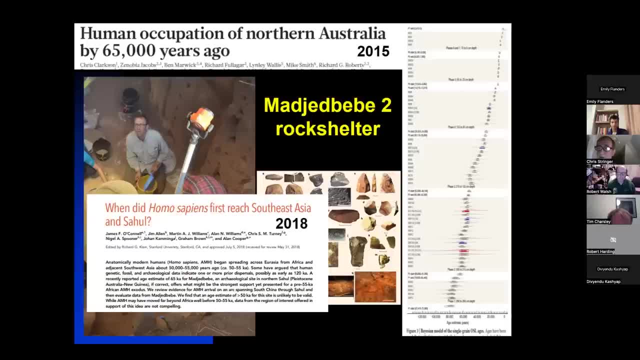 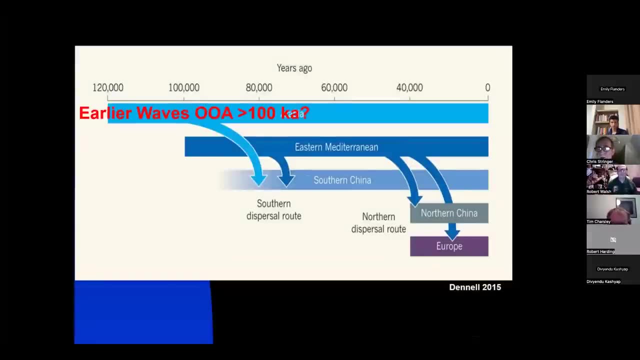 know it looks pretty sound to me and of course, if it is sound then more evidence will come forward from other sites which will demonstrate further evidence of a pre-60,000 year arrival of Homo sapiens in Australia. but if those early dispersals did happen- and this is a diagram from: 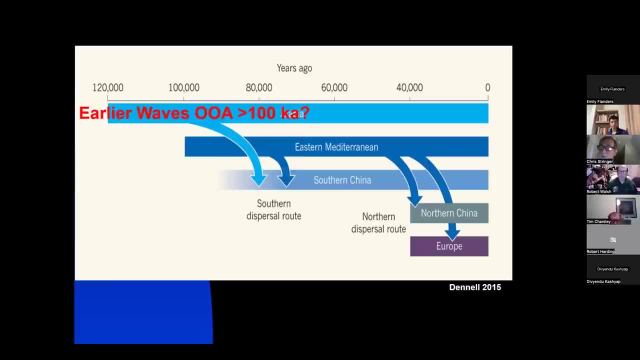 Robin Dennell from 2015. then, potentially, perhaps we did have these earlier waves of Homo sapiens out of Africa more than a hundred thousand years ago- perhaps several of them- and then we did have this major wave around 60,000 years ago, which the genetic data point to as the main dispersal. 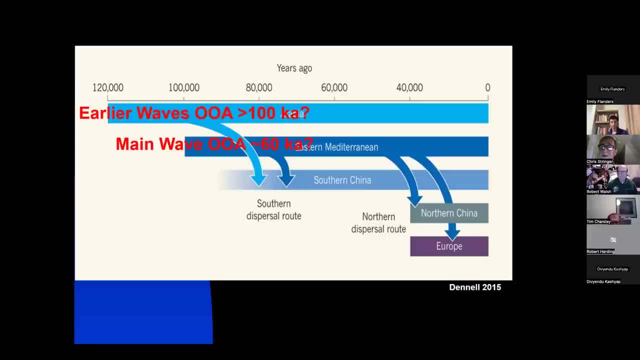 for the diversity, genetic diversity- of Homo sapiens out of outside of Africa today. but if that's correct, then either those earlier lineages disappeared or they were overprinted by this wave at 60,000 years that it actually swamped any genetic signature we can pick up. 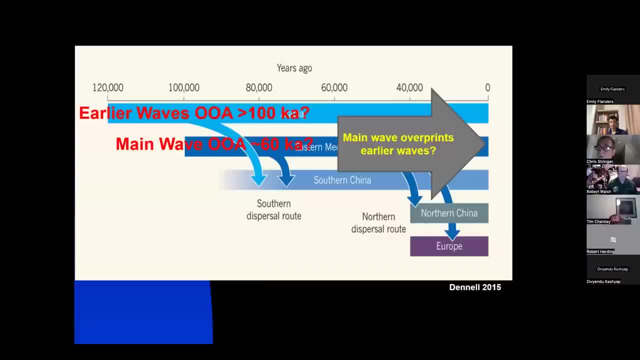 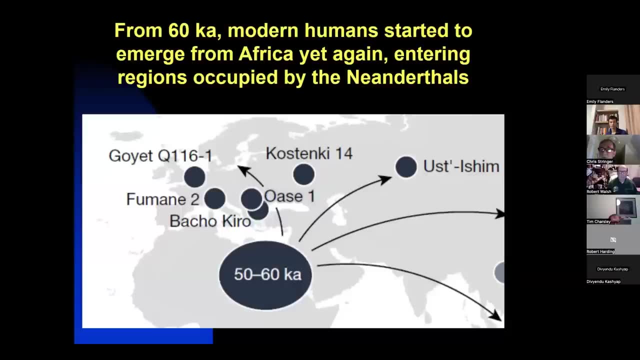 from those earlier Homo sapiens populations in regions like China and Australia, so on that 60,000 year dispersal or thereabouts. some modern humans emerged from Africa about 60,000 years ago and of course they were going to be entering regions occupied by the Neanderthals. 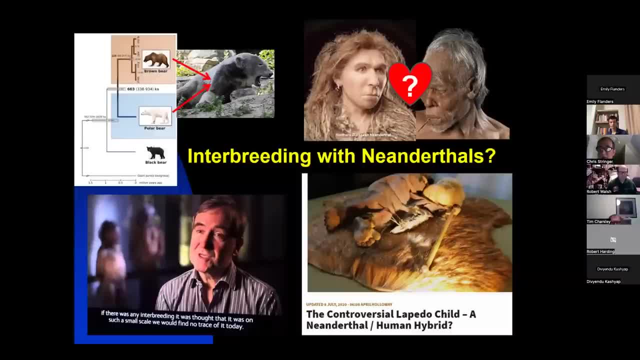 and that brings up, of course, that interesting question of interbreeding with the Neanderthal, something we've been arguing about for a long time. we've got that fossil down on the bottom right there from Portugal. a Lagavello or the Lepedo child argued to be a Neanderthal human hybrid. a lot of publicity on that 20 years ago. 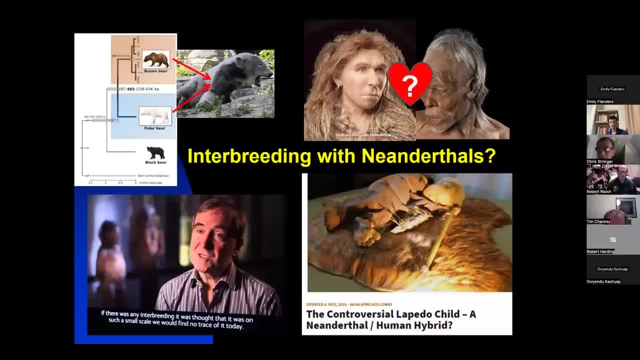 in fact the fossil morphologically to me doesn't look like any kind of hybrid. I see really no sign of Neanderthal morphology in that fossil and the skeleton is is Gravettian in age, so probably at most about 30,000 years old. so 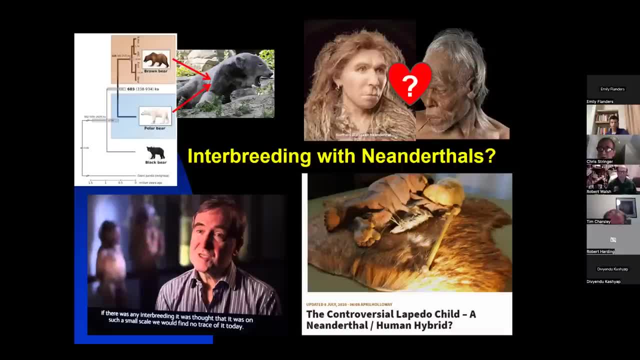 it's probably 10,000 years younger than any evidence of Neanderthals- convincing evidence of Neanderthals- in the region. so it's it's unlikely, both from chronology and morphology, to be any kind of a hybrid in my view, and my view for many years was that 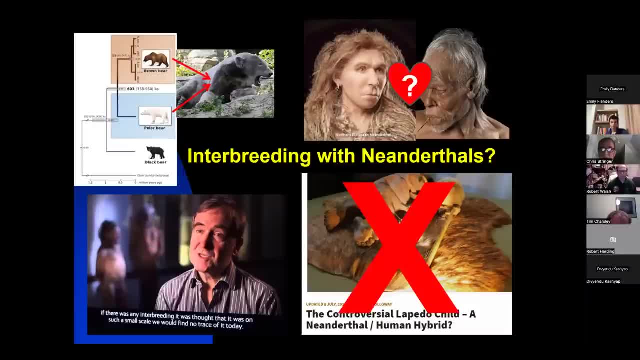 you know, given the evidence of brown bears and polar bears interbreeding- we've got that example up on the top left- that closely related mammal species can hybridize, as so I'm showing here, brown bear and polar bear with a similar divergence time of us and Neanderthals. 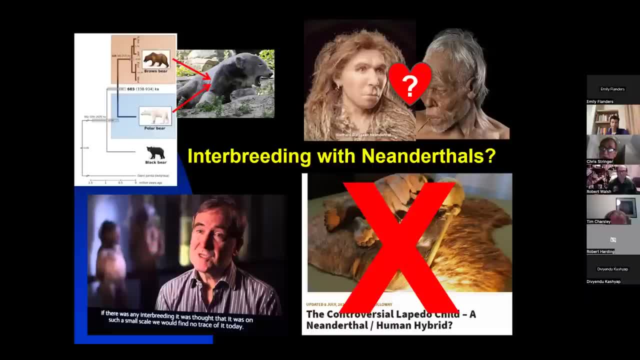 can produce fertile offspring. jackals and wolves can do that. species of baboons in Africa can do that. so I knew that could happen. so I thought that it could happen for us in Neanderthals. but my view up until 2010 was that if it happened, it wouldn't have been normal behavior, it'd be rare. these 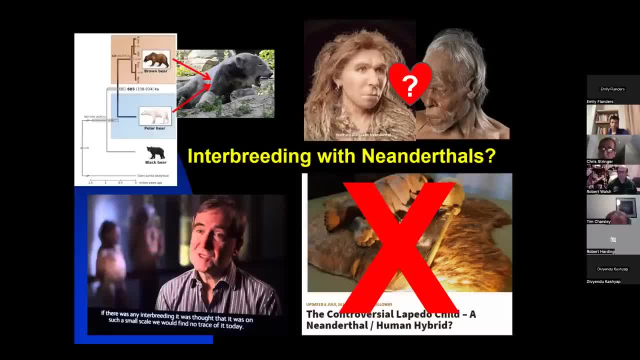 populations were quite small and it would have been very rare. and it would have been very rare and any small evidence of interbreeding from 40 or 50,000 years ago would have completely disappeared in the intervening time period. so maybe it happened 40 50,000 years ago, but in my view, 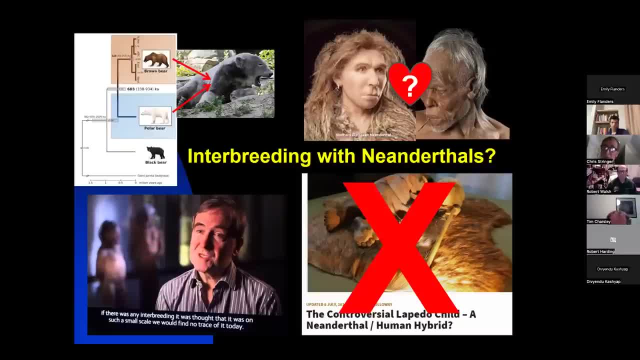 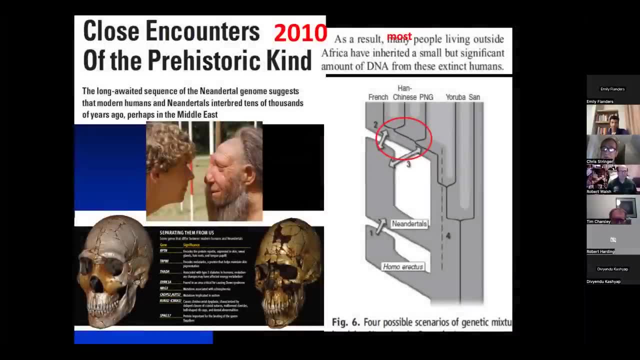 up to 2010, it will be trivial in the big picture of human evolution, but I was wrong about that, of course, because in 2010 we start to get the high quality Neanderthal genomes coming through and, as it says in this, this summary from science in 2010. 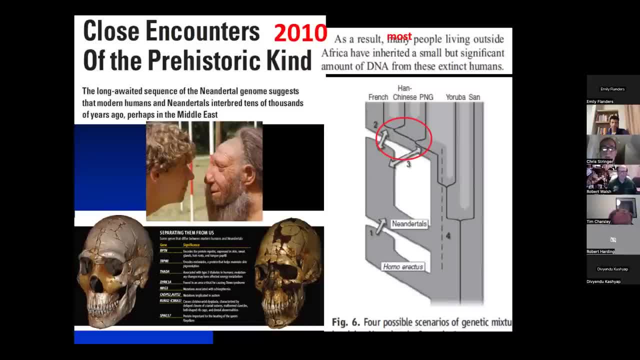 the long-awaited sequence of the Neanderthal genome suggests that modern humans and Neanderthals interbred tens of thousands of years ago, perhaps in the middle east. as a result- and I've corrected it to say most, not just many, but pretty well- everyone living outside of Africa has inherited. 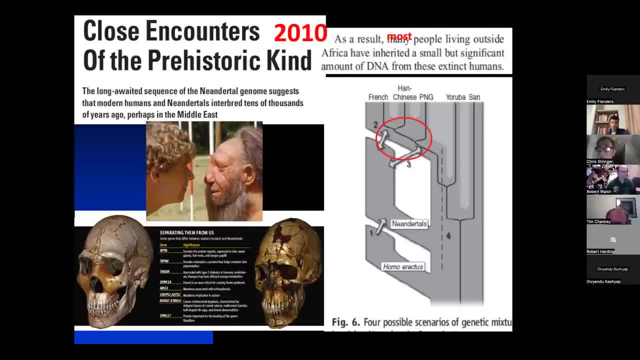 a small but significant amount of DNA from these extinct humans and, as it shows here on the diagram on the right, there we've got the view that, yes, there's a divergence of Neanderthals and the Homo sapiens lineage. and there's a divergence of Neanderthals and the Homo sapiens lineage and 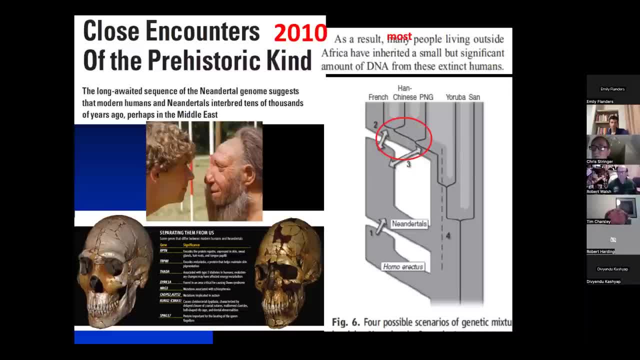 which stays in Africa, and then we come into the more recent past. we get the continuation of lineages in Africa, but a small group of humans get out into southwest Asia and there they meet Neanderthals. they interbreed with them, they pick up Neanderthal DNA and then it spreads with them. 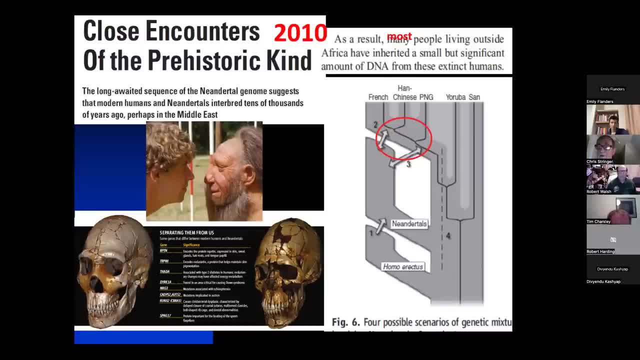 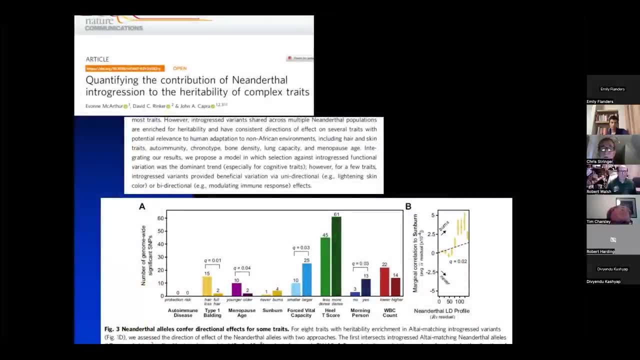 as they spread around the rest of the world outside of Africa, and, of course, a lot of work on what that DNA is doing. some of it certainly seems to be active in our, in our bodies today. here's just an example of one of these papers which talks about how 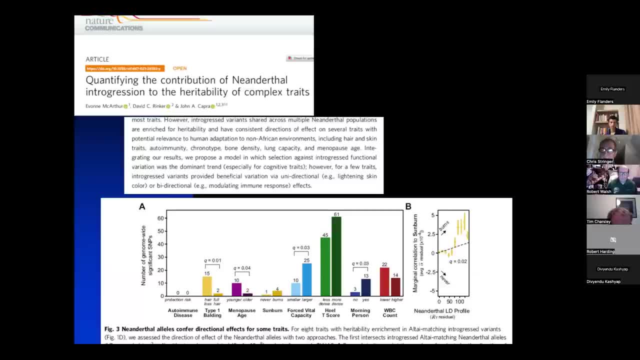 Neanderthal DNA is contributing to our phenotype today. so things like type 1 boarding, age of the menopause, susceptibility to sunburn, false vital capacity of the lungs, bone thickness, whether you're a morning or an evening person, your white blood cell count, so a number of things here which 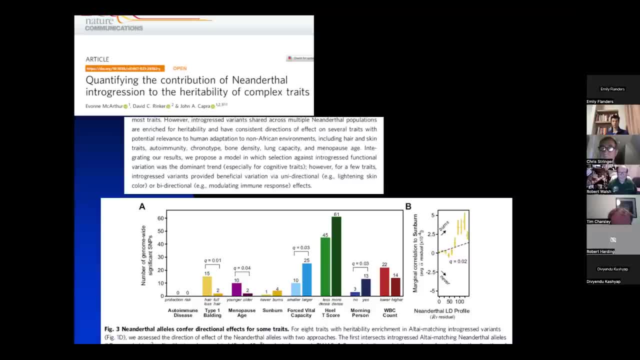 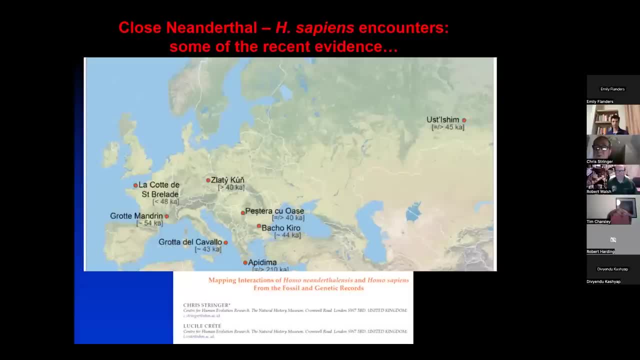 seem to be linked to the Neanderthal DNA and the Homo sapiens lineage, and the Homo sapiens lineage, which seems to be linked to the presence of Neanderthal DNA. so I recently wrote a review of some of this data from Europe about interactions of Homo. 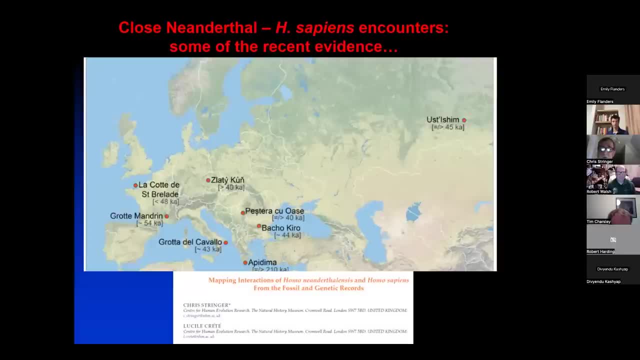 Neanderthalensis and Homo sapiens and wrote this with my colleague at the Natural History Museum, Lucille Crete, and have a look at it, because obviously some of what I say is covered in more detail in the paper and I'm just going to start talking now about Grotte Mondrian. you can see it. 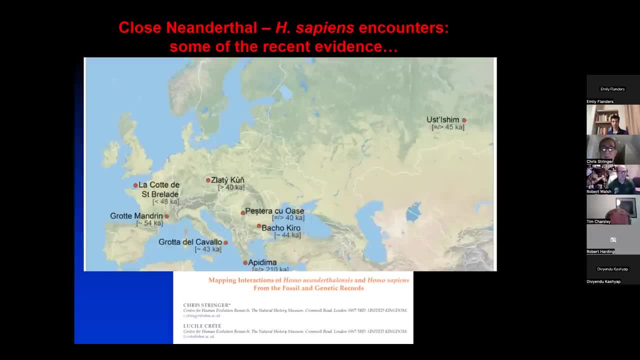 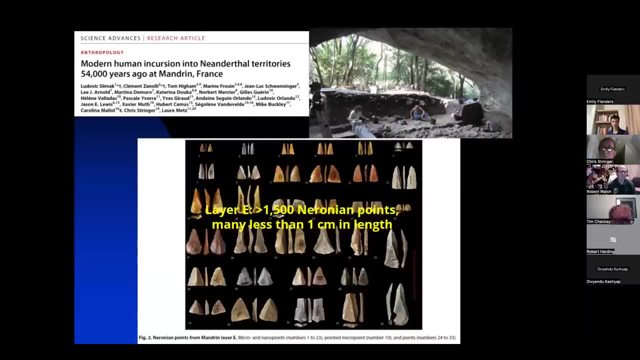 over on the left-hand side of this map here in the Rome Valley of France- and I'm just going to start talking now about Grotte Mondrian. you can see it over on the left-hand side of this map here in the Rome Valley of France. so I was involved in this publication … about a year ago- of this. 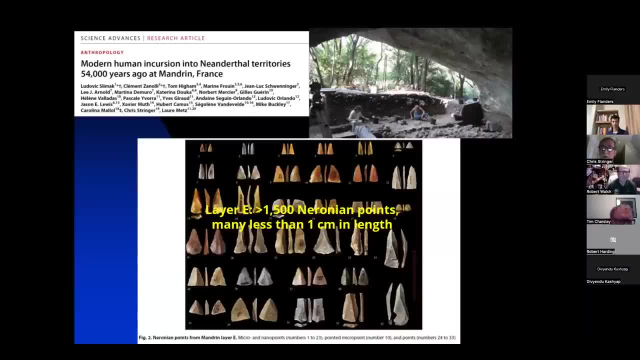 really intriguing evidence from Grotte Mondrian, where you've got this very distinctive archaeology in just one layer of the site, layer E, more than 1,500 of these tiny points called Neronian after archaeology from the nearby uh Neronian site …. and these are tiny points, many of them are less. 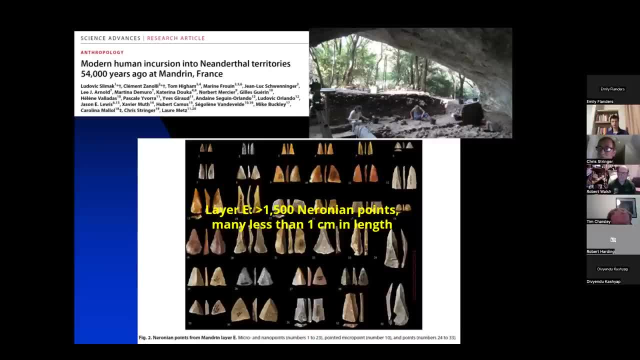 less than one centimeter in length and they look for all the world. like their arrowheads or dart heads, projectile small projectile points, and they're just present in one layer at the site. so this has been a puzzle for a long time, and ludovic slimac and his team have really worked. 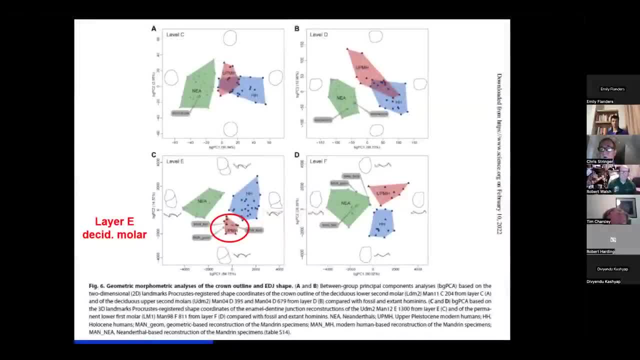 at this problem dated the layer to around 54 000 years old and there was one human tooth in that layer. the teeth in the other layers were all identified as neanderthal, but the teeth in layer e- the tooth in layer e, a deciduous, molar child's tooth- seems to fall into homo sapiens. so we seem. 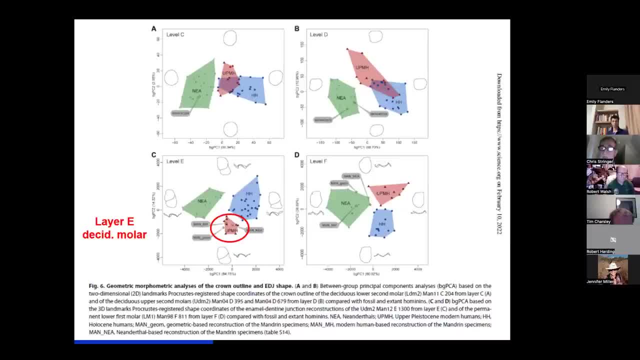 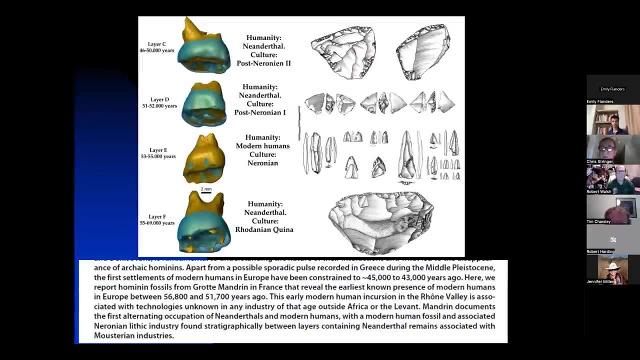 to have a homo sapiens morphology associated with this very distinctive neuronian archaeology at about 54 000 years ago. so here's a diagram summarizing that pattern. so in the lower levels we've got neanderthal teeth associated with neanderthal stone tools. we've got the neuronian level estimated to be a very 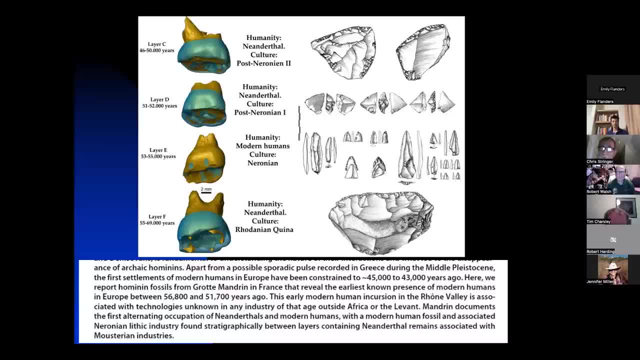 short duration. from studying the soot deposits of repeated fires in the cave, ludovic and colleagues estimated the duration of the occupation by this neuronian people could be even less than 100 years. then we have a sterile layer and the people who come back are neanderthals again making. 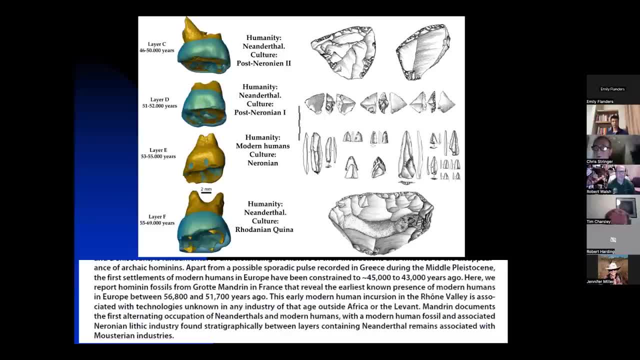 neanderthal stone tools and then finally the neanderthal stone tools and then finally, at the very top later on in the sequence, we actually get the arrival of homo sapiens and the oregnacian. so, as it says, here we report fossils from grot mondrand that show the early 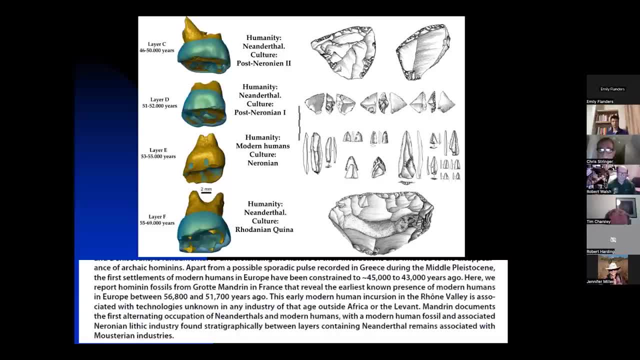 presence of modern humans in europe between about 57 000 and 52 000 years ago. this early modern human incursion in the rome valley is associated with technologies unknown in any industry of that age outside of africa or the levant. mondrand documents the first alternate gene of human. 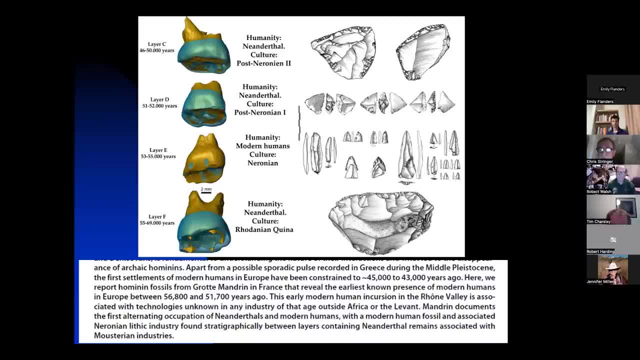 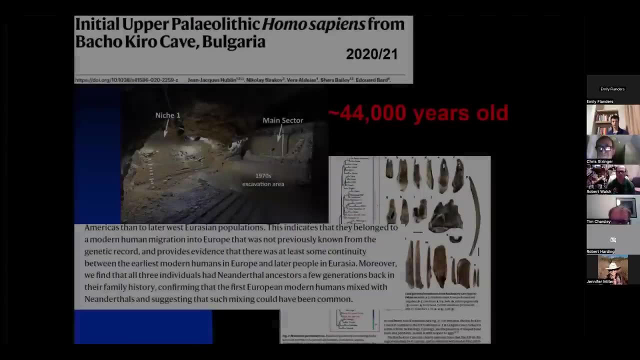 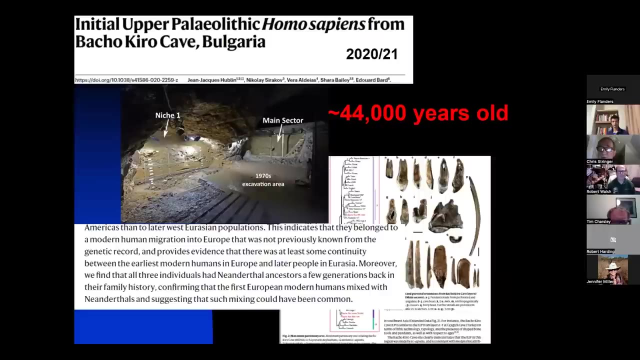 a fascinating occupation of Neanderthals and modern humans, with a modern human fossil and associated Neronian lithic industry found stratigraphically between layers containing Neanderthal remains associated with Mysterian industries. So really quite a surprising find. And later on in time, about 10,000 years later, we have more evidence of Homo sapiens from Bacchicuro, a site that's been known for many years but recently excavated by Hubelan and colleagues with wonderful results both in archaeology and in terms of fossil discoveries. 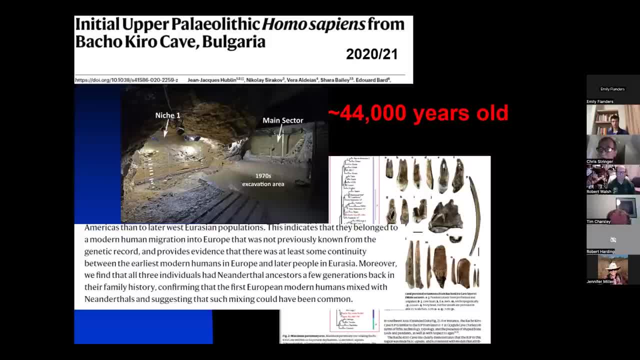 So a number of fragmentary human fossils. they can be identified as Homo sapiens from morphology or from their DNA And, as it says here, This indicates that they belong to a modern human migration to Europe That was not previously known from the genetic record and provides evidence that there was at least some continuity between the earliest modern humans in Europe and later people in Eurasia. 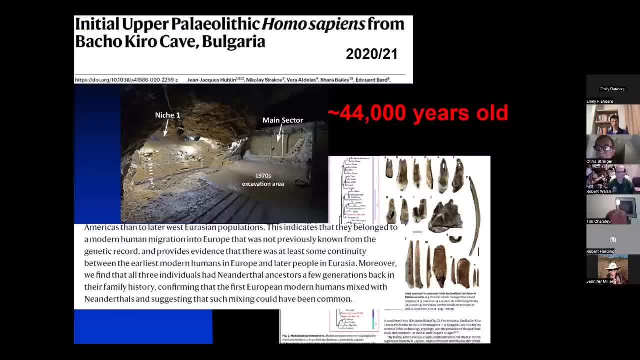 Moreover, we find that all three individuals had Neanderthal ancestors a few generations back in their family history, confirming that the first European modern humans mixed with Neanderthals and suggesting that such mixing could have been common, And subsequent papers actually also showed something very interesting. 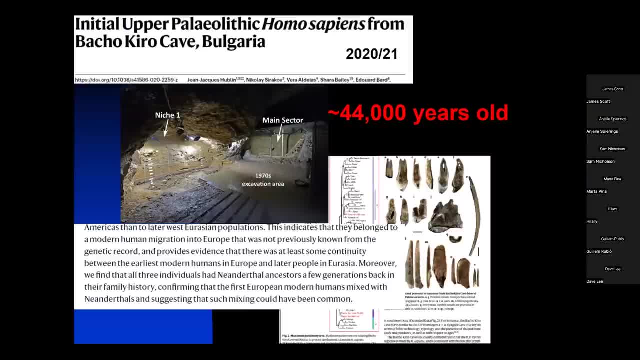 And I think it's interesting about the Bacchicuro evidence from about 44,000 years ago. So many of us have worked on the assumption that Homo sapiens came into Europe during climatic ameliorations, when the climate temporarily warmed up. that gave an opportunity for Homo sapiens to move out of regions like Western Asia and into Europe. 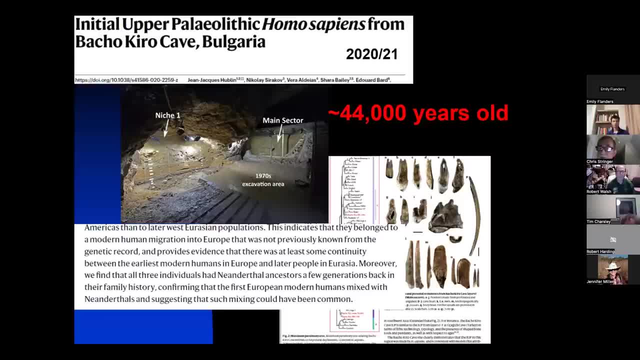 But in fact the evidence shows that these Bacchicuro early Homo sapiens were actually living in cold conditions alongside cold climate animals. But in fact the evidence shows that these Bacchicuro early Homo sapiens were actually living in cold conditions alongside cold climate animals. 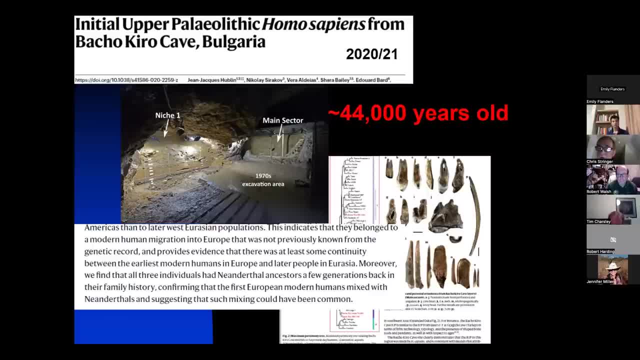 And they were coping with that. And of course we've got a question: whether is this a sign of their rapid adaptation to cold conditions, or could it even be that this mixing with Neanderthals provided some cultural background for them to adapt to the local conditions in Europe at the time? 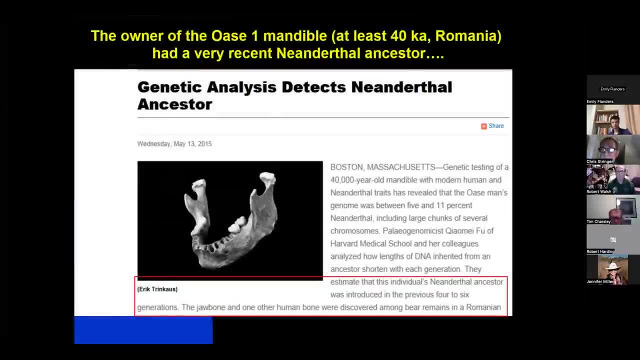 And then been known for a lot longer. this Oasi jawbone, a robust jawbone, got a nice chin on the front, so it looks like a Homo sapiens, But rather large and complex teeth, and suspicions that it might be some kind of a hybrid in this case were demonstrated from its DNA, because it has the largest amount of Neanderthal DNA known in any Homo sapiens fossil. 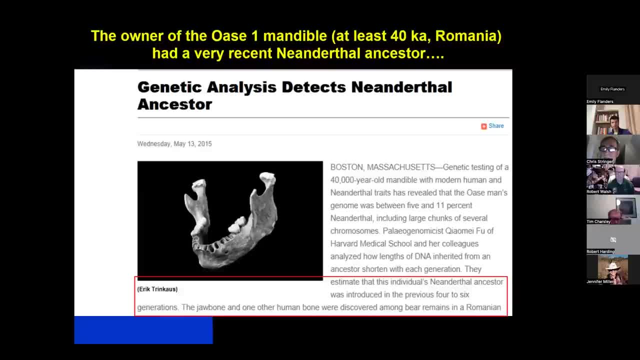 And, as it says here, they estimate that this individual's Neanderthal ancestor was introduced in the previous four to six generations. So this is a fossil that's at least 40,000 years old and has a very recent Neanderthal ancestor. 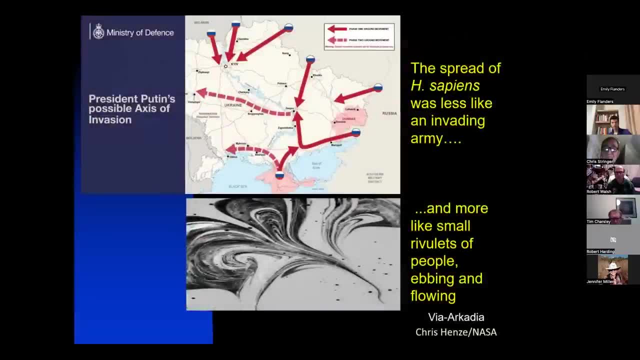 In its pedigree. So how did we look at this, you know, in arrival of Homo sapiens into Europe? Well, I don't think it's anything like this, this proposed model of Putin's invasion of Ukraine, which certainly didn't work out for Putin either, quite as was expected here in this map. 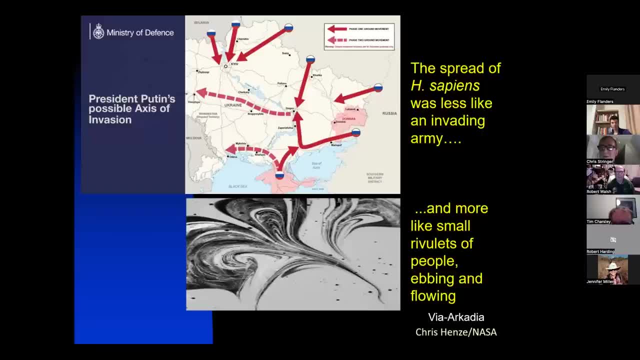 And I think it's much less. the arrival of Homo sapiens is much less like an invading army and much more like small rivulets of people ebbing and flowing, And the Neanderthal population also ebbing and flowing in a similar way. 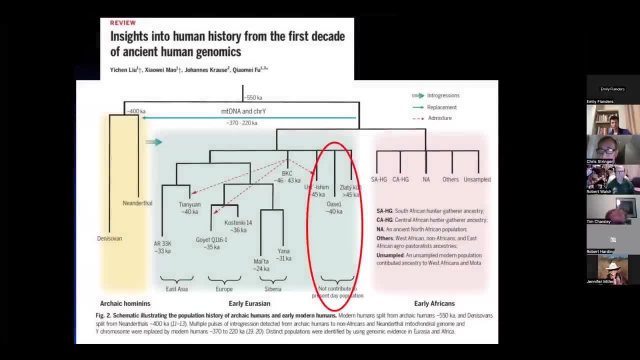 And what's interesting from the genetic data- and hinted at along the way already, is that on this summary from Liu and colleagues of the genetic data, It's a very nice summary paper. We've got on the left hand side there the Neanderthal and Denisovan lineages in yellow. 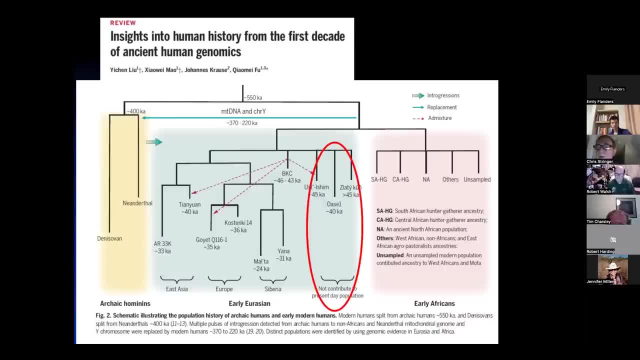 We've got the African lineages over there on the right hand side in the sort of pink color And the Neanderthal and Denisovan lineages in yellow. We've got the African lineages over there on the right hand side in the sort of pink color. 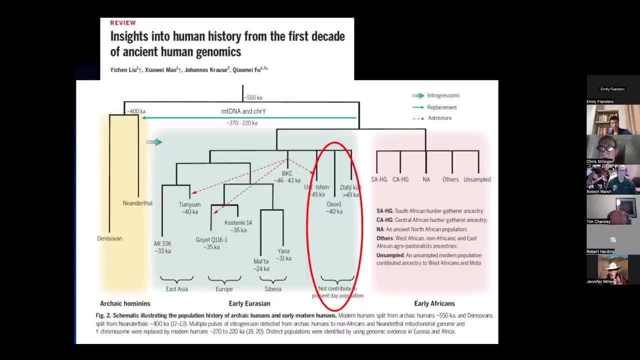 And then the Eurasian lineages of early Homo sapiens in green in the center of the diagram, And then the Eurasian lineages of early Homo sapiens in green in the center of the diagram. And you can see as I've circled there in this red ellipse, that some of these lineages- and that includes the Oasi individual, the leg bone from Ustikshim in Siberia, the Zlatikun skeleton from Chechya, their DNA does not seem to pass through to present day populations. 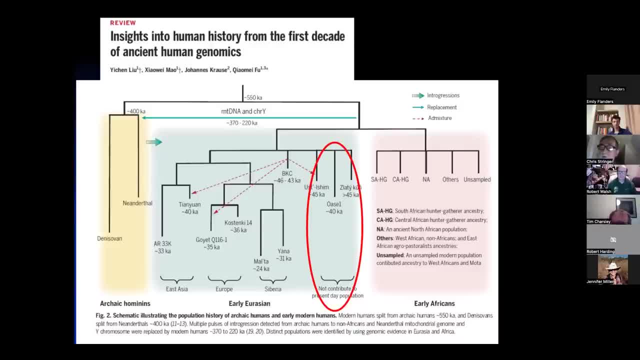 The Zlatikun skeleton from Chechya. their DNA does not seem to pass through to present day populations, So some of these could be said to be lost lineages of Homo sapiens. So some of these could be said to be lost lineages of Homo sapiens. 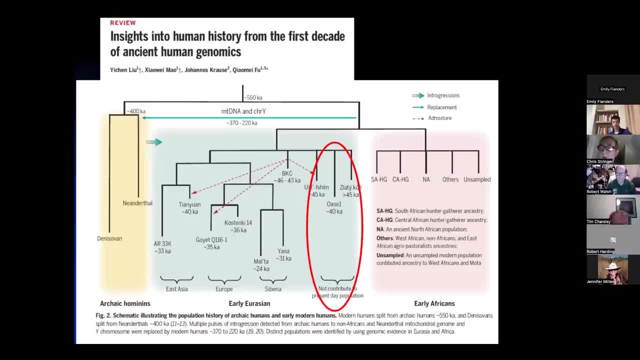 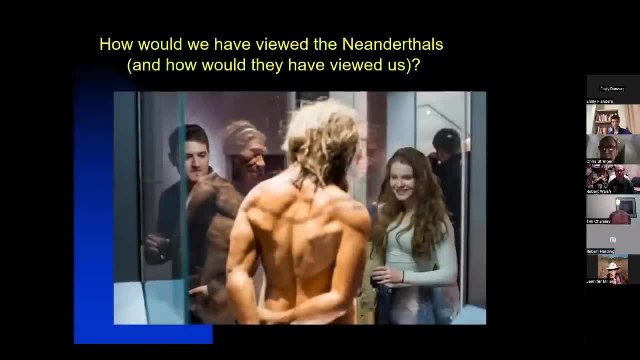 So not all of these populations carried on. They didn't have genetic continuity through to the present day. So how would we have viewed the Neanderthals when we, when we encountered them in Europe and Asia? So this is from our human evolution exhibit in London. 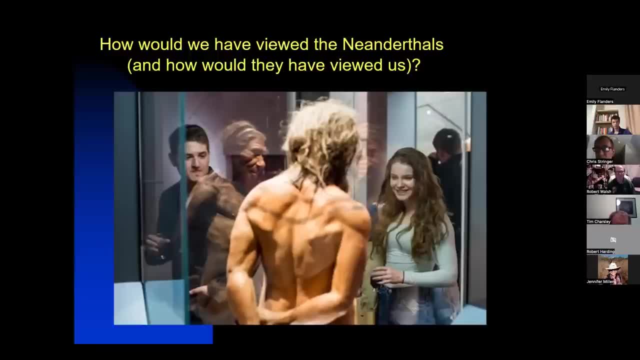 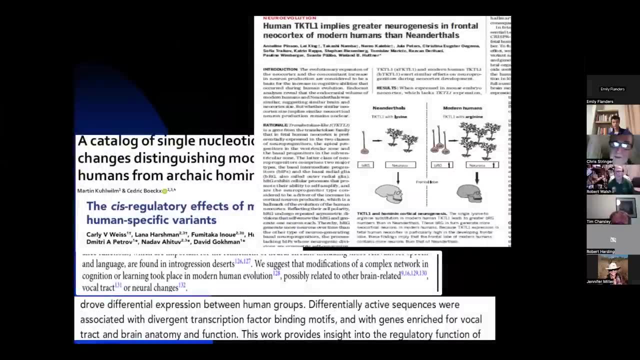 So this is a question which, of course, you know, we have no firm evidence on this at all. So this is a question which, of course you know, we have no firm evidence on this at all. there is some genetic data that suggests that there could have been, you know, significant. 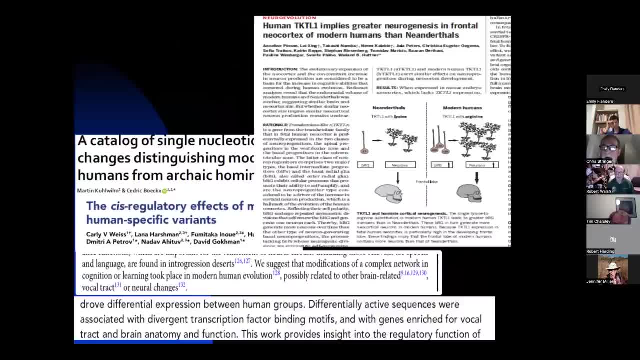 differences between us and Neanderthals in cognition and in, for example, the morphology of the vocal tract. so a couple of papers on the left hand side here and just summarizing the conclusion here, we suggest that modifications of a complex network in cognition or learning took place in modern human evolution, possibly related to other brain related vocal tract or 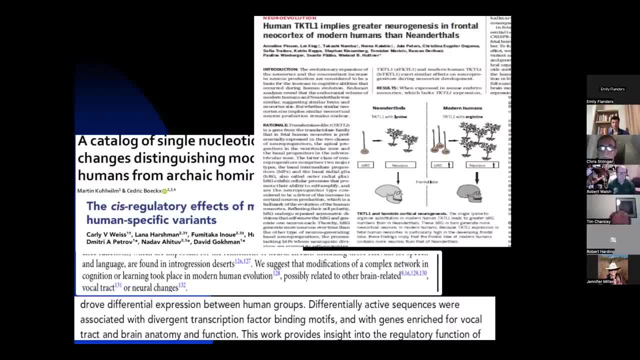 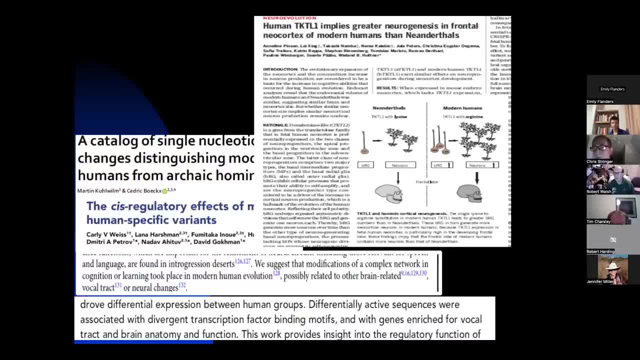 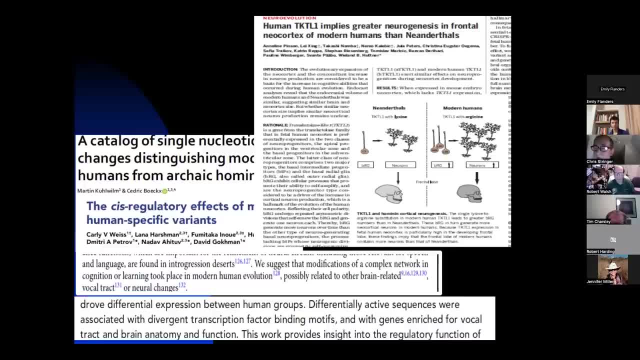 mutation in one gene which, when it's transferred into fetuses of other mammals, it produces a much greater initial diversity of neurons in the frontal cortex of the brain, in the frontal cortex of the brain, in the frontal cortex of the brain, compared with the neanderthal version of. 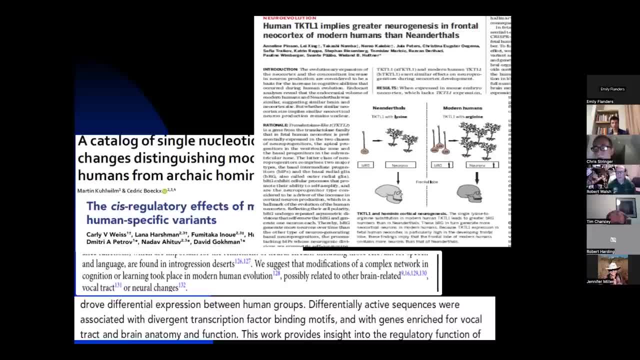 compared with the neanderthal version of, compared with the neanderthal version of the gene, so evidence that perhaps the gene so evidence, that perhaps the gene so evidence that perhaps modern infants had a much greater neuron. modern infants had a much greater neuron. modern infants had a much greater neuron density. 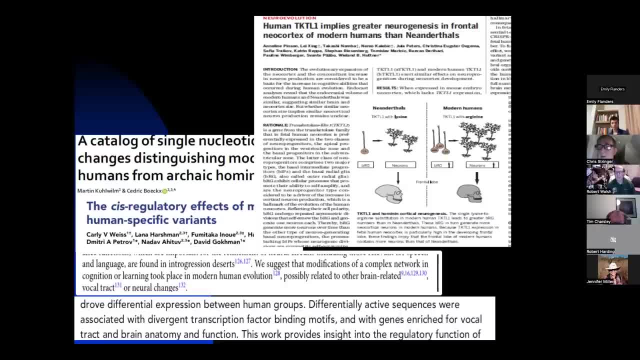 density, density, the ones who had this particular variant, the ones who had this particular variant, the ones who had this particular variant of this homo sapiens gene, different from of this homo sapiens gene, different from of this homo sapiens gene, different from the one known in neanderthals, and. 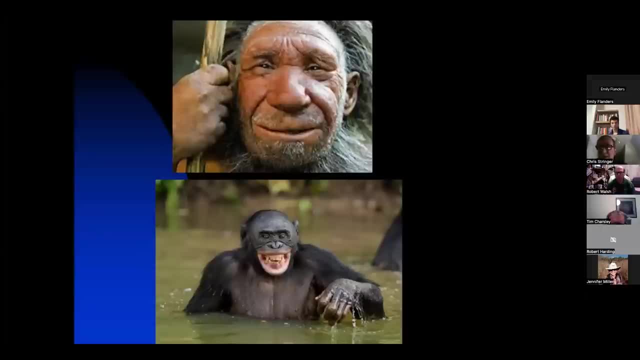 the one known in neanderthals and the one known in neanderthals and denisovans. so how would we have viewed the? so how would we have viewed the? so how would we have viewed the neanderthals when we met them? well, 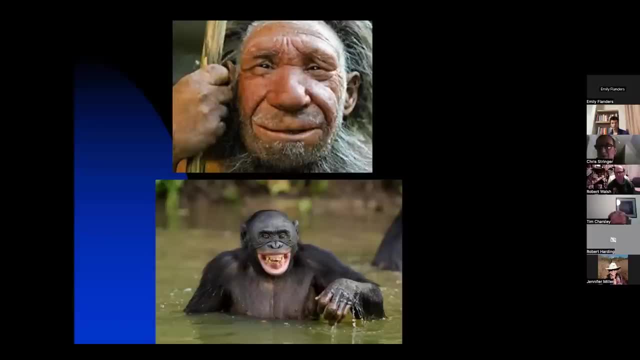 neanderthals when we met them well. neanderthals when we met them well. there's a bonobo at the bottom there. a, there's a bonobo at the bottom there. a, there's a bonobo at the bottom there, a reconstruction by the kenneth brothers. reconstruction by the kenneth brothers, reconstruction by the kenneth brothers of a neanderthal at the top, and we've got of a neanderthal at the top and we've got of a neanderthal at the top and we've got to remember the neanderthals are. 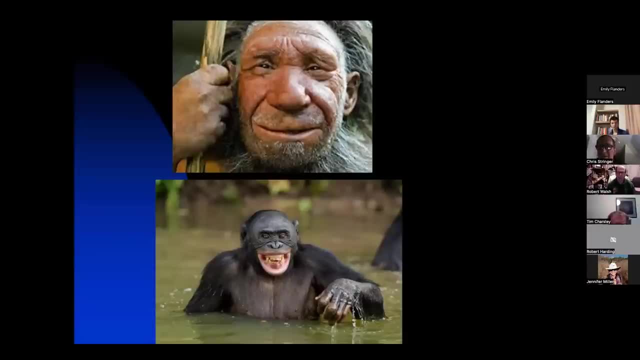 to remember the neanderthals are to remember. the neanderthals are certainly 10 times closer to us in time, certainly 10 times closer to us in time, certainly 10 times closer to us in time, and in genetics and in evolution than and in genetics and in evolution than. 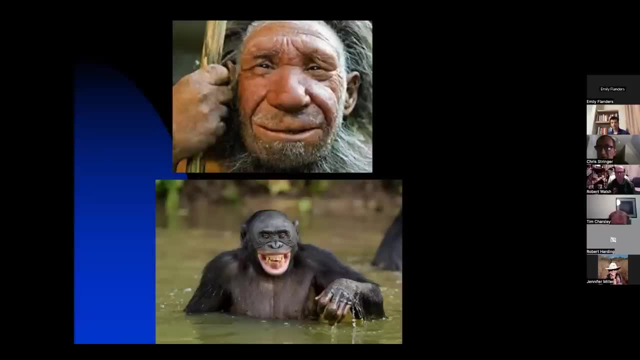 and in genetics and in evolution than the chimpanzees. so they are very human, the chimpanzees, so they are very human. the chimpanzees, so they are very human. they are very close to us in evolutionary. they are very close to us in evolutionary. they are very close to us in evolutionary terms. 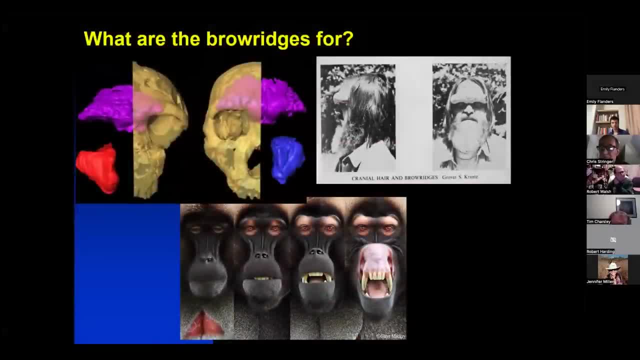 terms, terms, but there are differences and we mentioned. but there are differences and we mentioned, but there are differences and we mentioned some of them morphologically and there's some of them morphologically and there's some of them morphologically. and there's that brow ridge over the eyes. it's a. 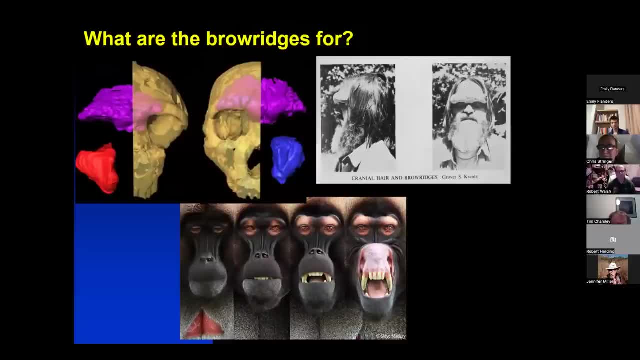 that brow ridge over the eyes. it's a that brow ridge over the eyes. it's a fascinating structure. fascinating structure. fascinating structure. um so, um so, um so. grover kranz because we're about 50 years. grover kranz because we're about 50 years. 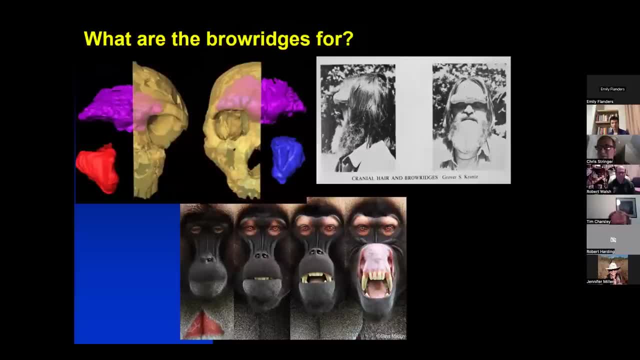 grover kranz, because we're about 50 years on from grover's famous experiment, on from grover's famous experiment, on from grover's famous experiment where he modified a, where he modified a, where he modified a homo erectus brow ridge and he wore it. 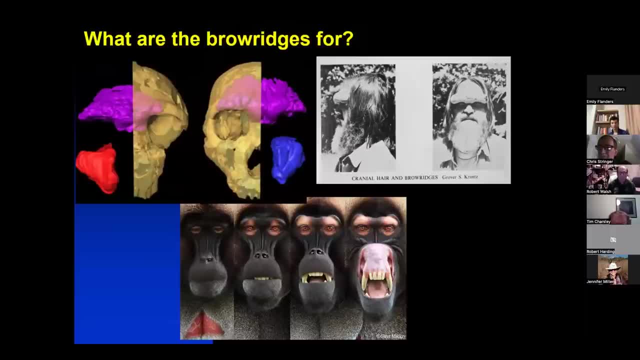 homo erectus brow ridge, and he wore it, homo erectus brow ridge, and he wore it on his head for six months to see what on his head for six months, to see what on his head for six months, to see what it would do for him. it would do for him. 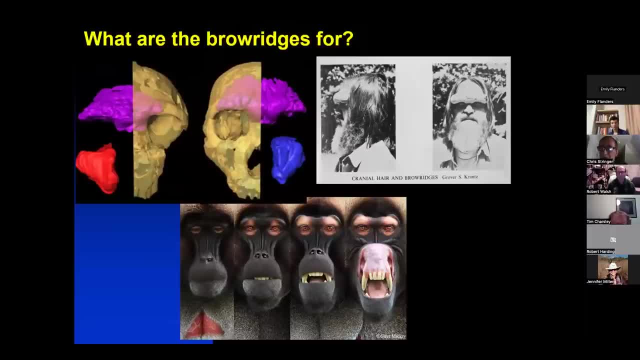 it would do for him. because he was puzzled about its function, because he was puzzled about its function. because he was puzzled about its function, he found it made a nice sunshade, as you, he found it made a nice sunshade. as you, he found it made a nice sunshade, as you can see there on a sunny day. 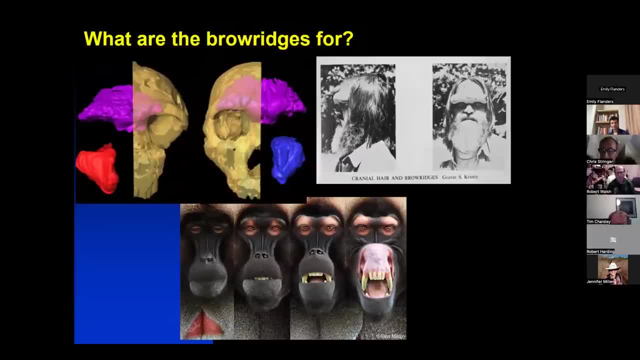 can see there on a sunny day. can see there on a sunny day. um, he found that when he ran along it, um, he found that when he ran along it, um, he found that when he ran along it, kept his hair neatly away from his eyes, kept his hair neatly away from his eyes. 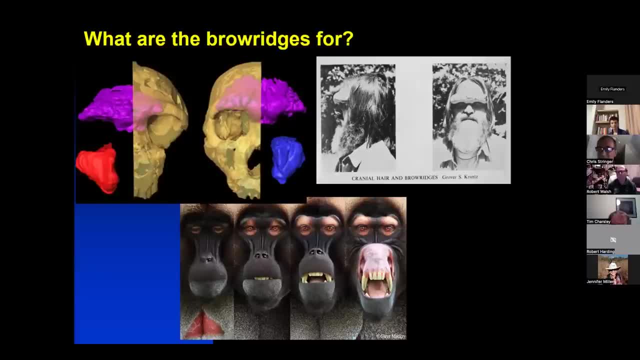 kept his hair neatly away from his eyes so he could see where he was going. so he could see where he was going. so he could see where he was going. um, i think that's probably uh, not the um. i think that's probably, uh, not the um. i think that's probably uh, not the best explanation, because you know these. 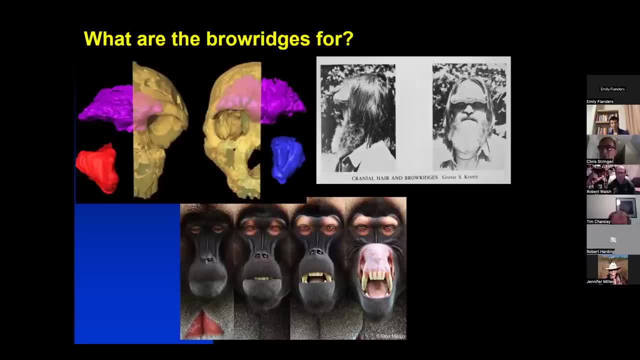 best explanation because you know these best explanation because you know these, these ancient humans were perfectly. these ancient humans were perfectly. these ancient humans were perfectly capable of butchering animal carcasses, capable of butchering animal carcasses, capable of butchering animal carcasses with sharp flints. and you'd have thought, with sharp flints and you'd have thought: with sharp flints, and you'd have thought they could have worked out to cut their. they could have worked out to cut their. they could have worked out to cut their hair if it was falling in front of their. 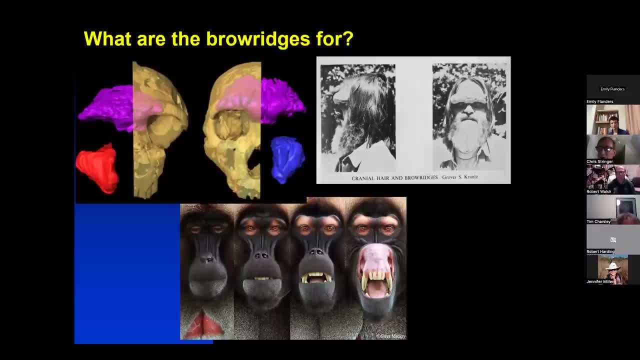 hair, if it was falling in front of their hair, if it was falling in front of their eyes, but what he also found was that on eyes. but what he also found was that on eyes. but what he also found was that on a dark night, coming around a corner. 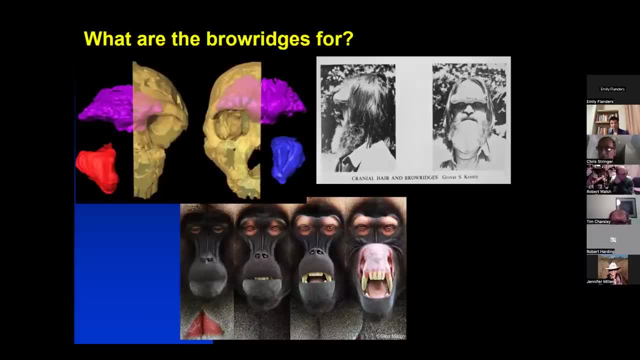 a dark night coming around a corner, a dark night coming around a corner, people were frightened almost to death. people were frightened almost to death. people were frightened almost to death when they suddenly met grover coming. when they suddenly met grover coming. when they suddenly met grover coming around with these great big brow. 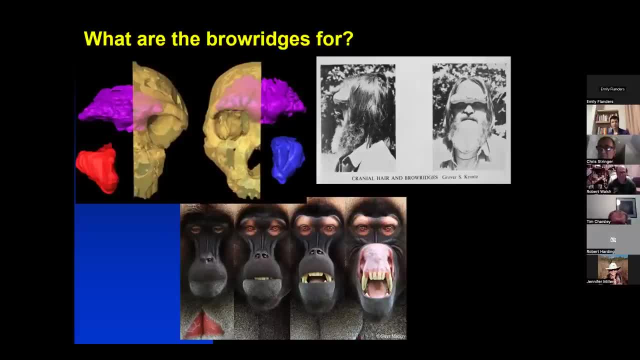 around with these great big brow, around with these great big brow ridges. so he also argued that it could ridges. so he also argued that it could ridges. so he also argued that it could have had a signaling function, have had a signaling function, have had a signaling function. um, and i think that's certainly a. 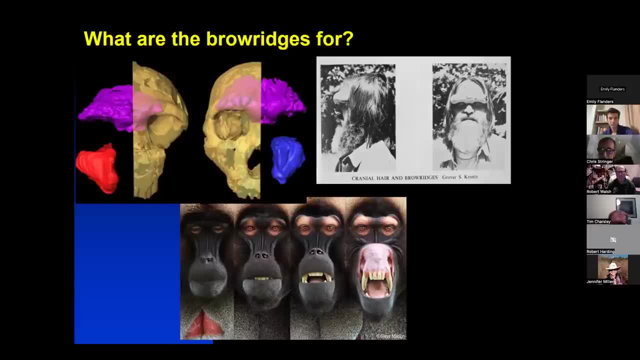 um, and i think that's certainly a um, and i think that's certainly a possibility- that this possibility, that this possibility that this, this brow ridge, could have accepted, this brow ridge could have accepted this brow ridge could have accepted accentuated signals from the eyes. accentuated signals from the eyes. 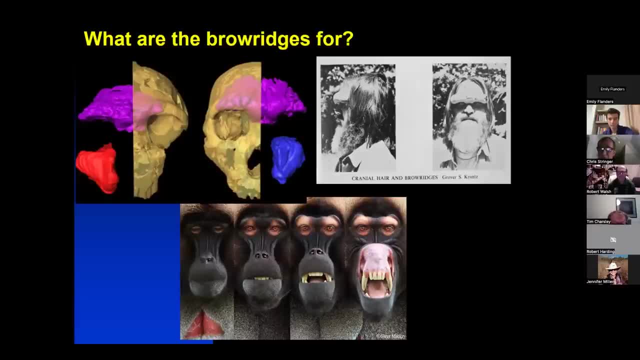 accentuated signals from the eyes of friendly or aggressive stares, of friendly or aggressive stares, of friendly or aggressive stares, and we see something like that even in, and we see something like that even in, and we see something like that even in baboons. so we've got an example of a 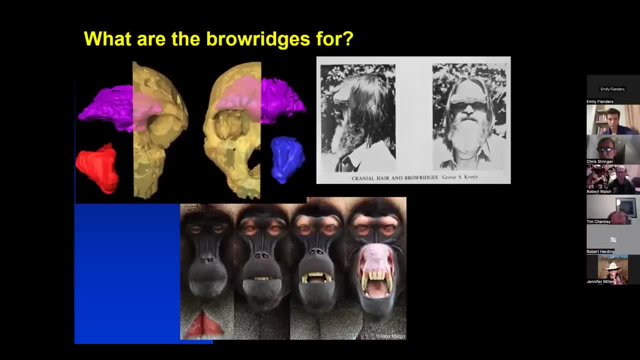 baboons. so we've got an example of a baboons. so we've got an example of a baboon, baboon, baboon in a threat gesture at the bottom there, in a threat gesture at the bottom there, in a threat gesture at the bottom there, and of course, baboons have got these huge. 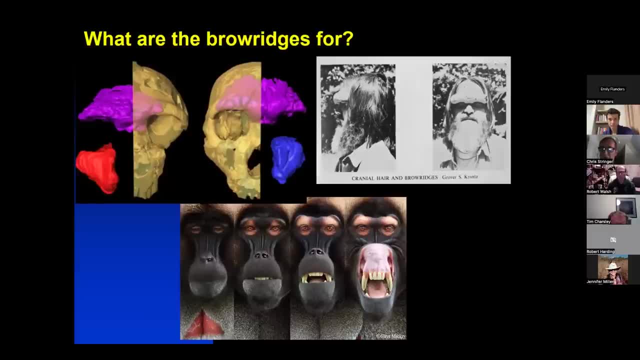 and of course baboons have got these huge and of course baboons have got these huge canines which they bear, canines which they bear, canines which they bear as part of their threat gesture, but also as part of their threat gesture, but also as part of their threat gesture. but also notice the way that the eyes 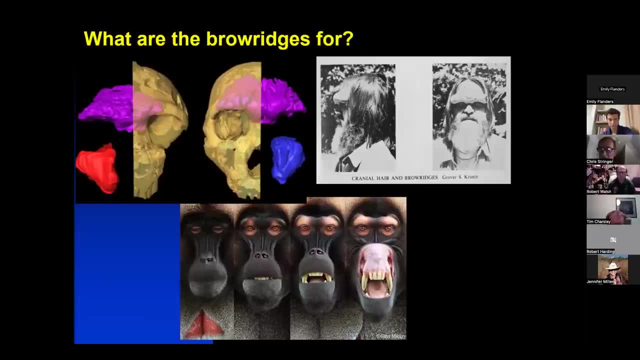 notice the way that the eyes notice, the way that the eyes highlight. they sort of light up to highlight, they sort of light up to highlight, they sort of light up to accentuate, accentuate, accentuate that aggressive stare. so perhaps there, that aggressive stare, so perhaps there. 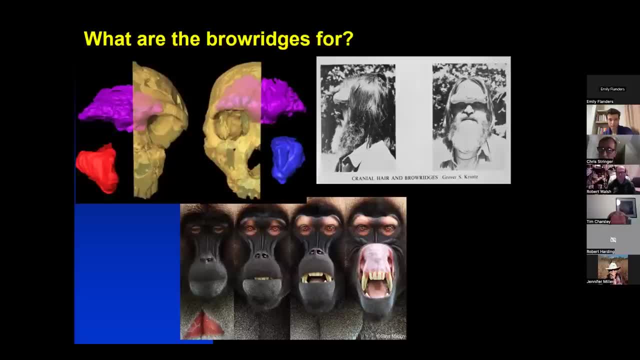 that aggressive stare. so perhaps there is a social function for these brow is a social function for these brow is a social function for these brow ridges which continued in the neanderthals ridges, which continued in the neanderthals ridges which continued in the neanderthals and which we have lost. 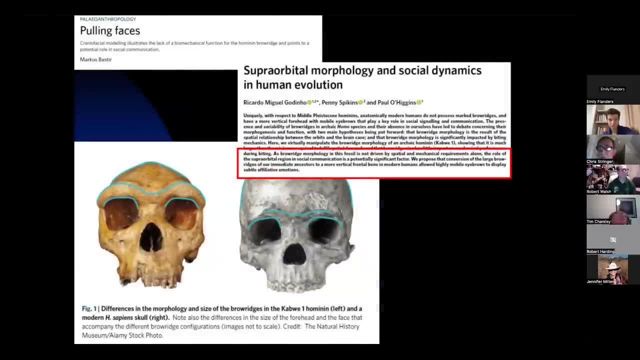 and which we have lost and which we have lost and that's something which uh gradino and and that's something which uh gradino and and that's something which uh gradino and colleagues uh suggested, and this is a colleagues uh suggested and this is a. 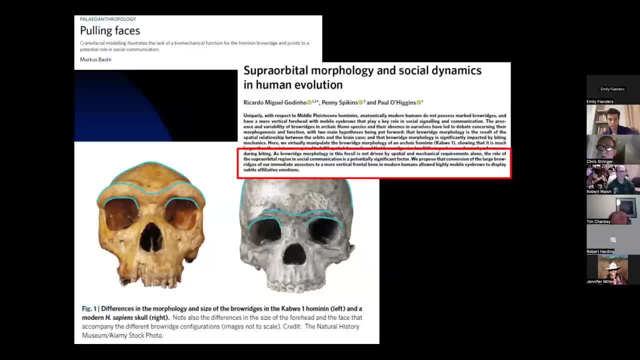 colleagues uh suggested, and this is a paper about super orbital morphology and paper about super orbital morphology and paper about super orbital morphology and social dynamics in human evolution and social dynamics in human evolution and social dynamics in human evolution and, as they say here, as brow ridge, as they say here, as brow ridge. 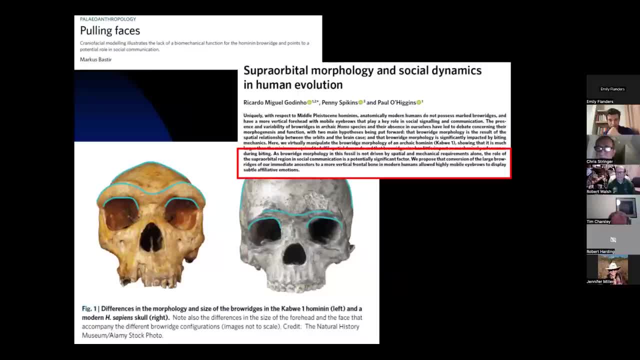 as they say here, as brow ridge- morphology in this fossil. we're talking morphology in this fossil. we're talking morphology in this fossil. we're talking about broken hill here cabway. about broken hill here cabway. about broken hill here cabway is not driven by spatial and mechanical. 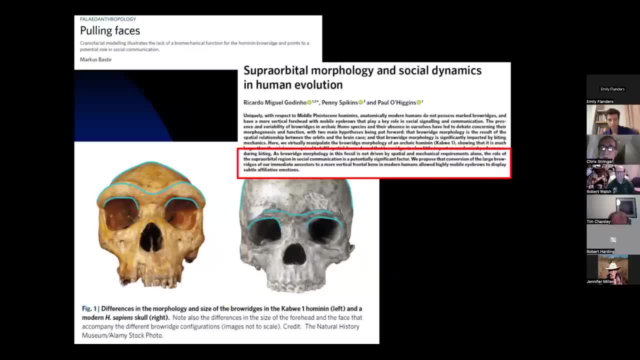 is not driven by spatial and mechanical, is not driven by spatial and mechanical requirements alone. the role of the requirements alone, the role of the requirements alone, the role of the super orbital region in social super orbital region, in social super orbital region, in social communication, is a potentially 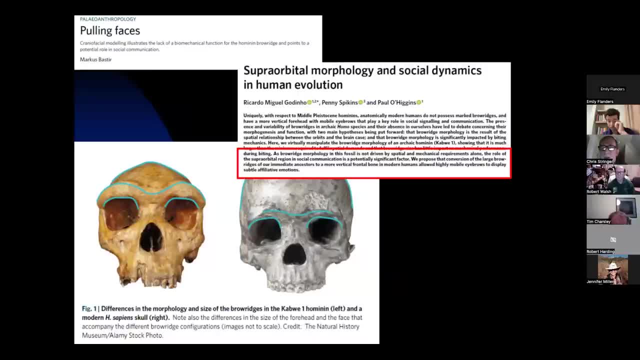 communication is a potentially communication is a potentially significant factor, significant factor, significant factor. we propose that conversion of the large. we propose that conversion of the large. we propose that conversion of the large brow ridges of our immediate ancestors, brow ridges of our immediate ancestors, brow ridges of our immediate ancestors- to a more vertical frontal bone in. 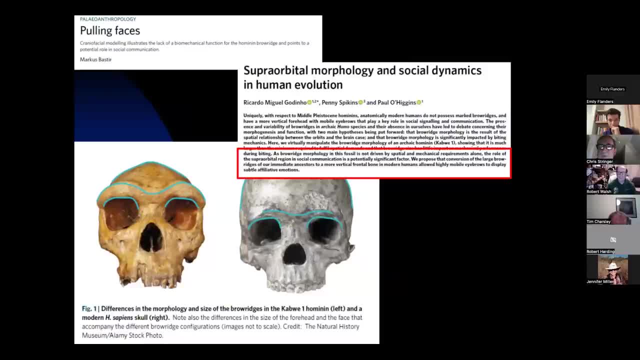 to a more vertical frontal bone, in to a more vertical frontal bone in modern humans. allowed highly mobile modern humans. allowed highly mobile modern humans. allowed highly mobile eyebrows to display subtle affiliative eyebrows. to display subtle affiliative eyebrows. to display subtle affiliative emotions, emotions, emotions. and marcus bastier in his commentary. 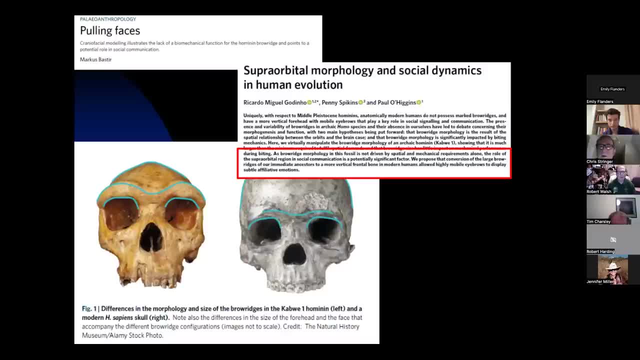 and marcus bastier in his commentary says: craniofacial modeling says craniofacial modeling, says craniofacial modeling illustrates the lack of a biomechanical, illustrates the lack of a biomechanical, illustrates the lack of a biomechanical function from the hominid brown ridge and 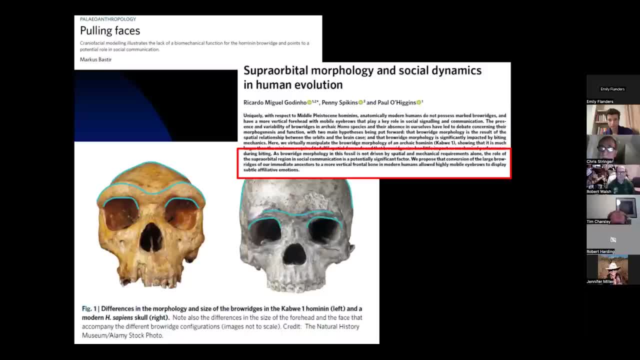 function from the hominid brown ridge and function from the hominid brown ridge and points to a potential role in social points, to a potential role in social points, to a potential role in social communication. so there could have been communication. so there could have been. 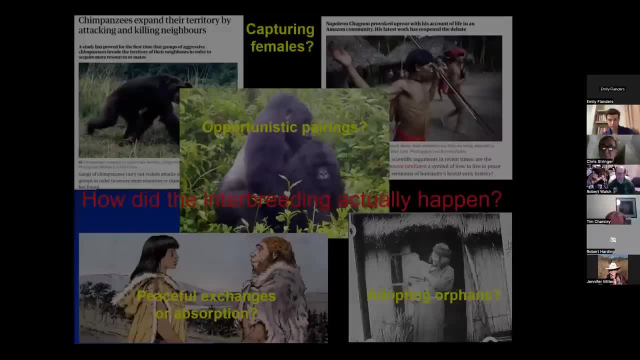 communication. so there could have been differences in social signaling, between differences in social signaling, between differences in social signaling between us and the neanderthals, us and the neanderthals, us and the neanderthals. and how did those interbreedings actually? 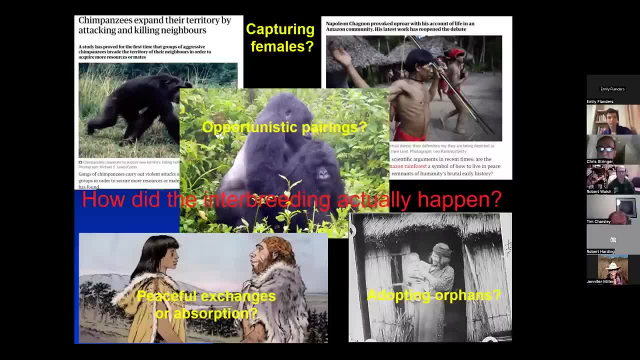 and how did those interbreedings actually? and how did those interbreedings actually happen? well, because we haven't got the happen. well, because we haven't got the happen well, because we haven't got the faintest idea, faintest idea, faintest idea. there are lots of possibilities and and 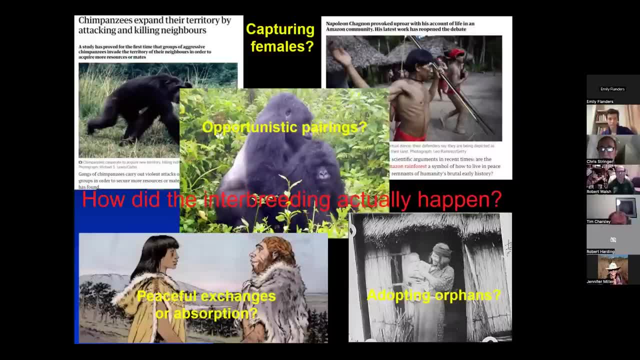 there are lots of possibilities, and, and there are lots of possibilities, and, and, indeed, all of these could have happened. indeed, all of these could have happened. indeed, all of these could have happened at times, at times, at times, females could have been captured from one. females could have been captured from one. 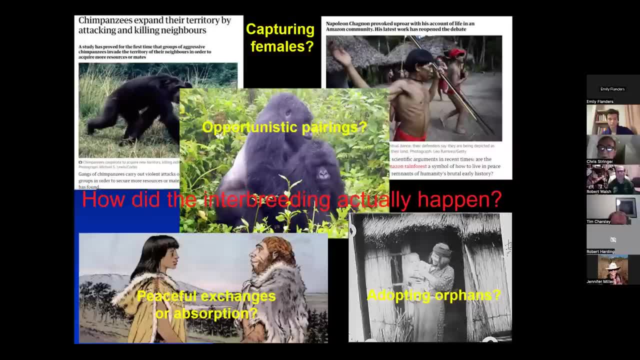 females could have been captured from one group to another group, to another group, to another, into homo sapiens groups and then into homo sapiens groups, and then into homo sapiens groups and then breeding on in those groups. there could breeding on in those groups. there could. 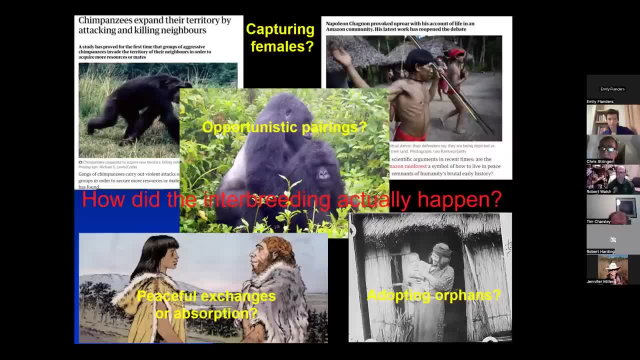 breeding on in those groups. there could have been opportunistic pairings. have been opportunistic pairings. have been opportunistic pairings- people moving away from their regular people, moving away from their regular people, moving away from their regular partners and partners and partners and and having sex with. 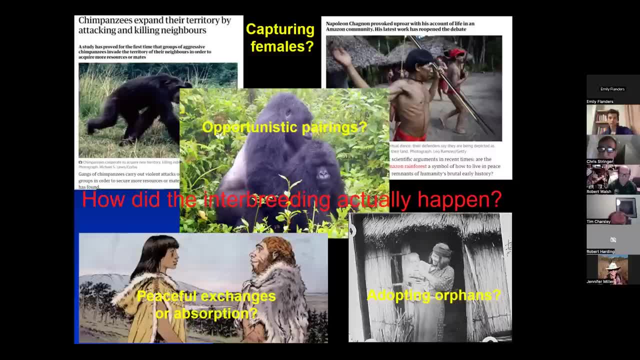 and having sex with, and having sex with a member of another population, another a member of another population, another a member of another population, another species, species, species. there could have been peaceful exchanges. there could have been peaceful exchanges. there could have been peaceful exchanges if these groups were on the landscape. 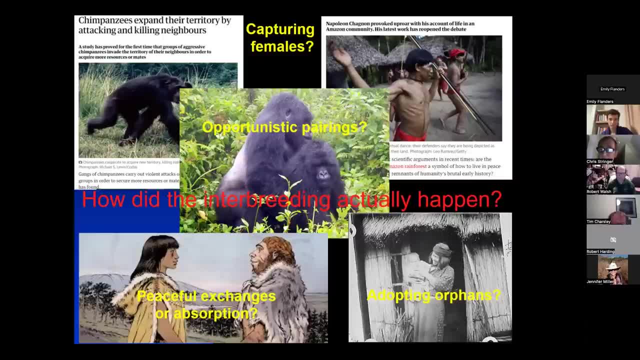 if these groups were on the landscape, if these groups were on the landscape long enough, long enough, long enough, populations could have been peacefully. populations could have been peacefully. populations could have been peacefully absorbed into into other populations, absorbed into into other populations, absorbed into into other populations. um orphans could have been adopted, uh. 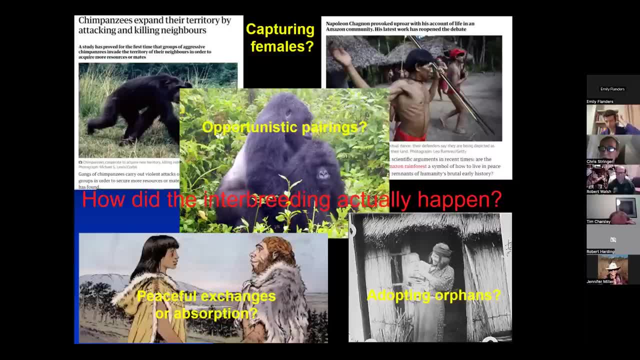 um orphans could have been adopted. uh, um orphans could have been adopted. uh, neanderthal babies that were orphaned. uh, perhaps homo sapiens groups actually, perhaps homo sapiens groups actually, perhaps homo sapiens groups actually adopted them and brought them up as adopted them and brought them up as. 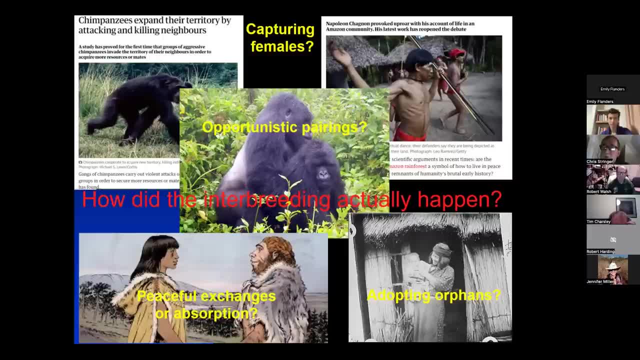 adopted them and brought them up as their own, their own, their own. so all of these things could have been so, all of these things could have been so, all of these things could have been ways in which there was gene flow from, ways in which there was gene flow from. 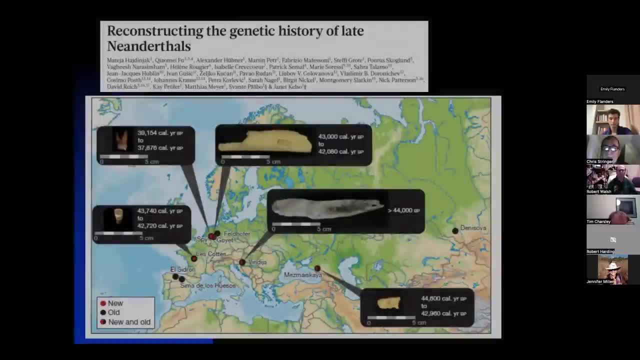 ways in which there was gene flow from neanderthals into homo sapiens. one of the interesting things is that on one of the interesting things is that on one of the interesting things is that on the data at the moment we've got the data at the moment we've got. 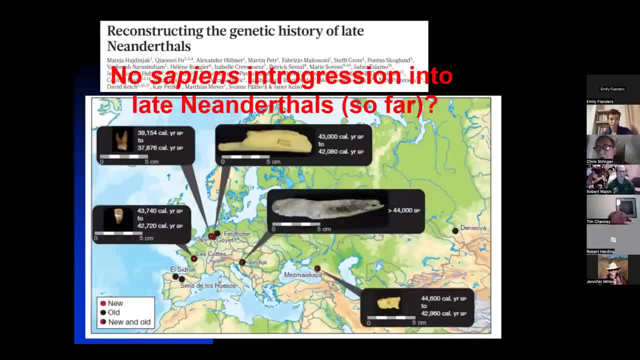 the data at the moment. we've got quite a lot of evidence of neanderthal dna, quite a lot of evidence of neanderthal dna, quite a lot of evidence of neanderthal dna entering the early homo sapiens gene, entering the early homo sapiens gene. 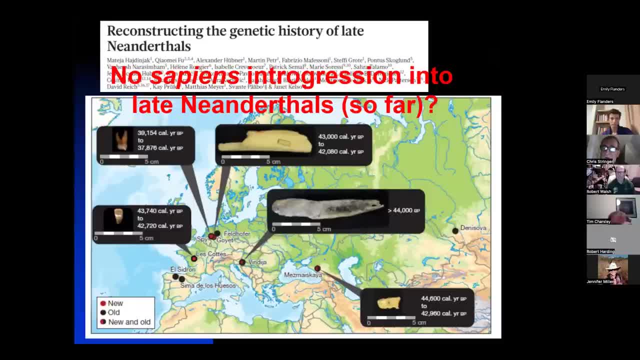 entering the early homo sapiens gene pool from fossils, pool from fossils, pool from fossils. but so far on the evidence of the late. but so far on the evidence of the late, but so far on the evidence of the late neanderthals- neanderthals- 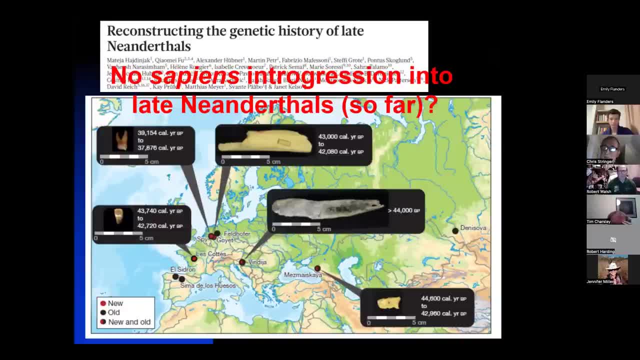 neanderthals that have been sequenced? there's no that have been sequenced. there's no that have been sequenced. there's no evidence of homo sapiens dna. evidence of homo sapiens dna, evidence of homo sapiens dna entering those populations, so there's no. 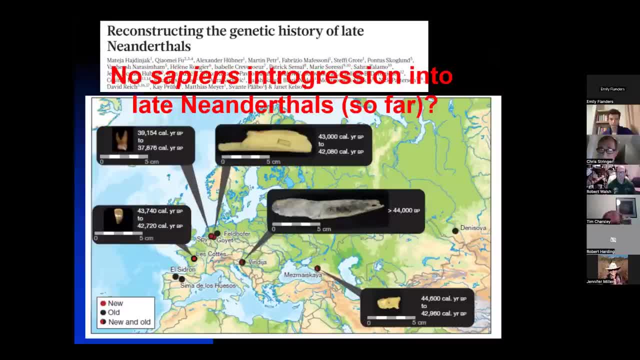 entering those populations. so there's no entering those populations, so there's no sapiens integration, sapiens integration, sapiens integration into late neanderthals so far and of into late neanderthals so far, and of into late neanderthals so far, and of course that could change. 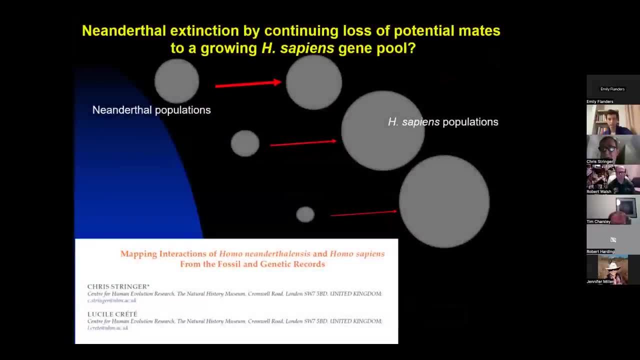 course that could change course that could change um. but this is something which lucille um. but this is something which lucille um. but this is something which lucille and i proposed in in our paper that and i proposed in in our paper that and i proposed in in our paper that perhaps this might be. 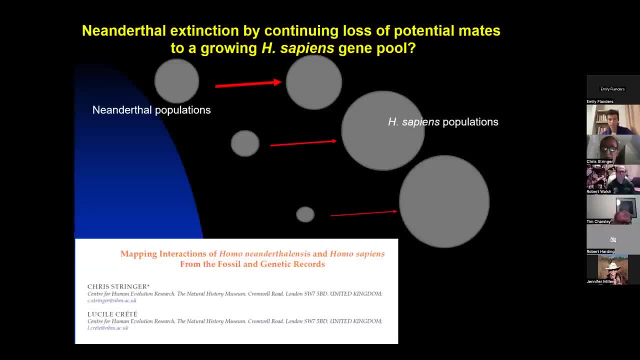 perhaps this might be, perhaps this might be one mechanism that contributed to the one mechanism that contributed to the one mechanism that contributed to the disappearance of the neanderthals. that disappearance of the neanderthals, that disappearance of the neanderthals, that, if there was mainly a one-way gene flow, 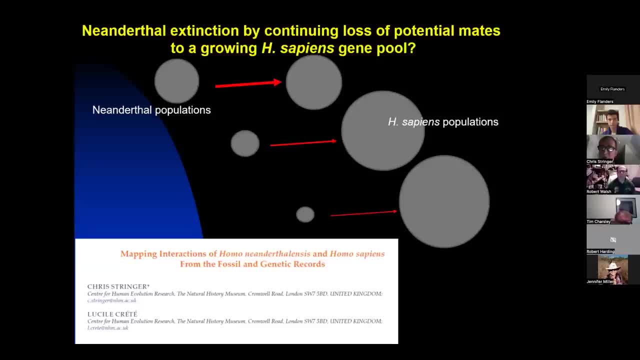 if there was mainly a one-way gene flow, if there was mainly a one-way gene flow from neanderthal populations into homo, from neanderthal populations into homo, from neanderthal populations into homo sapiens populations, sapiens populations and the neanderthal numbers were already. 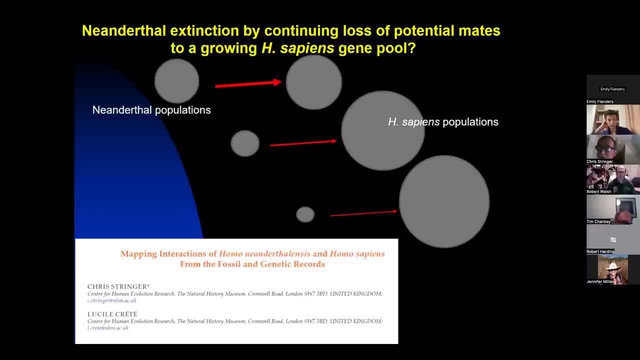 and the neanderthal numbers were already. and the neanderthal numbers were already quite low, quite low, quite low. this may have contributed to the physical. this may have contributed to the physical. this may have contributed to the physical extinction of the neanderthals, because 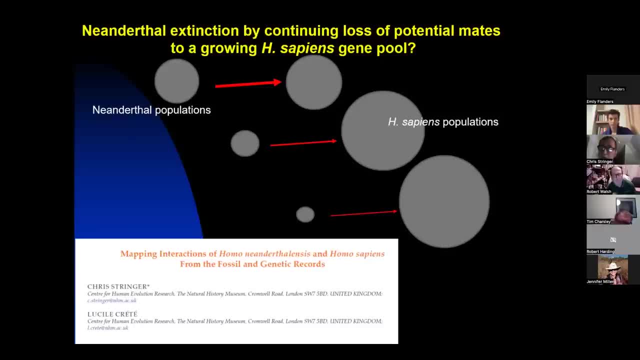 extinction of the neanderthals. because extinction of the neanderthals, because losing your breeding individuals, to losing your breeding individuals, to losing your breeding individuals to another population, another population, another population, is obviously going to be detrimental if is obviously going to be detrimental if. 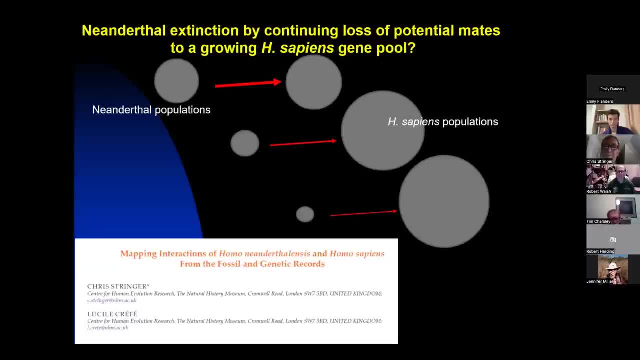 is obviously going to be detrimental if your own population numbers are very low. so in the future, i think we've got a lot. so in the future, i think we've got a lot. so in the future, i think we've got a lot of exciting future to look forward to. so 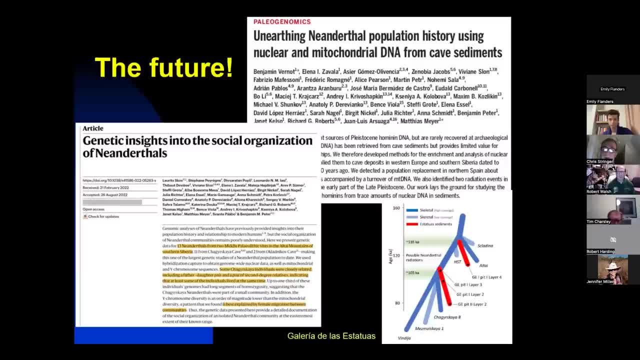 of exciting future to look forward to. so of exciting future to look forward to. so one of the main contributors- i think is one of the main contributors, i think is one of the main contributors, i think- is going to be going to be going to be obviously continuing to get dna uh more. 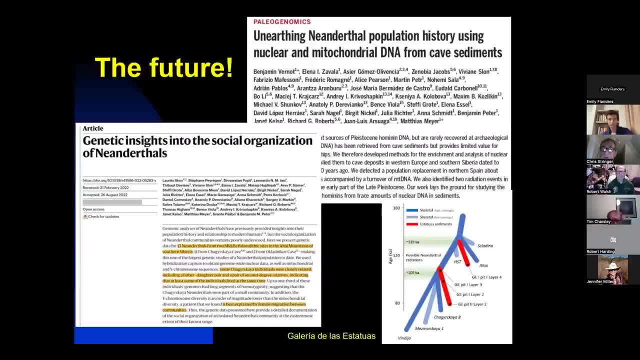 obviously continuing to get dna uh. more obviously continuing to get dna uh, more dna sequences, but also sediment dna dna sequences, but also sediment dna dna sequences, but also sediment dna sequences, sequences, sequences, so sites which don't have fossils, but so sites which don't have fossils, but 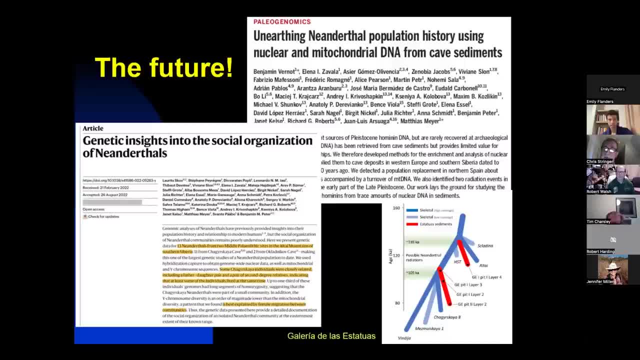 so sites which don't have fossils but have traces of human occupation may have have traces of human occupation, may have have traces of human occupation, may have dna by those occupants, and so we're dna by those occupants, and so we're dna by those occupants, and so we're starting to build up. 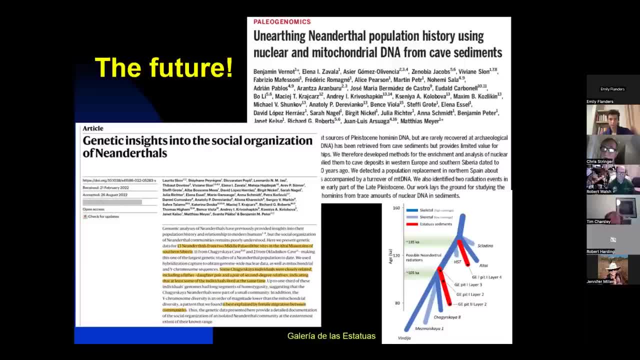 starting to build up. starting to build up sequences of neanderthals and denisovans. sequences of neanderthals and denisovans. sequences of neanderthals and denisovans: purely from cave sediments and we can. purely from cave sediments and we can. 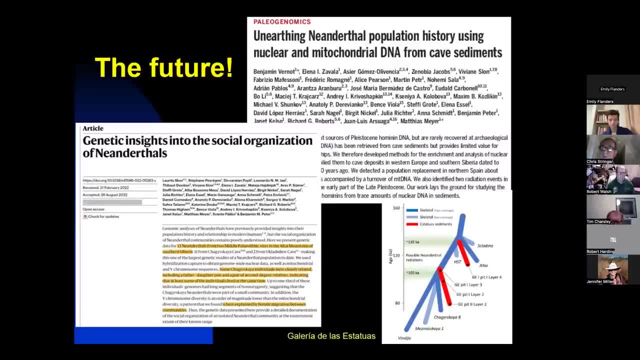 purely from cave sediments and we can look at the relationships. if we're lucky, look at the relationships. if we're lucky, look at the relationships. if we're lucky. if the data are good enough, we can. if the data are good enough, we can. if the data are good enough, we can actually build up evidence of 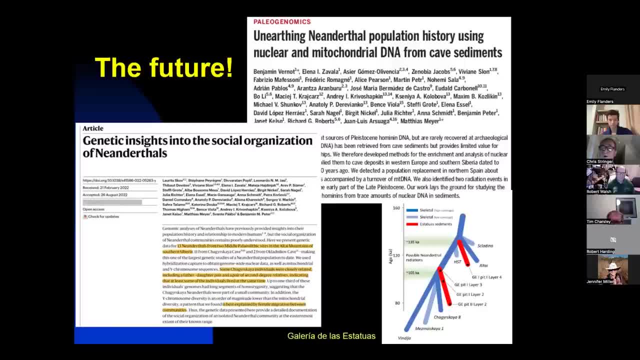 actually build up evidence of, actually build up evidence of relationships and we're starting to get relationships. and we're starting to get relationships and we're starting to get these pictures through of possible, these pictures through of possible, these pictures through of possible social structures of the neanderthals. 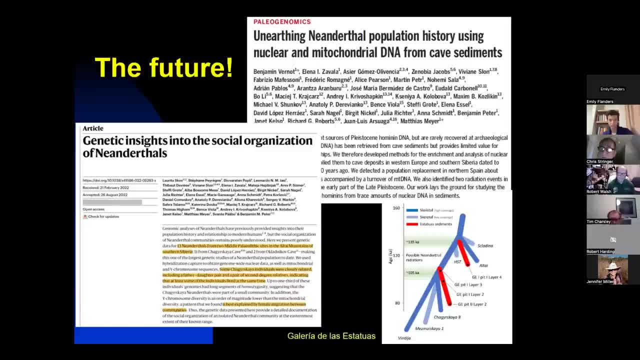 social structures of the neanderthals, social structures of the neanderthals and potentially relationships close and potentially relationships close and potentially relationships close around a first generation hybrid of a around a first generation hybrid of a around a first generation hybrid of a denisovan and a neanderthal. so an 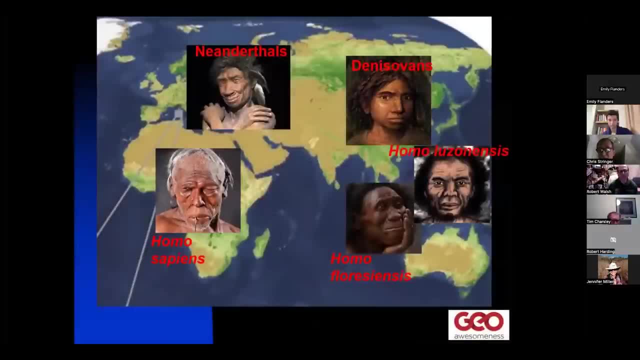 denisovan and a neanderthal, so an denisovan and a neanderthal, so an exciting future here. so moving on to the end, now we've got. so moving on to the end, now we've got. so moving on to the end, now we've got that. of course, big question of why we 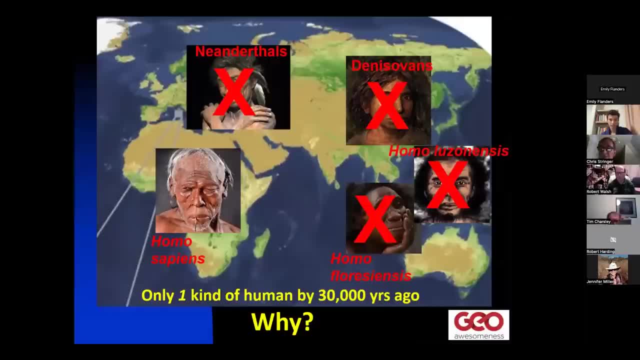 that, of course, big question of why we that, of course, big question of why we are the only human species left. there are the only human species left. there are the only human species left. there was all this diversity, even 70 000, was all this diversity, even 70 000. 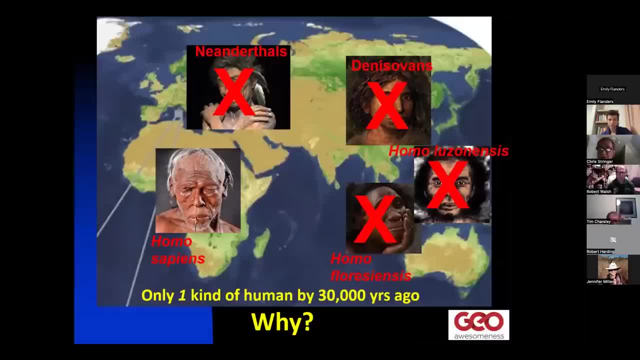 was all this diversity even 70 000 years ago, years ago. years ago, we had homo sapiens evolving in africa. we had homo sapiens evolving in africa. we had homo sapiens evolving in africa, the neanderthals evolving in european, the neanderthals evolving in european. 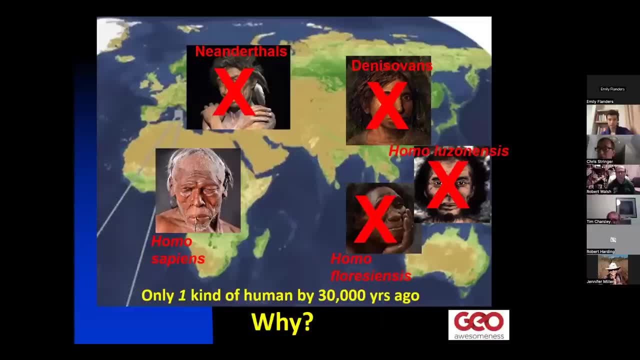 the neanderthals evolving in european asia. the denisovans were in east asia, asia. the denisovans were in east asia, asia. the denisovans were in east asia, on the islands of southeast asia we had on the islands of southeast asia. we had 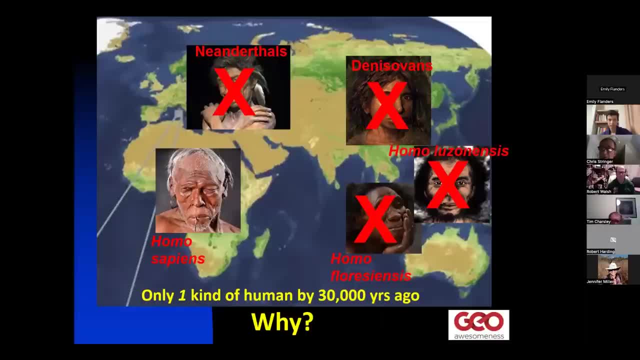 on the islands of southeast asia, we had homo floresiensis, homo floresiensis, homo floresiensis and homo lucidensis, these, these dwarf and homo lucidensis, these these dwarf and homo lucidensis, these these dwarf human species. they were, they were all. 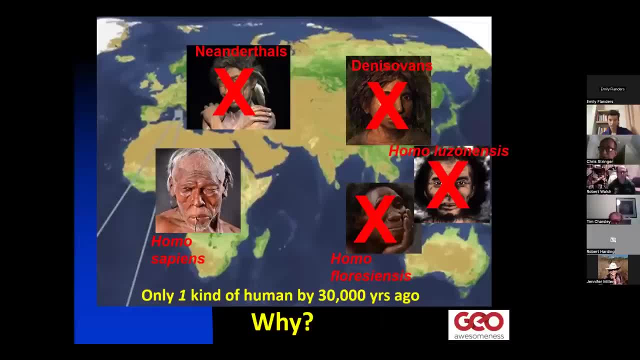 human species. they were, they were all human species, they were, they were all there about 70 000 years ago, there about 70 000 years ago, there about 70 000 years ago, and yet by 30 000 years ago as far as, and yet by 30 000 years ago as far as. 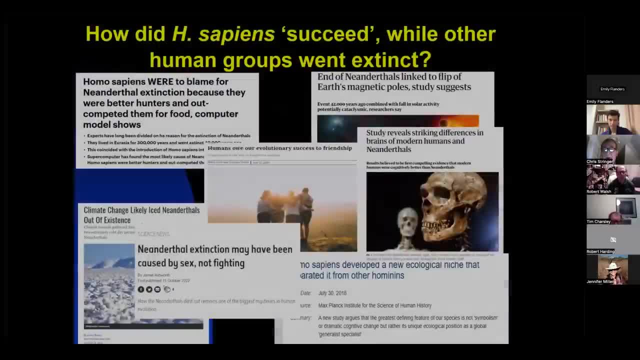 and yet by 30 000 years ago, as far as we know, they'd all gone. so why is that we know they'd all gone? so why is that we know they'd all gone? so why is that? well, well, well, many explanations have been offered, and 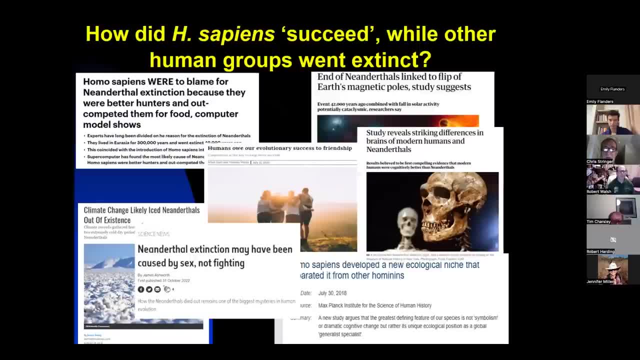 many explanations have been offered and many explanations have been offered, and here and here they summarize from the here and here they summarize from the here and here they summarize from the popular literature, popular literature, popular literature: uh, homo sapiens were to blame for. uh, homo sapiens were to blame for. 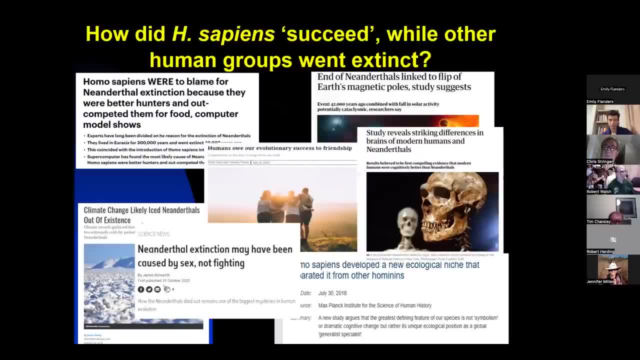 uh, homo sapiens were to blame for neanderthal extinction. because they're neanderthal extinction, because they're neanderthal extinction because they're better hunters and out competed them for better hunters and out competed them for better hunters and out competed them for food. a computer model shows: 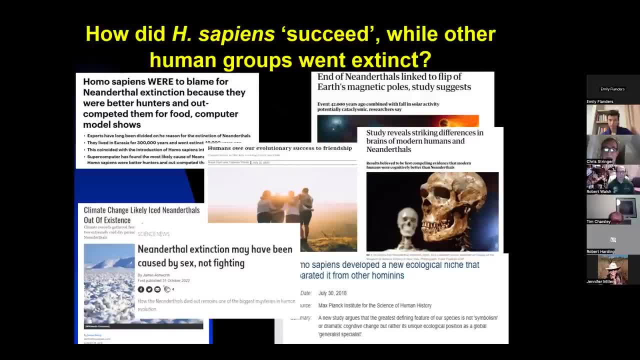 food. a computer model shows food. a computer model shows bottom left. the suggestion that climate bottom left. the suggestion that climate bottom left, the suggestion that climate change iced the neanderthals out of change, iced the neanderthals out of change, iced the neanderthals out of existence. there were two extremely cold. 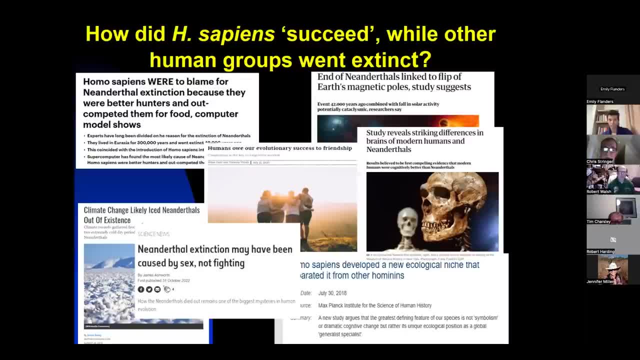 existence. there were two extremely cold existence. there were two extremely cold, dry periods. dry periods, dry periods close to the time of neanderthal, close to the time of neanderthal, close to the time of neanderthal. extinction, extinction, extinction. on the top right there, this suggestion. 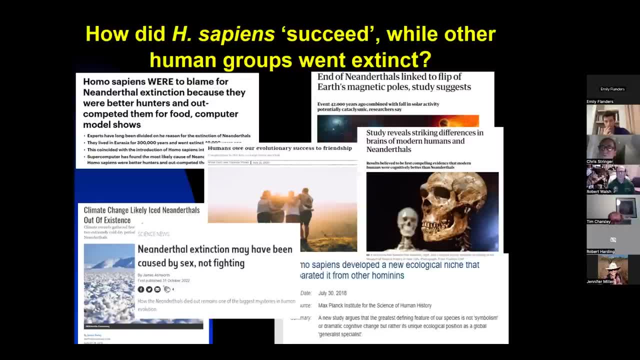 on the top right there. this suggestion on the top right there, this suggestion that that that the end of the neanderthals was linked to the end of the neanderthals was linked to the end of the neanderthals was linked to a flip of the earth's magnetic poles. 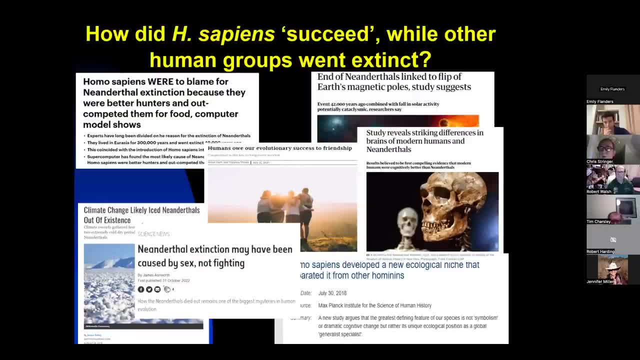 a flip of the earth's magnetic poles. a flip of the earth's magnetic poles, an event 42 000 years ago, combined with an event 42 000 years ago, combined with an event 42 000 years ago, combined with a fall in solar activity, was 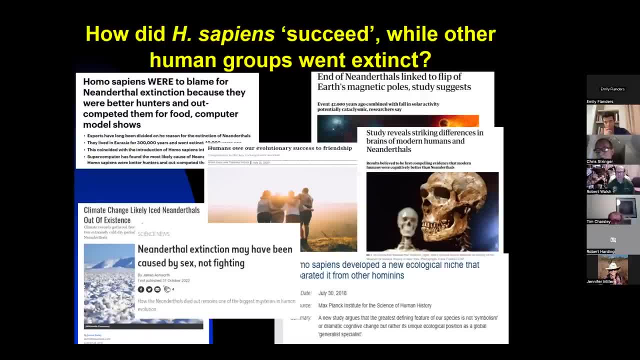 a fall in solar activity was a fall in solar activity was potentially cataclysmic, potentially cataclysmic. potentially cataclysmic, um i mean the problem with that model, um i mean the problem with that model, um i mean the problem with that model and with the climate change model is. 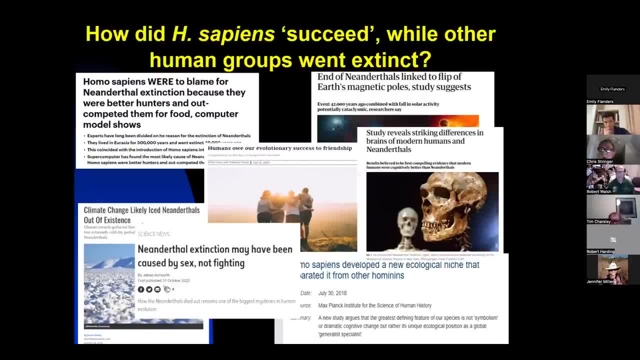 and with the climate change model is. and with the climate change model is because that this isn't just going to, because that this isn't just going to, because that this isn't just going to impact neanderthals: it's going to impact, impact neanderthals, it's going to impact. 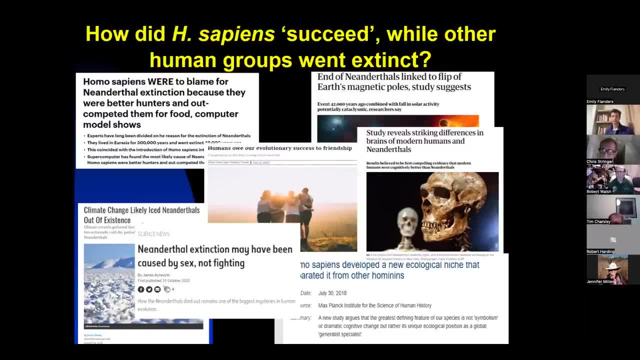 impact neanderthals. it's going to impact everything, um so, everything, um so, everything, um so. you know we're really looking for some. you know we're really looking for some. you know we're really looking for some that's more specific to the neanderthal. 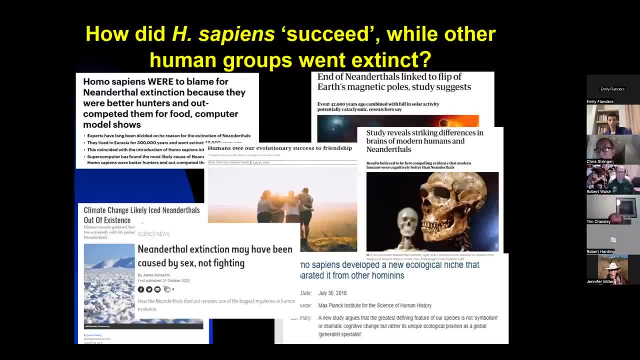 that's more specific to the neanderthal, that's more specific to the neanderthal sapiens relationship. we mentioned that sapiens relationship. we mentioned that sapiens relationship. we mentioned that brain study there on the right hand side. brain study there on the right hand side. 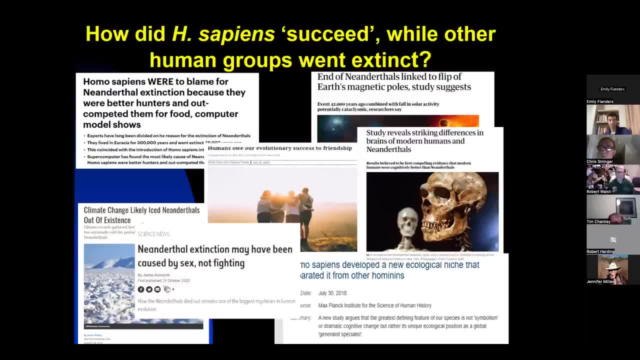 brain study there on the right hand side. their study reveals striking differences. their study reveals striking differences. their study reveals striking differences in the brains of modern humans and in the brains of modern humans and in the brains of modern humans and neanderthals- neanderthals. 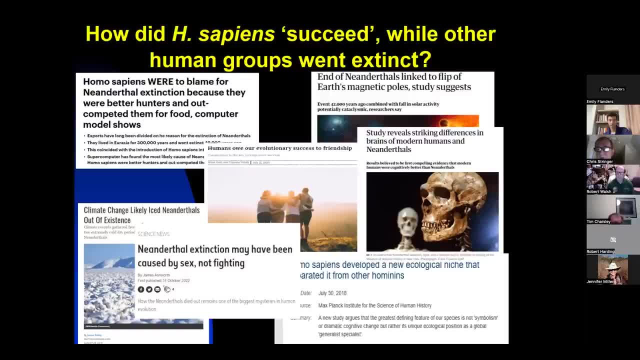 neanderthals. the results are believed to be the first. the results are believed to be the first. the results are believed to be the first compelling evidence, that modern compelling evidence, that modern compelling evidence that modern humans are cognitively better than humans are cognitively better than. 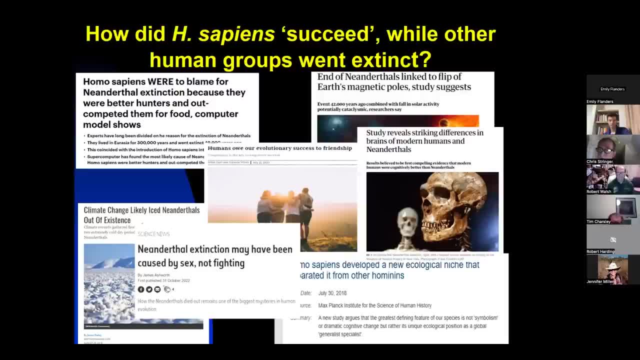 humans are cognitively better than neanderthals. well, i'm not sure about neanderthals. well, i'm not sure about neanderthals. well, i'm not sure about that. but in terms of neuron density, that, but in terms of neuron density. 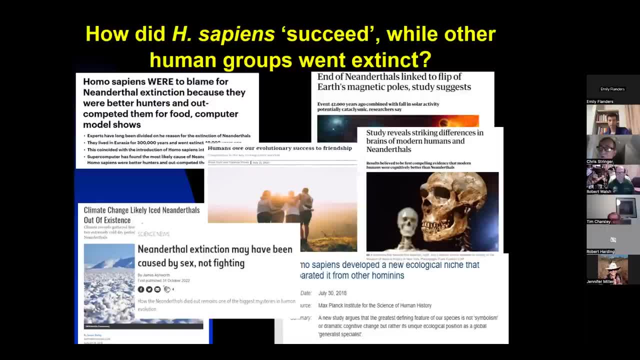 that. but in terms of neuron density, yes, maybe we did have a a greater growth. yes, maybe we did have a a greater growth. yes, maybe we did have a a greater growth of neurons early on in of neurons, early on in of neurons early on in in child development. um, on the bottom, 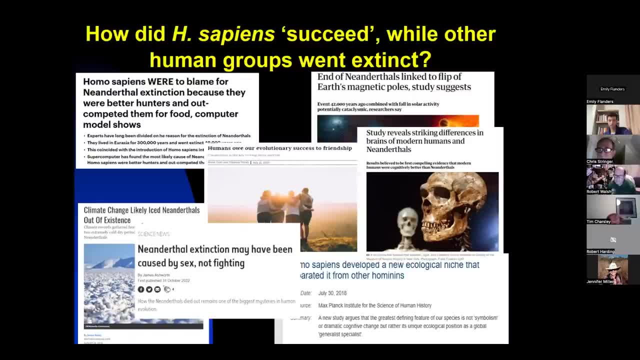 in child development. um, on the bottom in child development. um, on the bottom, right there, right there, right there um. homo sapiens developed a new ecological um. homo sapiens developed a new ecological um. homo sapiens developed a new ecological niche that separated it from niche that separated it from. 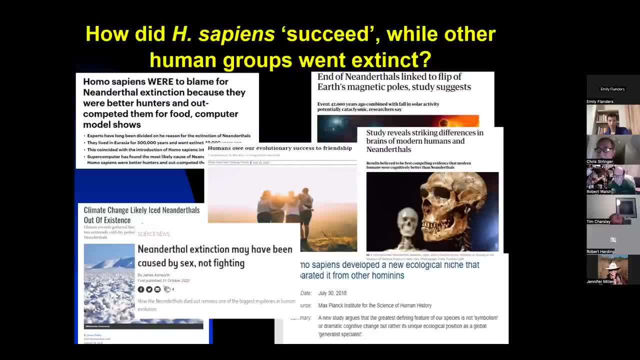 niche that separated it from other hominins. a new study argues that other hominins. a new study argues that other hominins. a new study argues that the greatest defining feature of our, the greatest defining feature of our, the greatest defining feature of our species, is not symbolism or dramatic. 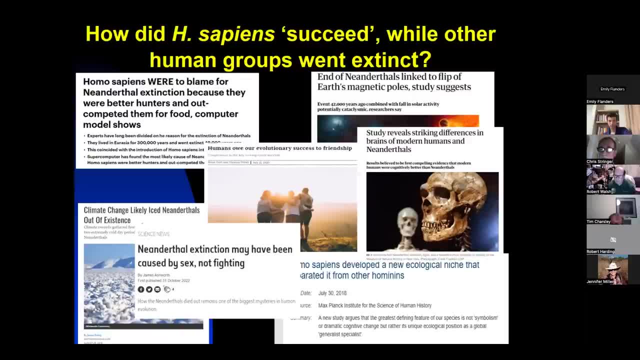 species is not symbolism or dramatic species is not symbolism or dramatic cognitive change, but rather its unique cognitive change, but rather its unique cognitive change, but rather its unique ecological position as a global ecological position, as a global ecological position as a global generalist specialist. generalist specialist. 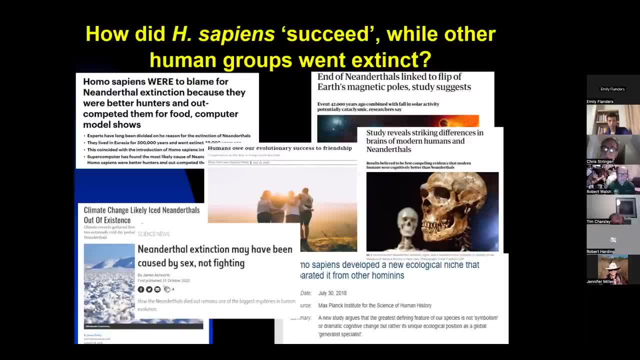 generalist specialist in the center there, the idea that we in the center there, the idea that we in the center there, the idea that we owe our evolutionary success to owe our evolutionary success, to owe our evolutionary success to friendship. so cooperation was the key: friendship. so cooperation was the key. 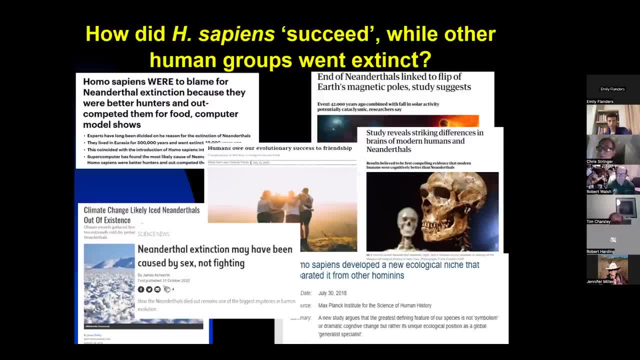 friendship. so cooperation was the key to our survival and our success, that we to our survival and our success, that we to our survival and our success, that we were less aggressive within groups than were less aggressive within groups, than were less aggressive within groups than some of these other earlier humans were. 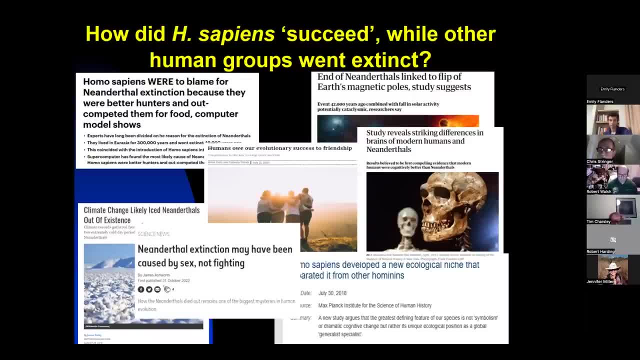 some of these other earlier humans were, some of these other earlier humans were, and that led to the development of, and that led to the development of, and that led to the development of friendships. wider networking led to our friendships. wider networking led to our friendships. wider networking led to our revolution success. 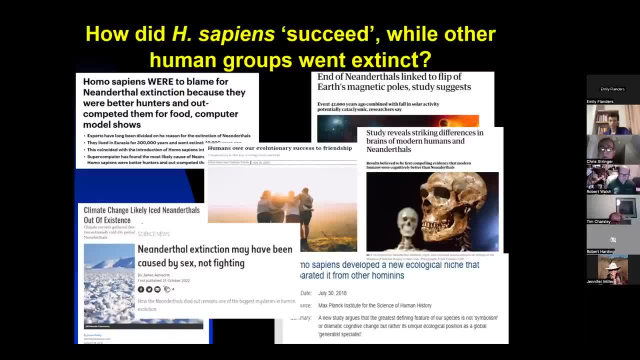 revolution success, revolution, success. and then the suggestion uh from lucille, and then the suggestion uh from lucille, and then the suggestion uh from lucille and i that neanderthal extinction may and i that neanderthal extinction may and i that neanderthal extinction may have been caused actually by the 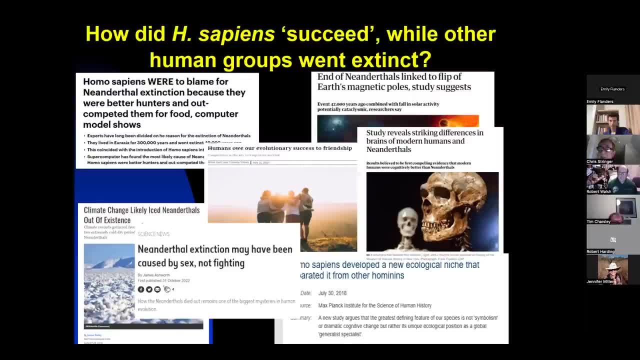 have been caused actually by the have been caused actually by the interbreeding with homo sapiens. if that interbreeding with homo sapiens, if that interbreeding with homo sapiens, if that interbreeding was mainly going in one interbreeding was mainly going in one. 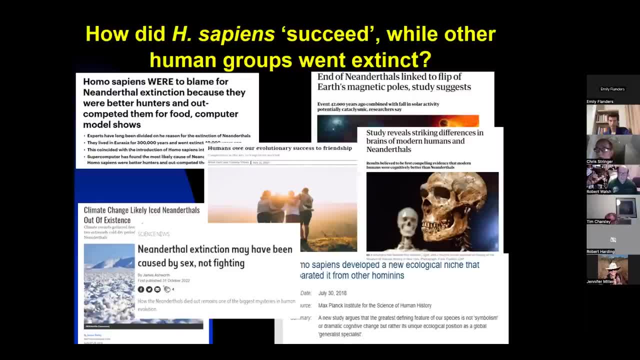 interbreeding was mainly going in one direction, direction: direction. then it may have led to a depletion of, then it may have led to a depletion of, then it may have led to a depletion of neanderthal populations, neanderthal populations, neanderthal populations. yeah, so these are all possibilities, and 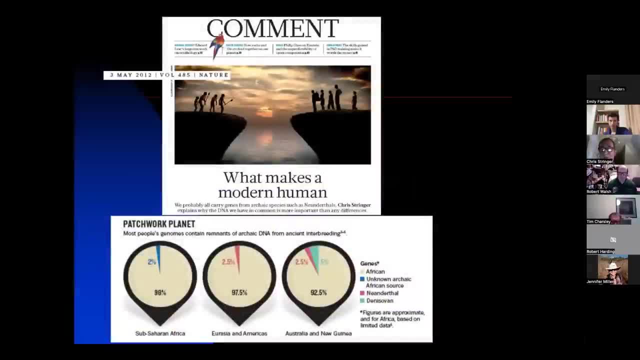 yeah, so these are all possibilities. and yeah, so these are all possibilities, and no doubt there are many more. you can no doubt there are many more. you can no doubt there are many more you can think of, think of, think of. so finally then, yes, so what makes a? 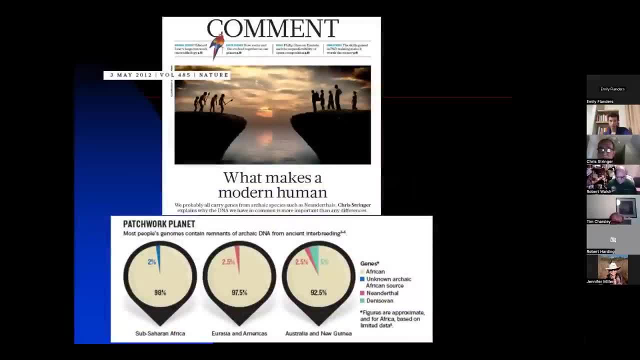 so finally then, yes, so what makes a? so? finally then, yes, so what makes a modern human? modern human, modern human- uh, we are mostly out of africa. i think, uh, we are mostly out of africa. i think, uh, we are mostly out of africa. i think that's the way to summarize it. 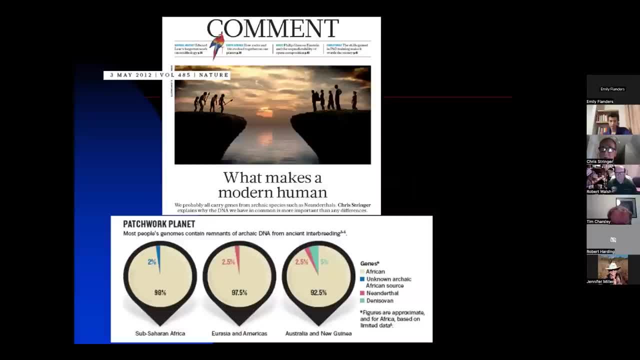 that's the way to summarize it. that's the way to summarize it um that. we're not a hundred percent um that. we're not a hundred percent um that, we're not a hundred percent recent african origin. we are recent african origin. we are recent african origin. we are part neanderthal, part denisovan, and 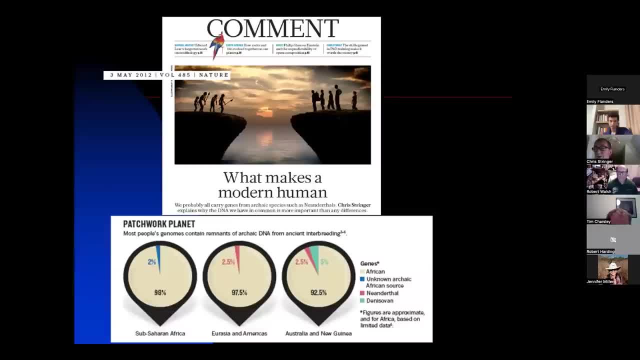 part neanderthal, part denisovan and part neanderthal part denisovan. and even african populations may have a. even african populations may have a. even african populations may have a component of component of component of introgression from uh another species. introgression from uh another species. 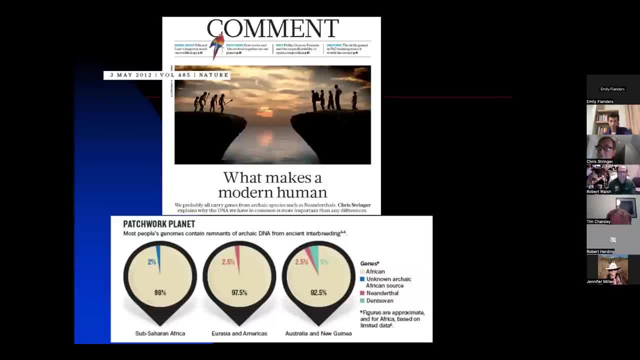 introgression from, uh, another species within africa. so we are not a hundred within africa, so we are not a hundred within africa, so we are not a hundred percent recent african, as i would have. percent recent african, as i would have percent recent african, as i would have, uh, commented before. so how best to? 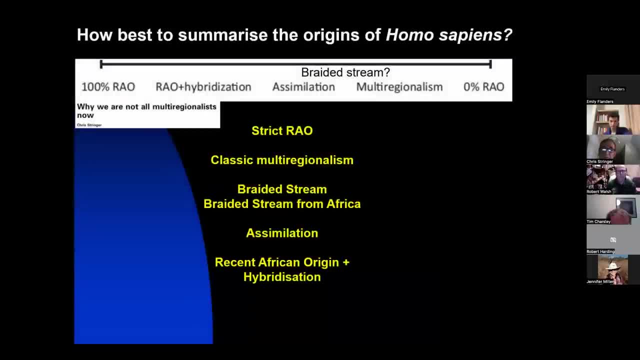 uh commented before. so how best to uh commented before. so how best to summarize our origins? well, this is a summarize our origins. well, this is a summarize our origins. well, this is a diagram, diagram. diagram from a paper i i wrote about eight years. from a paper i i wrote about eight years. 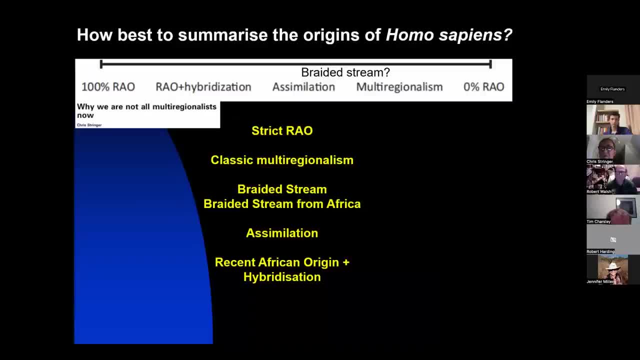 from a paper i i wrote about eight years ago. so we can see here a kind of ago. so we can see here a kind of ago. so we can see here a kind of spectrum of, of spectrum of, of spectrum of of these ideas that we've got a hundred. 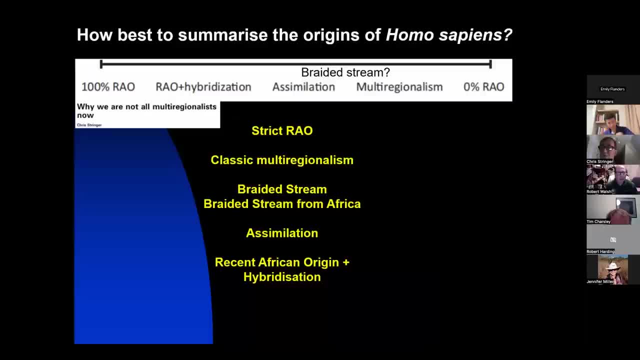 these ideas that we've got a hundred. these ideas that we've got a hundred percent recent african origin over on percent recent african origin over on percent recent african origin over on the left and naught percent recent the left and naught percent recent the left and naught percent recent african origin over on the right hand. 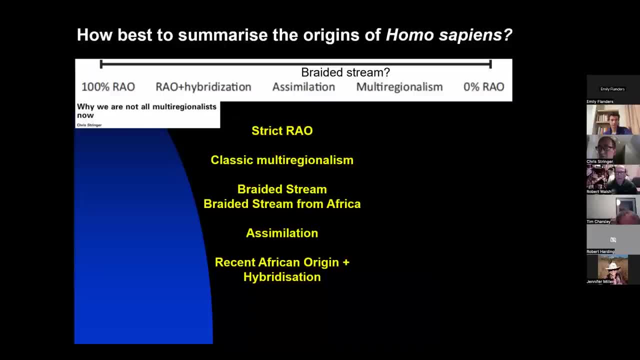 african origin over on the right hand, african origin over on the right hand side. ideas like clark howells or christy side. ideas like clark howells or christy side. ideas like clark howells or christy turner's view that homo sapiens. 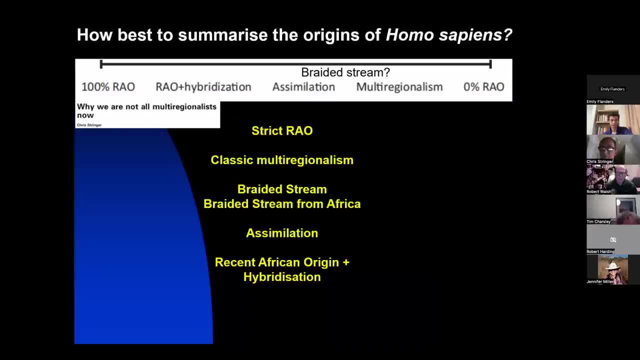 turner's view that homo sapiens turner's view that homo sapiens originated in asia, originated in asia, originated in asia as a single region and then in between as a single region, and then in between as a single region, and then in between we've got these kind of 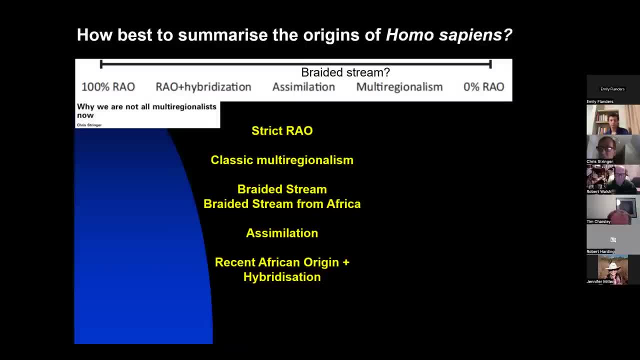 we've got these kind of. we've got these kind of models such as recent african origin and models such as recent african origin and models such as recent african origin. and hybridization, hybridization, hybridization- good to broers model assimilation- good to broers model assimilation. 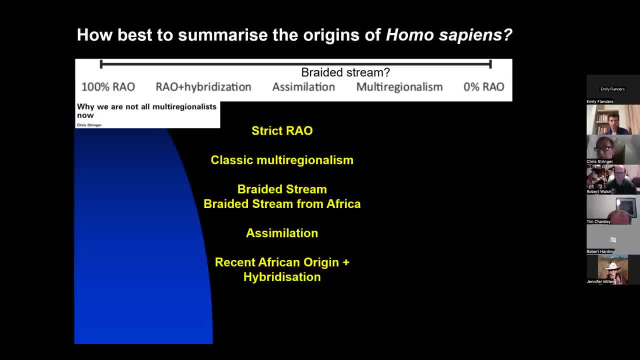 good to broers model assimilation. linked with fred smith and eric. linked with fred smith and eric. linked with fred smith and eric. drinkhouse, multi-regionalism, drinkhouse, multi-regionalism, drinkhouse, multi-regionalism- uh. linked with people like milford. 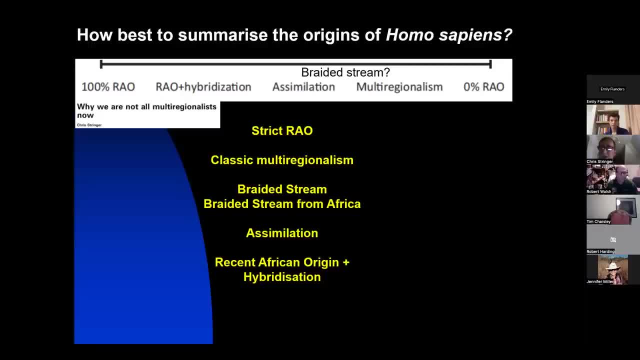 uh, linked with people like milford. uh, linked with people like milford, walpole, walpole, walpole. so which of these is really the most so? which of these is really the most so? which of these is really the most accurate label? well, accurate label. well, accurate label. well, i think, a strict recent african origin. 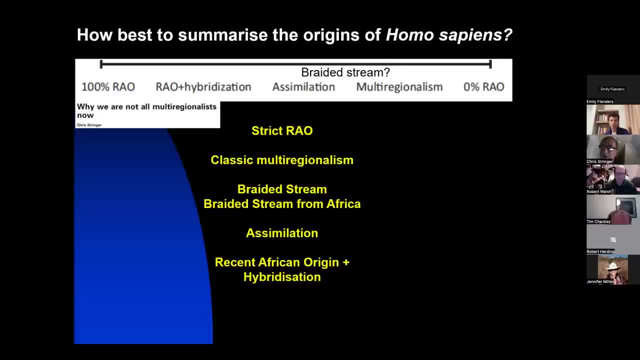 i think a strict recent african origin. i think a strict recent african origin model, as we've said it's. it's not model. as we've said it's it's not model. as we've said it's it's not tenable anymore. we are not a hundred. 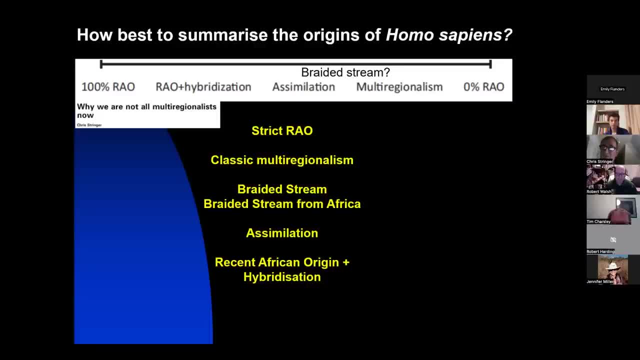 tenable anymore. we are not a hundred tenable anymore. we are not a hundred percent, percent, percent recent african origin. we do have recent african origin. we do have recent african origin. we do have components from components from components from other populations in our genomes, other populations in our genomes. 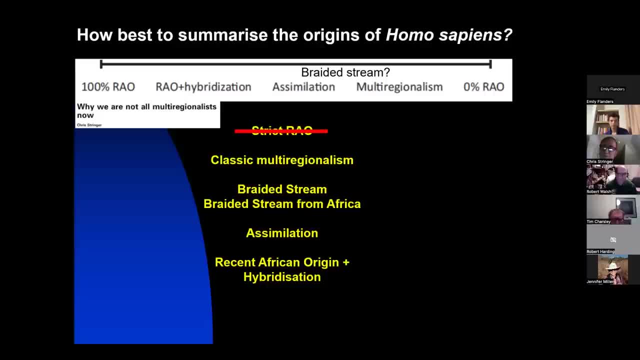 other populations in our genomes, classic multi-regionalism, i think has. classic multi-regionalism, i think has classic multi-regionalism, i think has has certainly been falsified. uh, there's has certainly been falsified. uh, there's has certainly been falsified. uh, there's no evidence that uh. 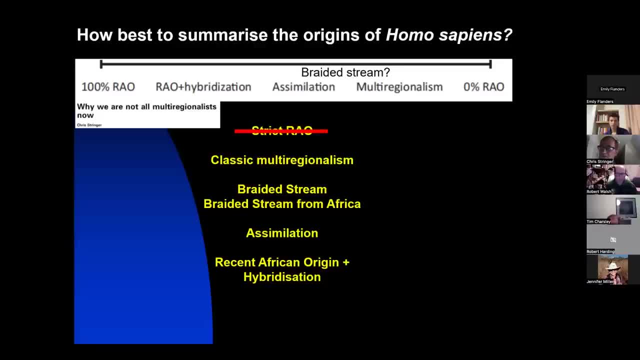 no evidence that uh, no evidence that uh. early populations in china, such as homo early populations in china, such as homo early populations in china, such as homo erectus, gave rise to erectus, gave rise to erectus gave rise to to recent chinese populations: no. to recent chinese populations, no. 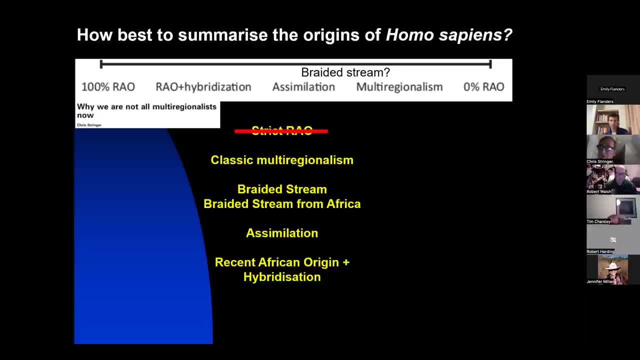 to recent chinese populations. no evidence that indonesian homo erectus. evidence that indonesian homo erectus. evidence that indonesian homo erectus gave rise to recent native australian gave rise to recent native australian gave rise to recent native australian populations. 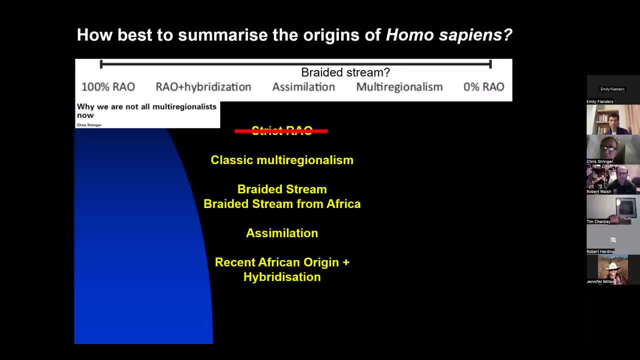 populations, populations. no evidence that neanderthals directly no evidence that neanderthals directly, no evidence that neanderthals directly evolved into into recent europeans. so i evolved into into recent europeans, so i evolved into into recent europeans. so i think that's falsified too. 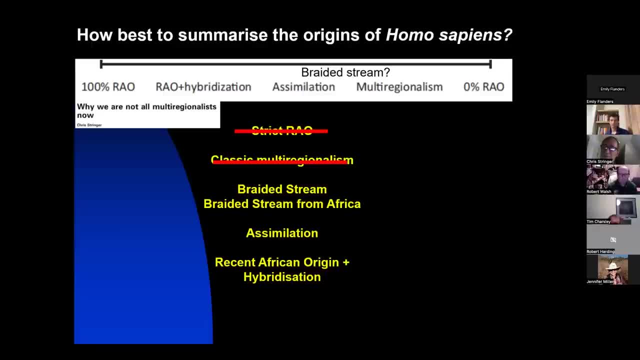 think that's falsified too. think that's falsified too. the braided stream model has become the braided stream model has become the braided stream model has become popular, popular, popular, and this i find difficult to distinguish. and this i find difficult to distinguish, and this i find difficult to distinguish from multi-regionism in its arguments. 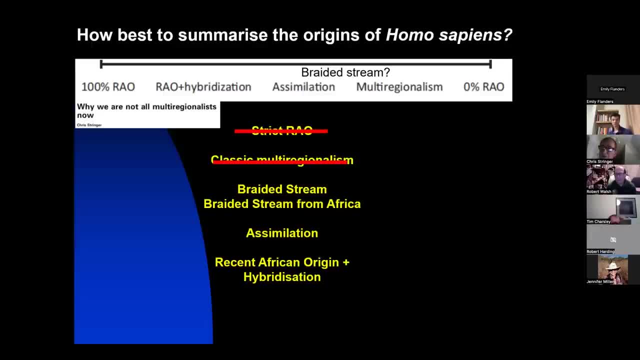 from multi-regionism in its arguments, from multi-regionism in its arguments, but the argument is that you have this, but the argument is that you have this, but the argument is that you have this, this river that's flowing across the, this river that's flowing across the. 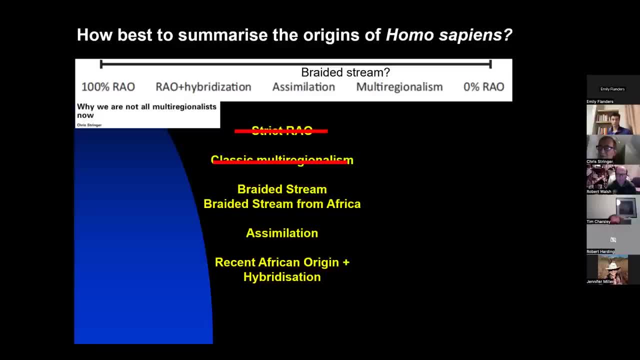 this river that's flowing across the inhabited world and little streams and inhabited world and little streams and inhabited world and little streams and rivulets come and go, they merge, they. rivulets come and go, they merge, they rivulets come and go, they merge, they separate, they come back together and so 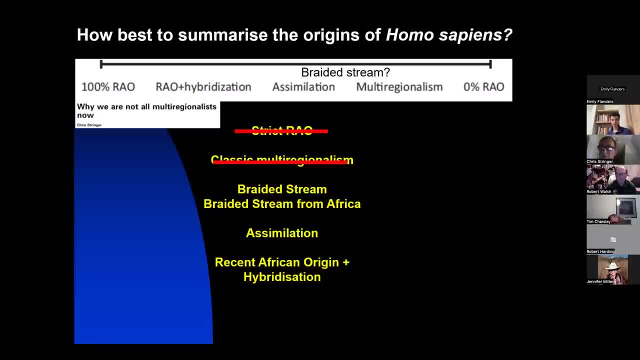 separate, they come back together, and so separate, they come back together. and so we have this braided stream pattern, for we have this braided stream pattern, for we have this braided stream pattern for the evolution of homo sapiens, but if the evolution of homo sapiens, but if 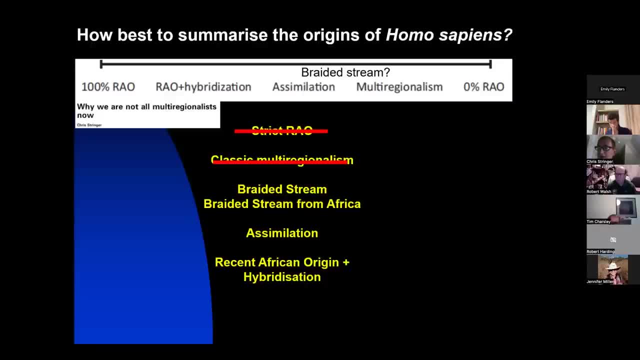 the evolution of homo sapiens. but if that pattern is there, then i would say that pattern is there, then i would say that pattern is there, then i would say that the african pattern is predominant, that the african pattern is predominant, that the african pattern is predominant. you know our morphological data, our 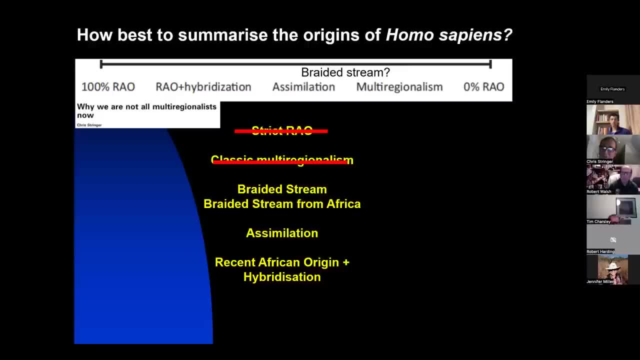 you know our morphological data. our you know our morphological data. our genetic data suggests that genetic data suggests that genetic data suggests that africa dominates the story of homo africa dominates the story of homo africa dominates the story of homo sapiens origin. and so i think we'd have 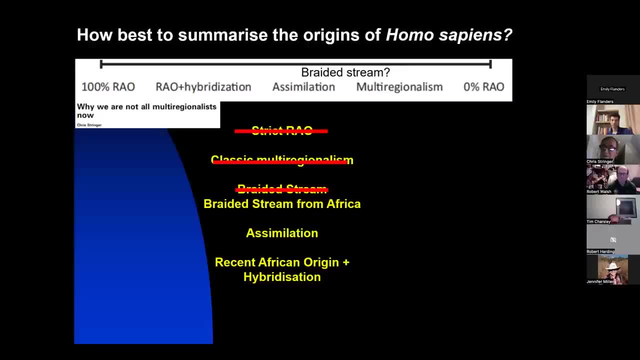 sapiens origin, and so i think we'd have sapiens origin, and so i think we'd have to call it. if it's a braided stream, it's to call it. if it's a braided stream, it's to call it. if it's a braided stream, it's a braided stream from africa. 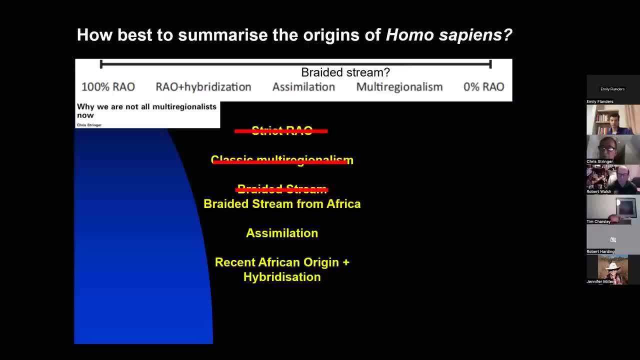 a braided stream from africa, a braided stream from africa, and then we're left with assimilation, and then we're left with assimilation, and then we're left with assimilation and recent african origin and and recent african origin and and recent african origin and hybridization and, in my view, 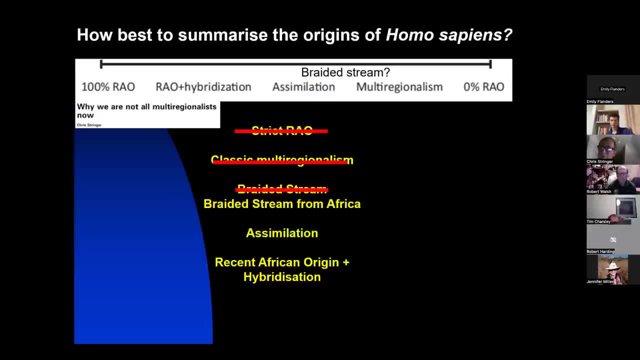 hybridization and, in my view, hybridization and, in my view, the data at the moment support the data at the moment support the data at the moment support a recent african origin and a recent african origin and a recent african origin and hybridization that the main gene flow. 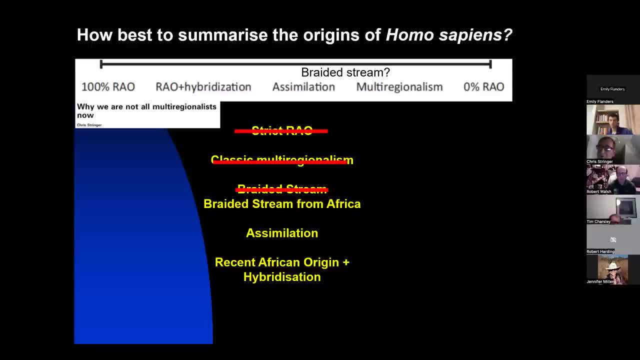 hybridization that the main gene flow, hybridization that the main gene flow is going from these resident, is going from these resident, is going from these resident populations outside of africa, from populations outside of africa, from populations outside of africa, from neanderthals and from genicivans. 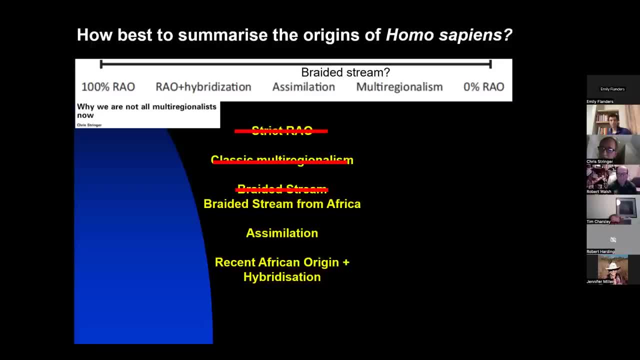 neanderthals and from genicivans neanderthals and from genicivans into the homo sapiens populations, into the homo sapiens populations, into the homo sapiens populations. there's little sign of it going the. there's little sign of it going the. 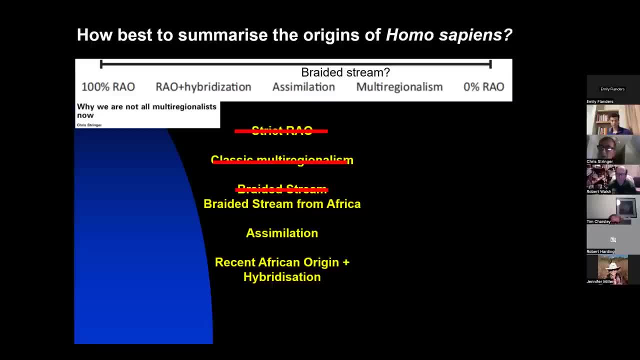 there's little sign of it going the other way, other way, other way. those populations are not assimilating. those populations are not assimilating. those populations are not assimilating homo sapiens genes, homo sapiens genes, homo sapiens genes- in gene flow and transforming into 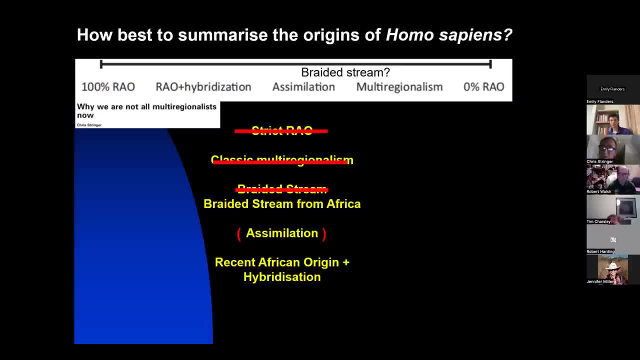 in gene flow and transforming into: in gene flow and transforming into homo sapiens populations in situ, homo sapiens populations in situ, homo sapiens populations in situ. so i would say assimilation is less likely. so i would say assimilation is less likely. so i would say assimilation is less likely. as a model: uh and recent african origin. 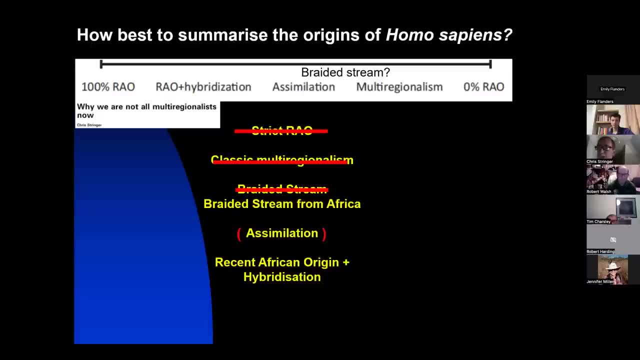 as a model uh and recent african origin. as a model uh and recent african origin, hybridization is the most likely one. hybridization is the most likely one. hybridization is the most likely one. but if you don't want all these labels, but if you don't want all these labels, 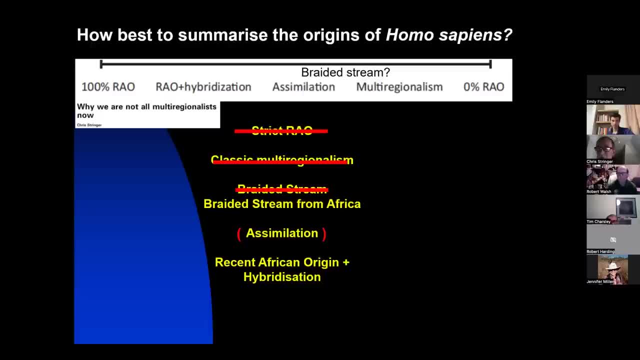 but if you don't want all these labels, then i would say we can follow the. then i would say we can follow the. then i would say we can follow the recent nobel prize winners: fantipabo. recent nobel prize winners: fantipabo. recent nobel prize winners: fantipabo- and just say that we are mostly out of. 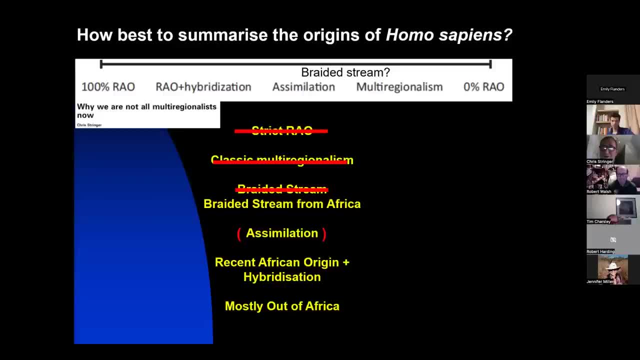 and just say that we are mostly out of, and just say that we are mostly out of africa, and, uh, that certainly will do for africa. and, uh, that certainly will do for africa. and, uh, that certainly will do for me as a summary of the situation, me as a summary of the situation. 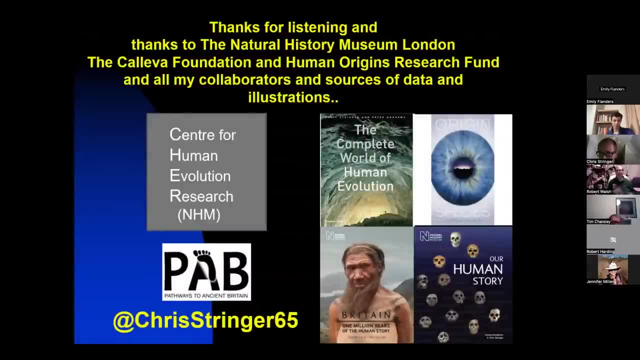 me as a summary of the situation. so i'll stop there. thank you very much, so i'll stop there. thank you very much, so i'll stop there. thank you very much. yeah, thank you for that. yeah, thank you for that. yeah, thank you for that. yeah, so should i stop screen sharing, or? 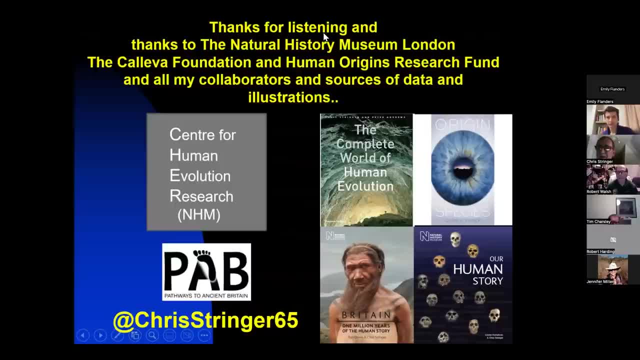 yeah, so should i stop screen sharing? or yeah, so should i stop screen sharing, or should i leave that slide up? should i leave that slide up? should i leave that slide up? um, um, um, uh. either you can leave it up, if you okay, uh, either you can leave it up, if you okay. 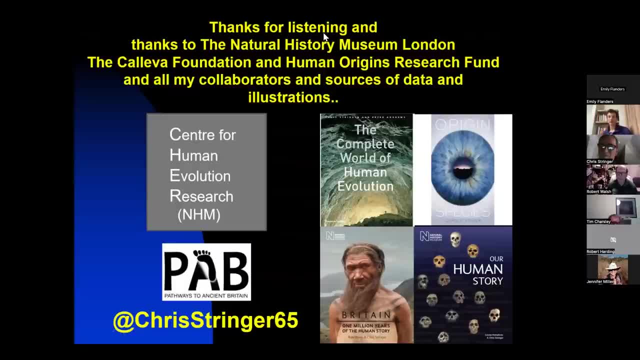 uh, either you can leave it up, if you okay, i'll leave it up to you, okay. yeah, fine, i'll leave it up to you, okay. yeah fine, i'll leave it up to you, okay. yeah, fine, thanks, thanks, thanks. so if anybody has questions, uh, feel free. 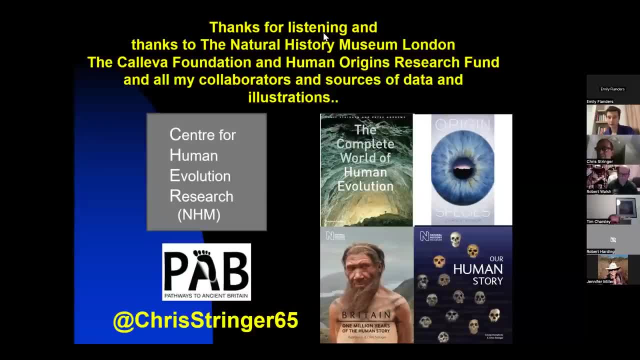 so if anybody has questions, uh feel free. so if anybody has questions, uh feel free to either to either to either use the raise hand function, uh, or to use the raise hand function uh, or to use the raise hand function uh, or to- to put it in the chat and i'll read it: 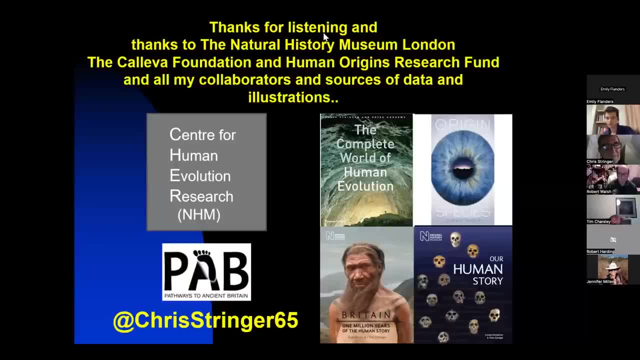 to put it in the chat and i'll read it. to put it in the chat and i'll read it out. i guess well people think of their, their. i guess well people think of their, their. i guess well people think of their, their questions, i i can start out with one. 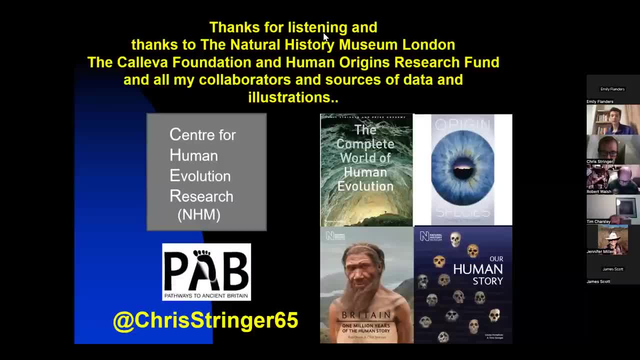 questions: i i can start out with one questions. i i can start out with one. okay, okay, okay, uh, uh, uh. obviously you, obviously, you, obviously you played a large part in um, played a large part in um, played a large part in um. shaping the, the, shaping the, the. 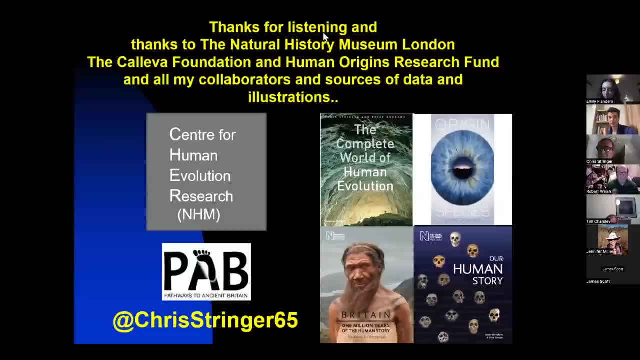 shaping the the main, the mainstream out of africa theory, main the mainstream out of africa theory, main the mainstream out of africa theory. uh, that has been like dominant over the uh. that has been like dominant over the uh. that has been like dominant over the past few decades. uh versus the the. 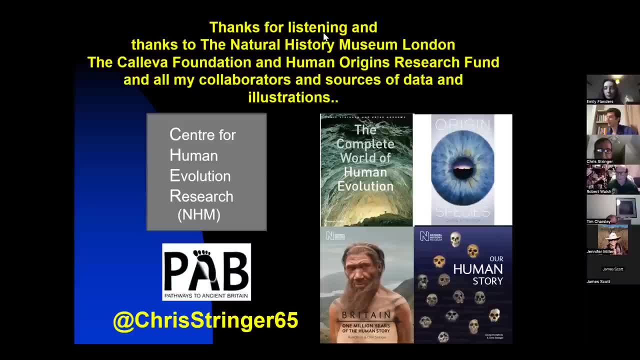 past few decades, uh versus the, the past few decades, uh versus the, the multi-regional hypothesis, and you briefly multi-regional hypothesis and you briefly multi-regional hypothesis and you briefly mentioned um, mentioned um, mentioned um, the, the pan african model, the, the pan african model. 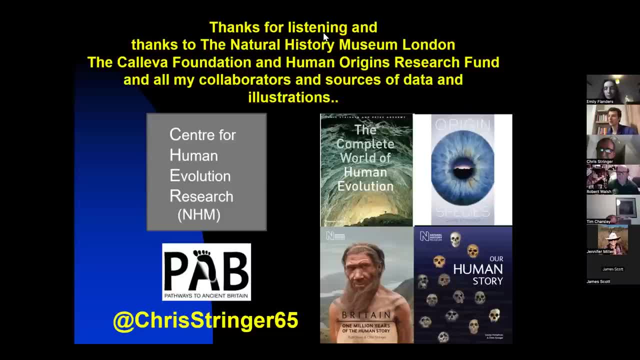 the, the pan african model, um um, um, and i was just wondering what, and i was just wondering what, and i was just wondering what, uh, uh, and i was just wondering what, what evidence do you think there would? what evidence do you think there would? what evidence do you think there would need to be? 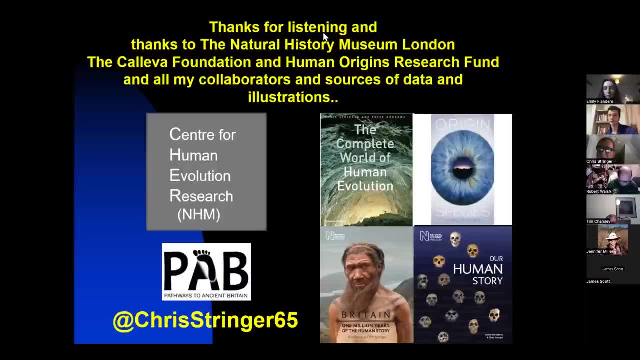 need to be, need to be to um support the pan-african versus to um support the pan-african versus to um support the pan-african versus the. the current model, the, the current model, the, the current model, um, and like what we would need to do in. 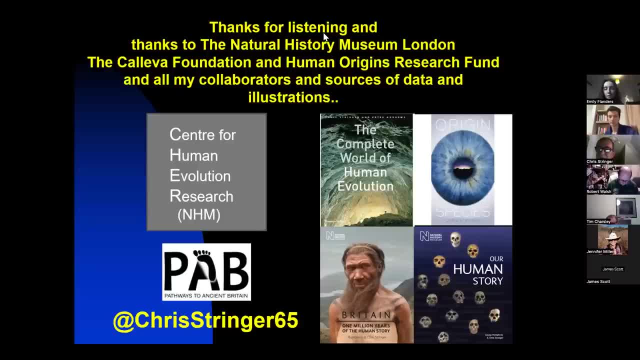 um, and like what we would need to do in um, and like what we would need to do in order to obtain that evidence. order to obtain that evidence. order to obtain that evidence. yes, so i think that obviously i alluded. yes, so i think that obviously i alluded. 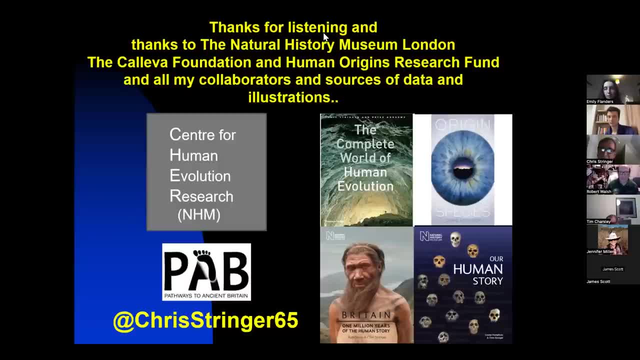 yes, so i think that obviously i alluded to the fact that some of the fossil, to the fact that some of the fossil, to the fact that some of the fossil record is not well dated, so i think that record is not well dated. so i think that obviously i alluded to the fact that 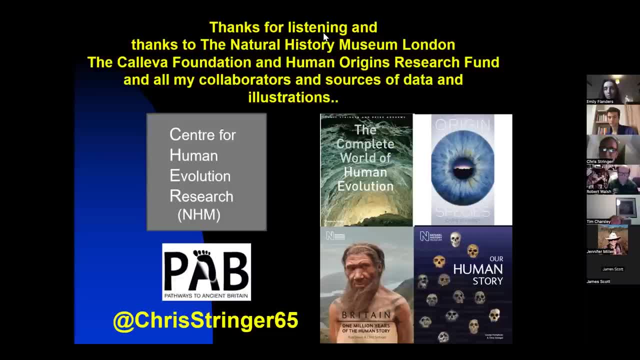 record is not well dated. so i think that obviously i alluded to the fact that having having having obviously a better dated record for africa, obviously a better dated record for africa, obviously a better dated record for africa, is going to help us really see, is going to help us really see. 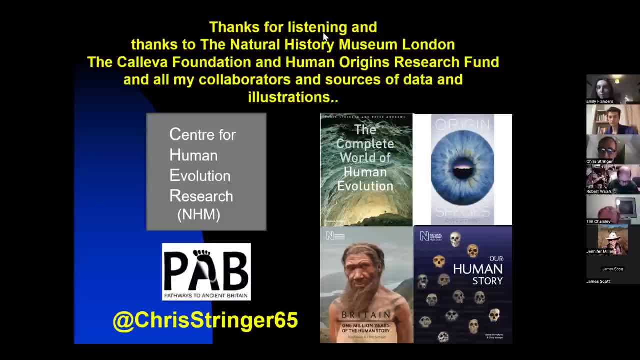 is going to help us really see which areas if you like were were, which areas if you like were were, which areas if you like were were dominant, dominant, dominant, even within africa, in terms of the even within africa, in terms of the even within africa in terms of the evolution of these homo sapiens. 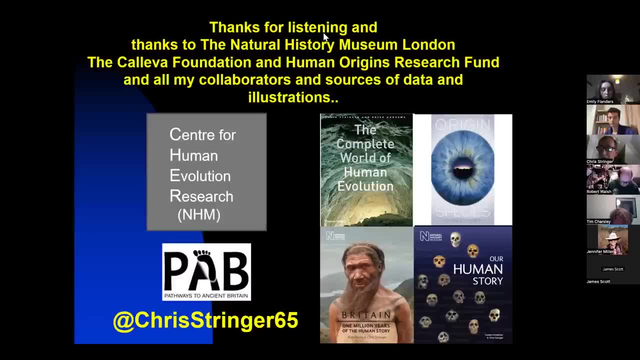 evolution of these homo sapiens. evolution of these homo sapiens: features so features, so features. so you know which area of africa has the. you know which area of africa has the. you know which area of africa has the appearance of a globular cranial vault. appearance of a globular cranial vault. 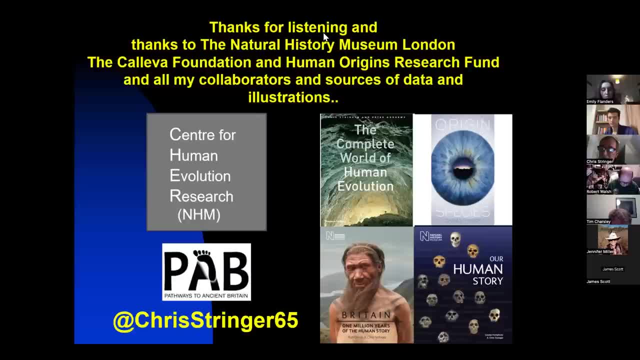 appearance of a globular cranial vault for the first time. which area has the? for the first time, which area has the? for the first time, which area has the reduction of the brow ridge down to the reduction of the brow ridge, down to the reduction of the brow ridge, down to the, the recent homo sapiens pattern, which 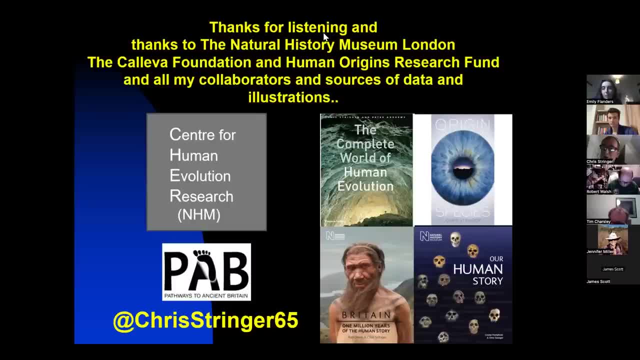 the recent homo sapiens pattern. which the recent homo sapiens pattern? which area shows the clear evolution of a chin area? shows the clear evolution of a chin area. shows the clear evolution of a chin. which area shows the earliest devolution? which area shows the earliest devolution? 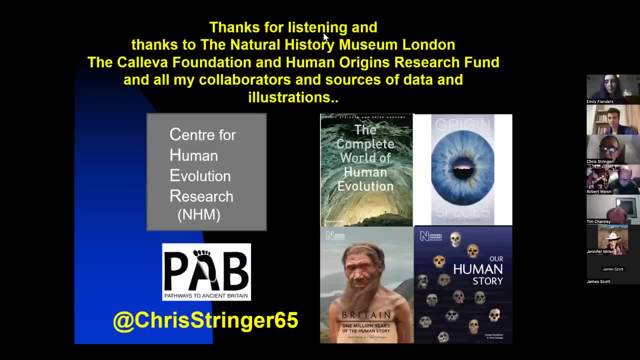 which area shows the earliest devolution of that, of that, of that homo sapiens pelvic morphology, so homo sapiens pelvic morphology, so homo sapiens pelvic morphology. so i think, as we get a better picture for i think, as we get a better picture for i think, as we get a better picture for africa, we will, we will build a more. 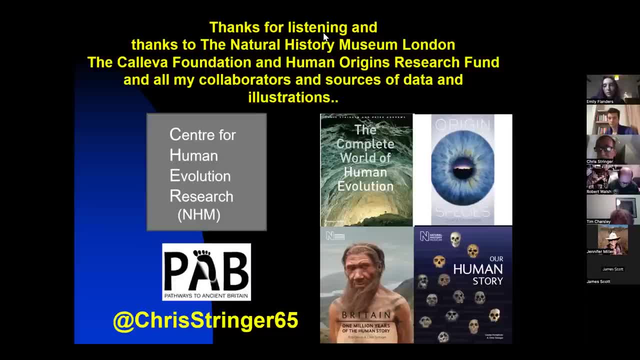 africa. we will, we will build a more africa. we will, we will build a more complete scenario of how we evolve there, complete scenario of how we evolve there, complete scenario of how we evolve there. but the problem is, i didn't get a chance. but the problem is i didn't get a chance. 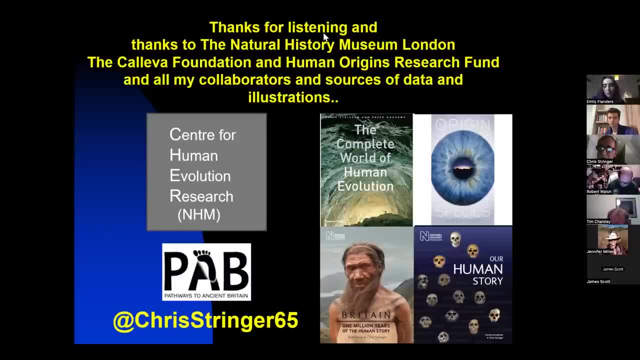 but the problem is, i didn't get a chance to say it, but of course to say it, but of course to say it, but of course, even now, our african evidence comes from. even now our african evidence comes from. even now, our african evidence comes from only a very small part of the whole. 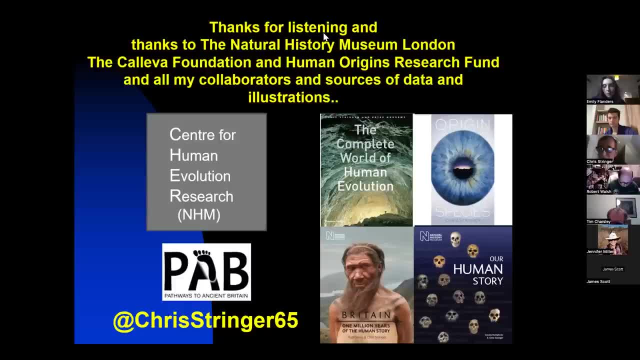 only a very small part of the whole, only a very small part of the whole continent, continent, continent. um you know, i often say it's that more um you know, i often say it's that more um you know, i often say it's that more than 90 percent of the african continent. 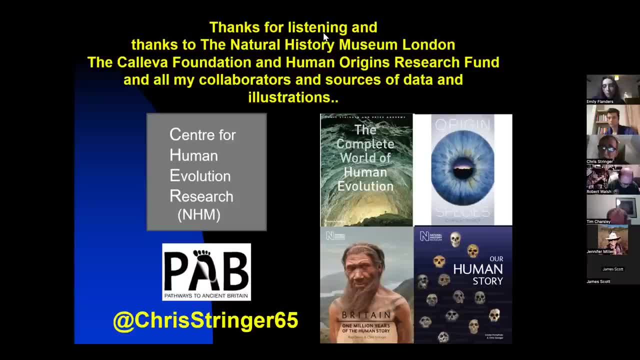 than 90 percent of the african continent, than 90 percent of the african continent has produced no significant fossil, has produced no significant fossil, has produced no significant fossil. evidence, evidence, evidence for the time period i'm talking about. so, for the time period i'm talking about so. 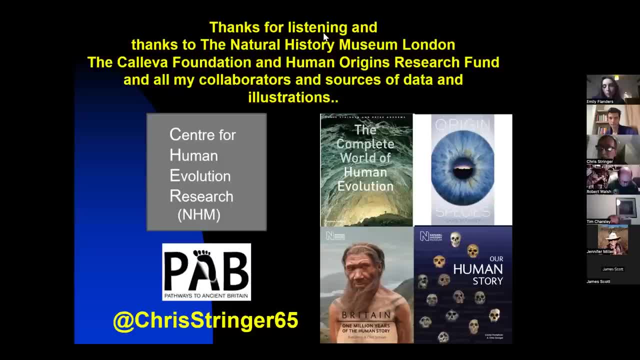 for the time period i'm talking about so huge areas of huge areas of huge areas of of central and western africa. um, we know of central and western africa. um, we know of central and western africa, um, we know people were there from archaeology. people were there from archaeology. 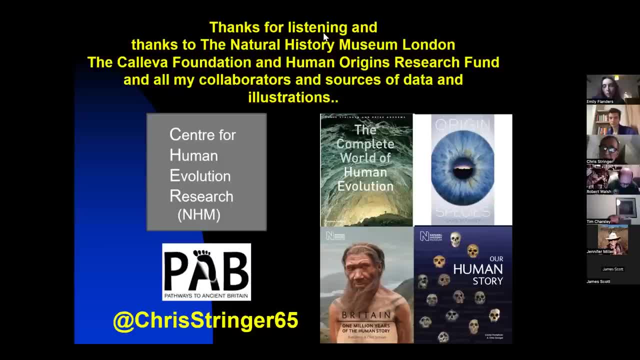 people were there from archaeology, but we don't know anything about what. but we don't know anything about what, but we don't know anything about what they look like. they look like. they look like you've got these wonderful sedimentary. you've got these wonderful sedimentary. 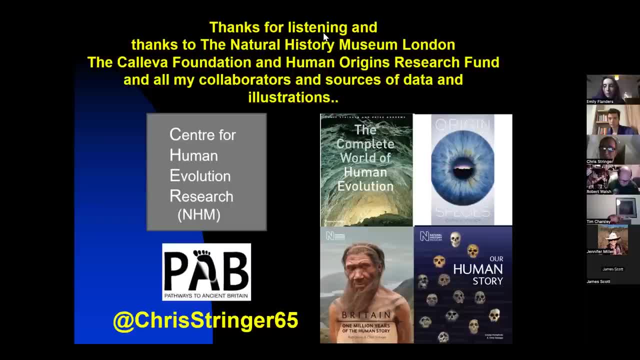 you've got these wonderful sedimentary basins which preserve the fossils basins, which preserve the fossils basins, which preserve the fossils, and so of course it's easy to build up, and so of course it's easy to build up, and so of course it's easy to build up a picture of. 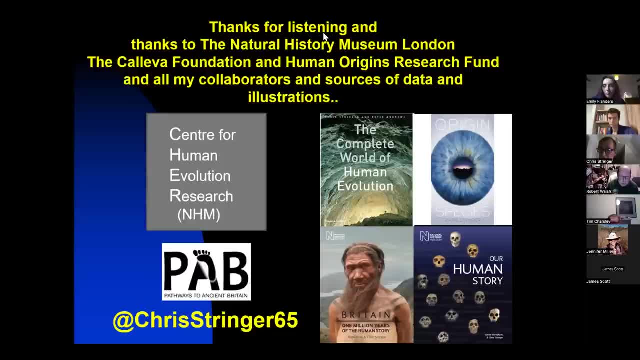 a picture of a picture of of homo sapiens, evolution from that of homo sapiens, evolution from that of homo sapiens, evolution from that evidence because it's evidence, because it's evidence, because it's, in many ways it was pretty much most of, in many ways it was pretty much most of. 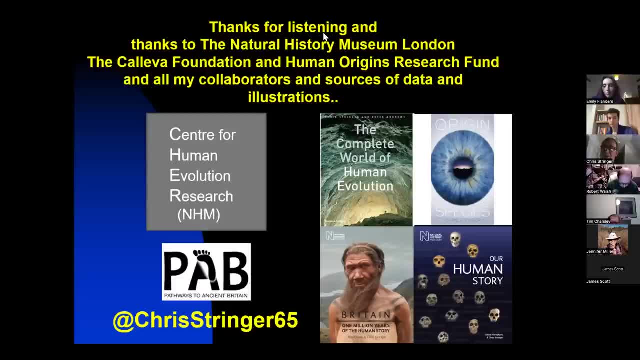 in many ways it was pretty much most of the evidence we had, the evidence we had, the evidence we had, but, as people said, it's often the but as people said, it's often the but, as people said, it's often the analogy about the- uh, the guy who's lost. 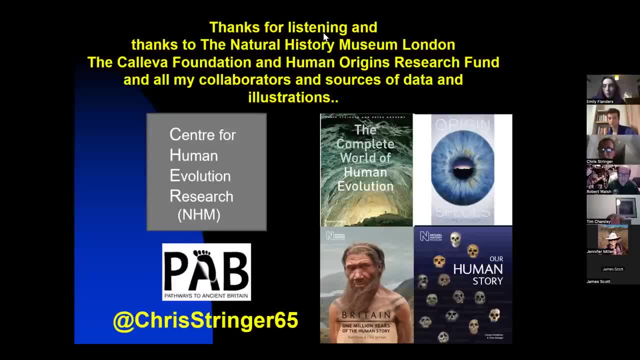 analogy about the. uh, the guy who's lost. analogy about the. uh, the guy who's lost his car keys, his car keys, his car keys, um, and so uh, he's he's looking around um, and so uh, he's he's looking around um, and so uh he's he's looking around under the street light for his car keys. 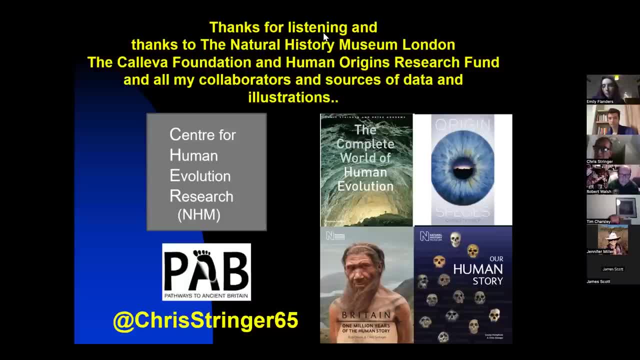 under the street light for his car keys, under the street light for his car keys, because that's where the light is, but because that's where the light is, but because that's where the light is. but actually his car keys are a bit further. actually his car keys are a bit further. 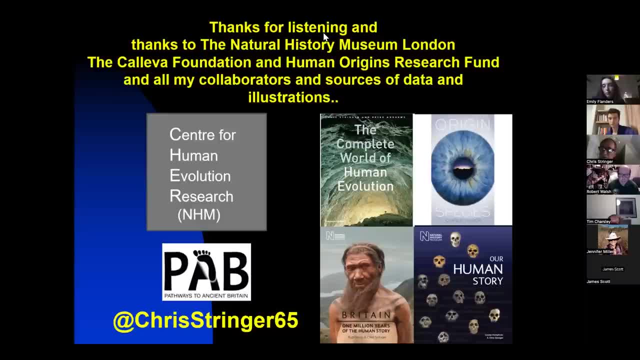 actually, his car keys are a bit further away, where it's dark, and so he isn't away where it's dark, and so he isn't away where it's dark, and so he isn't going to find them. and so it's a bit going to find them, and so it's a bit. 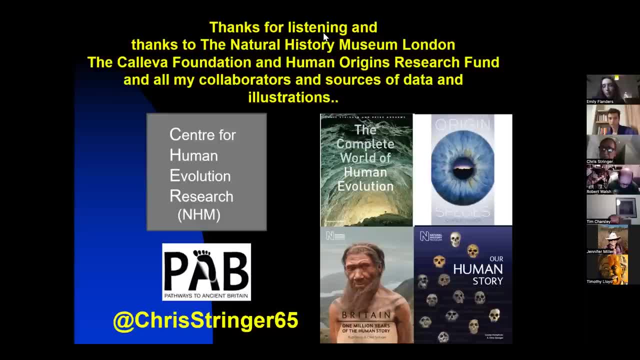 going to find them, and so it's a bit like that with with the african fossil, like that with with the african fossil, like that with with the african fossil record. that we record that we record that we, we obviously have a i i'm very. we obviously have a i i'm very. 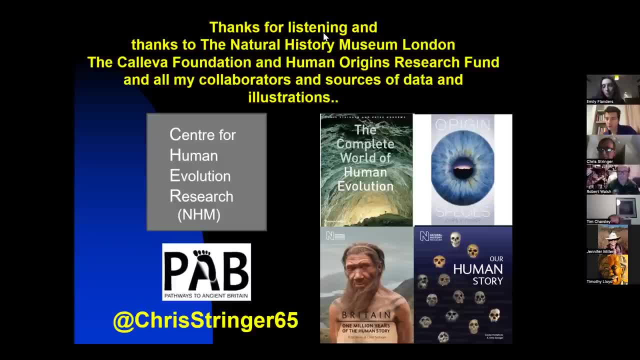 we obviously have a: i i'm very stimulated, but stimulated, but stimulated, but string at all, string at all, string at all, your your microphone, so yeah, so that's really just to say so. yeah, so that's really just to say so. yeah, so that's really just to say that. you know, i think that we will you. that you know. i think that we will. you that you know, i think that we will. you know it's too early to say for sure that know. it's too early to say for sure that know. it's too early to say for sure that it's a pan-african pattern. and 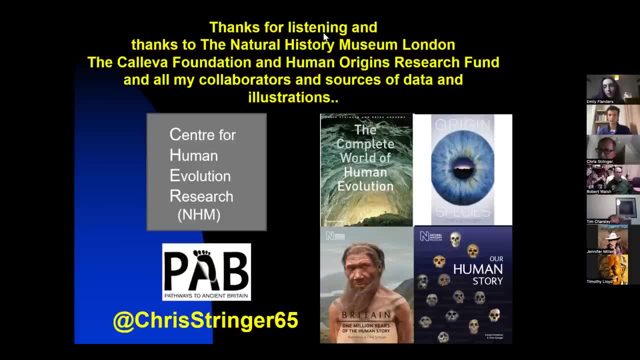 it's a pan-african pattern, and it's a pan-african pattern and that's why i said that it isn't. that's why i said that it isn't, that's why i said that it isn't necessarily the entire african continent, necessarily the entire african continent. 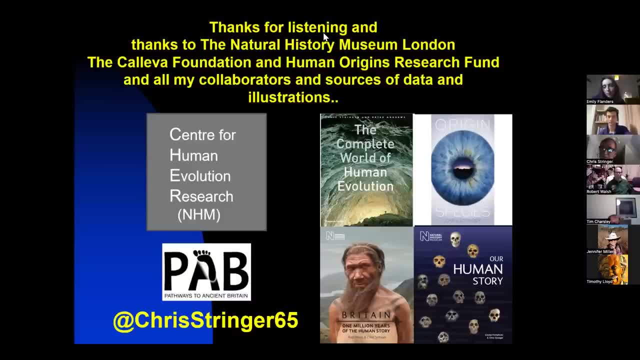 necessarily the entire african continent. that's contributing to the evolution of, that's contributing to the evolution of, that's contributing to the evolution of homo sapiens, homo sapiens, homo sapiens. but i think that it certainly will be, but i think that it certainly will be. 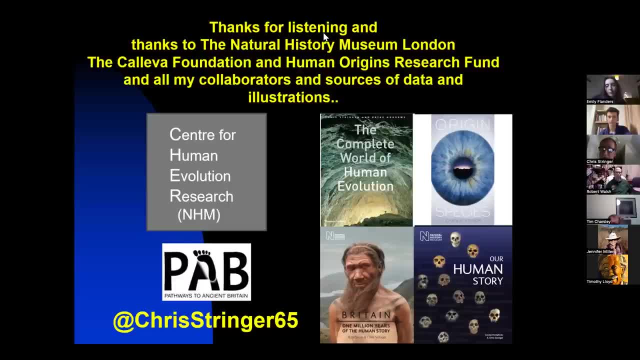 but i think that it certainly will be more than one small area and obviously more than one small area and obviously more than one small area. and obviously, genetic data hopefully will come through. genetic data hopefully will come through. genetic data, hopefully will come through to also support this idea of a 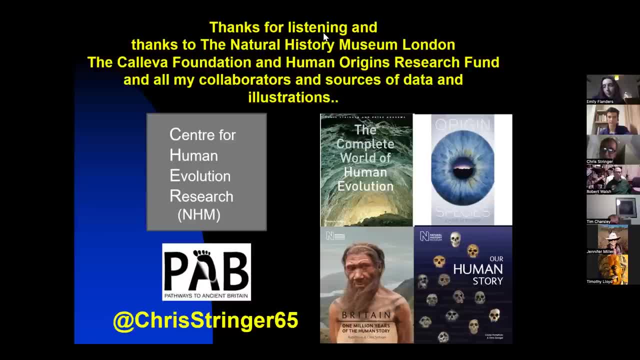 to also support this idea of a, to also support this idea of a pan-african uh model, that i think that pan-african uh model, that i think that pan-african uh model, that i think that, and culturally, in terms of you know the, and culturally, in terms of you know the. 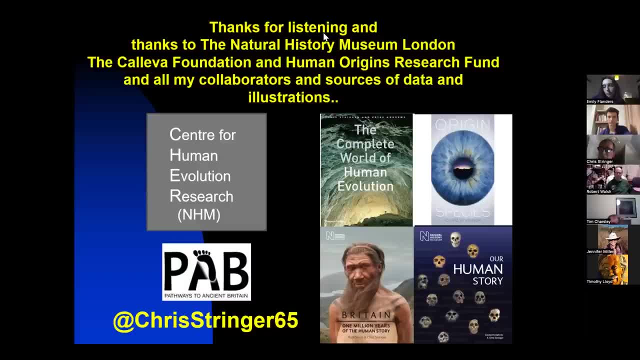 and culturally in terms of you know the archaeology also, i think supports this archaeology also. i think supports this archaeology also. i think supports this idea that there isn't just one place idea that there isn't just one place idea that there isn't just one place where modern human behavior, as we call. 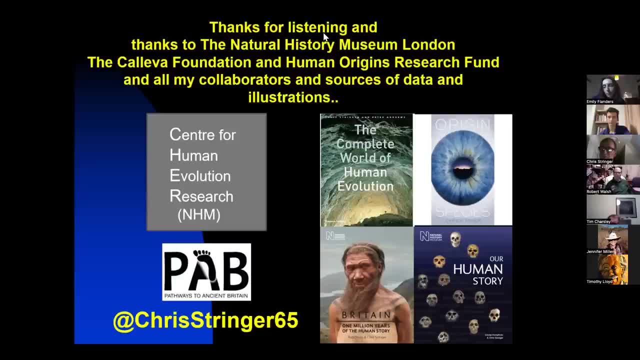 where modern human behavior, as we call, where modern human behavior, as we call it, emerged, it's emerging in a number of it emerged. it's emerging in a number of it emerged. it's emerging in a number of different places, different places, different places. yeah, thank you. yeah, that's quite. 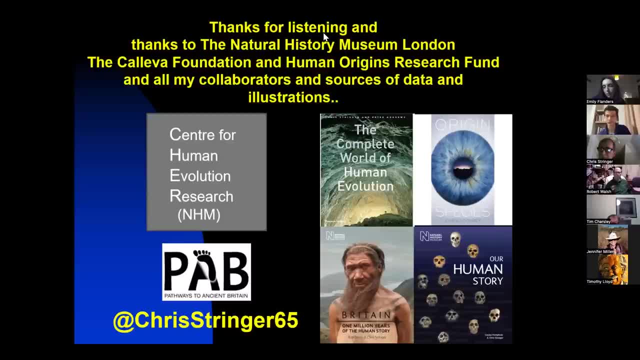 yeah, thank you. yeah, that's quite. yeah, thank you. yeah, that's quite interesting. i guess, yeah, we, we can't interesting. i guess, yeah, we, we can't interesting. i guess, yeah, we, we can't know until we we look know, until we we look know, until we we look um. 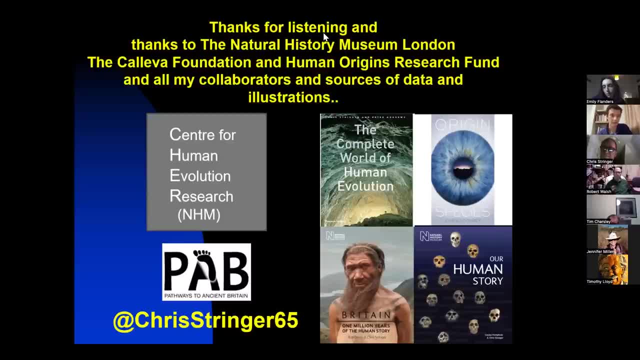 um, um and then and then and then. there's a number of questions that have. there's a number of questions that have. there's a number of questions that have come in through the chat, so i don't know. come in through the chat, so i don't know. 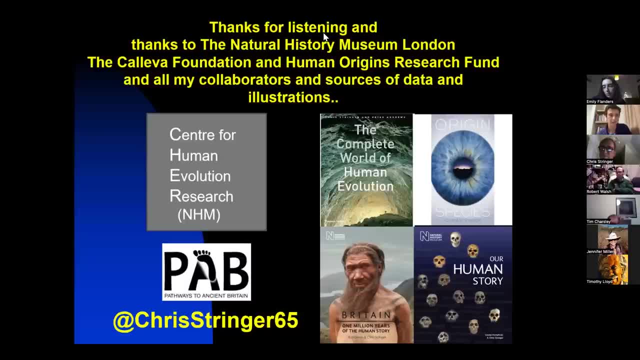 come in through the chat. so i don't know if um, if um, if um, they want to be asked out loud, so tim. they want to be asked out loud, so tim. they want to be asked out loud, so tim. charles lee, do you want to? charles lee, do you want to? 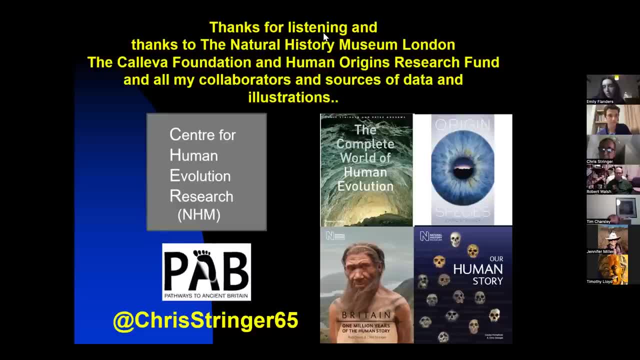 charles lee, do you want to read yours out, or should i read yours out? or should i read yours out, or should i? i'll read out um. so tim is wondering. i'll read out um. so tim is wondering. i'll read out um. so tim is wondering why there is no gene flow back into. 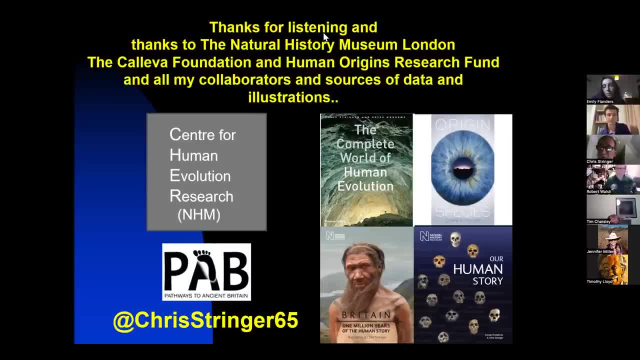 why there is no gene flow back into, why there is no gene flow back into africa, africa, africa. yeah, i mean there is some gene flow back. yeah, i mean there is some gene flow back. yeah, i mean there is some gene flow back into africa. and that's why i mean. 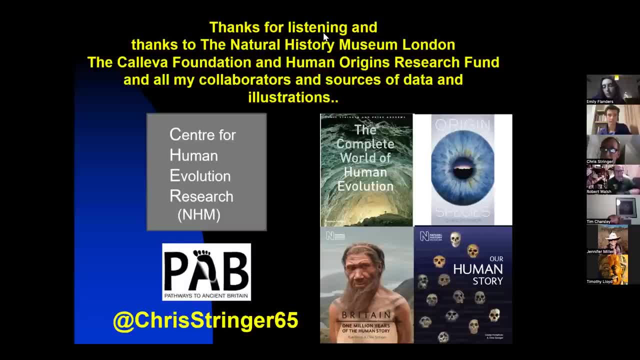 into africa, and that's why i mean into africa, and that's why i mean african populations. today have got african populations. today have got african populations today have got neanderthal dna and certainly a lot of neanderthal dna and certainly a lot of neanderthal dna and certainly a lot of it has come in. 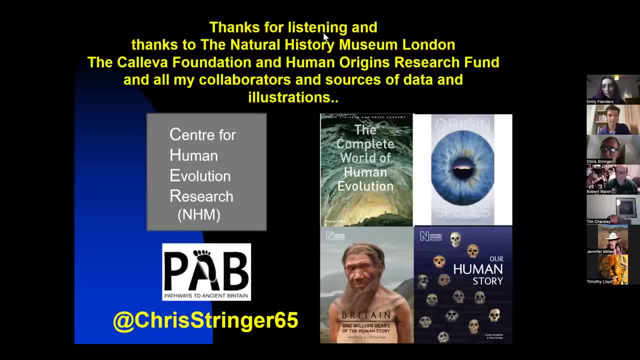 it has come in. it has come in in historic times. so obviously the in historic times, so obviously the in historic times. so obviously the spread of the roman empire around the spread of the roman empire around the spread of the roman empire around the mediterranean took neanderthal dna into. 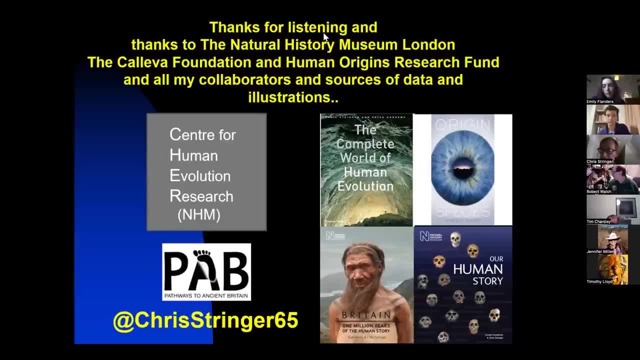 mediterranean took neanderthal dna into mediterranean. took neanderthal dna into africa, africa, africa. the spread of islam has has taken. the spread of islam has has taken. the spread of islam has has taken neanderthal dna into africa. 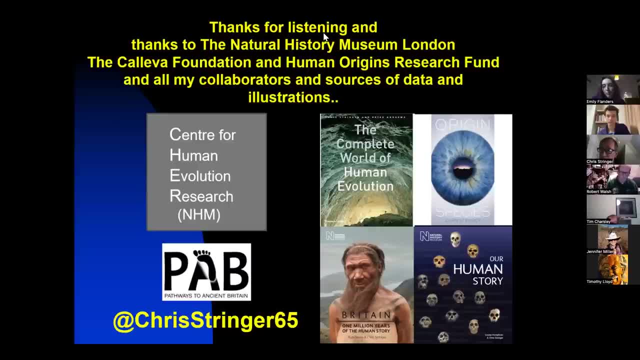 neanderthal dna into africa. neanderthal dna into africa. trading networks around the trading networks around the trading networks around the indian ocean. took neanderthal dna from indian ocean. took neanderthal dna from indian ocean. took neanderthal dna from. there's no reason why, even in ancient, 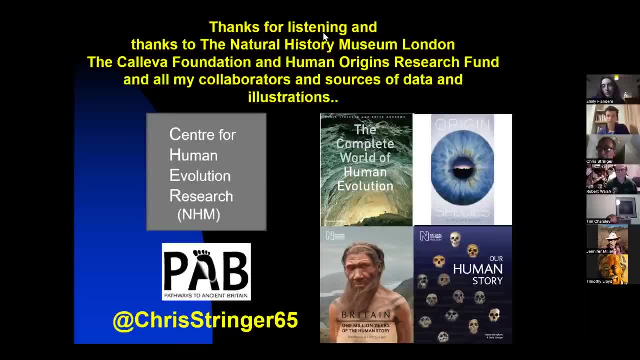 there's no reason why, even in ancient, there's no reason why even in ancient times, populations couldn't have been. you times populations couldn't have been, you times populations couldn't have been. you know there was no barrier that stopped. know there was no barrier that stopped. 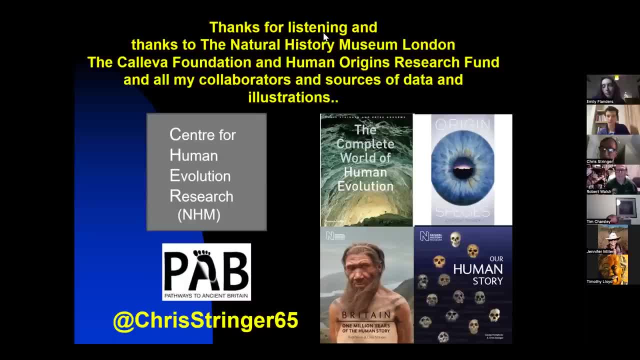 know there was no barrier that stopped people coming into africa, people coming into africa, people coming into africa- and i've speculated before that. you know and i've speculated before that. you know and i've speculated before that you know neanderthals, we know from neanderthals, we know from. 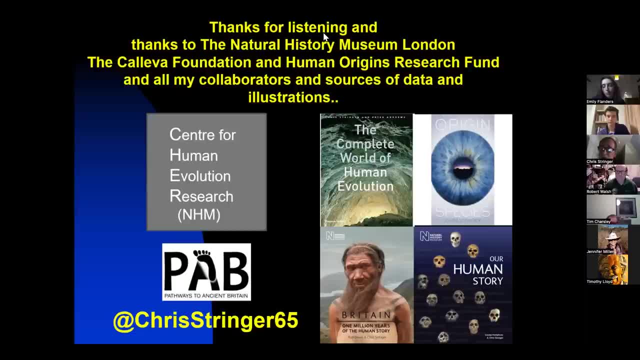 neanderthals. we know from the shukpa site uh in southern israel. the shukpa site uh in southern israel, the shukpa site uh in southern israel. shukpa is only a few hundred kilometers. shukpa is only a few hundred kilometers. 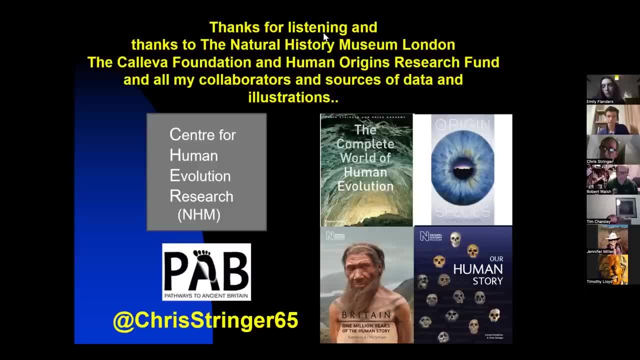 shukpa is only a few hundred kilometers from cairo. so if neanderthals got that from cairo, so if neanderthals got that from cairo, so if neanderthals got that far south, far south, far south, um, i don't see any reason why at times 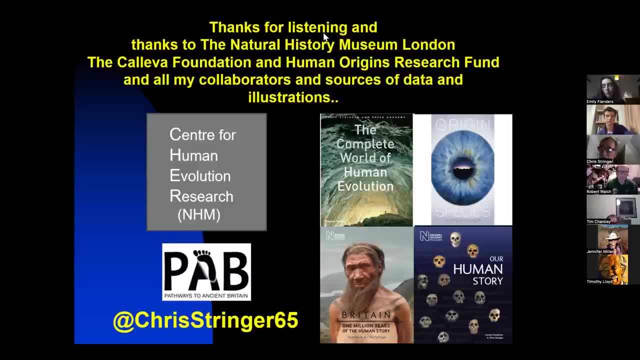 um, i don't see any reason why, at times, um, i don't see any reason why, at times, even they couldn't have penetrated into, even they couldn't have penetrated into, even they couldn't have penetrated into africa at times, africa at times, africa at times. so, um, you know, i think that's a. 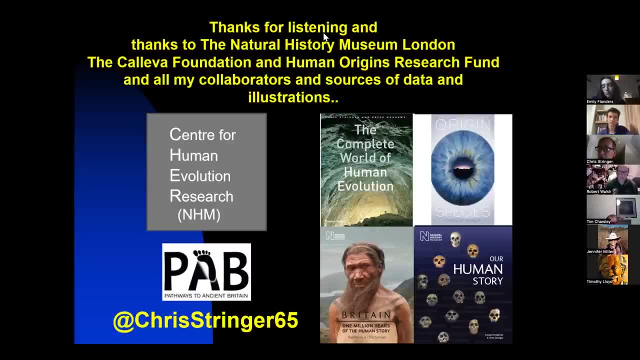 so um, you know, i think that's a so um, you know, i think that's a possibility, and, as i said, for possibility, and as i said for possibility, and as i said, for the origin of the homo sapiens, the origin of the homo sapiens, the origin of the homo sapiens lineage, um. 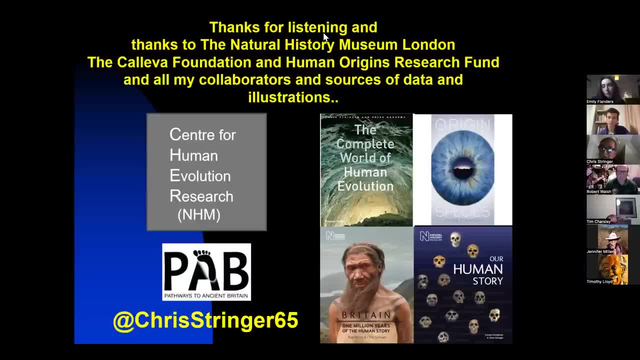 the origin of the homo sapiens lineage um and the neanderthal lineage? we don't. and the neanderthal lineage: we don't. and the neanderthal lineage, we don't even know, even know, even know where that common ancestor lived of us, where that common ancestor lived of us. where that common ancestor lived, of us and neanderthals and denisovans, and neanderthals and denisovans, and neanderthals and denisovans. it could have been an african origin, as it could have been an african origin as. 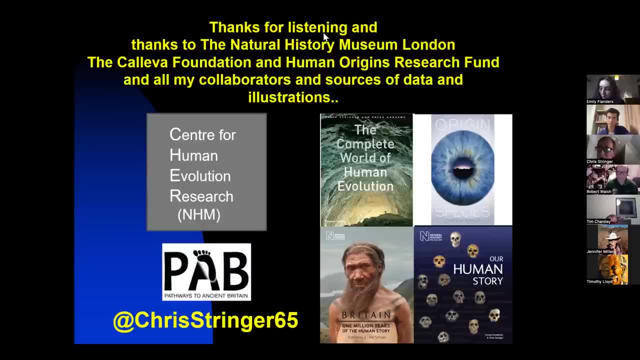 it could have been an african origin, as many people have suggested, many people have suggested, many people have suggested. but equally it could have been an asian. but equally, it could have been an asian, but equally it could have been an asian origin. it could have been even a. 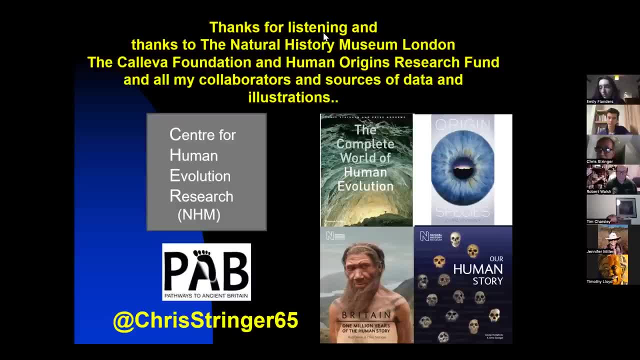 origin. it could have been even a origin. it could have been even a european origin. so yeah, european origin. so yeah, european origin. so yeah, i'm not saying it's all africa, um, and i'm not saying it's all africa, um, and i'm not saying it's all africa, um, and there could be. 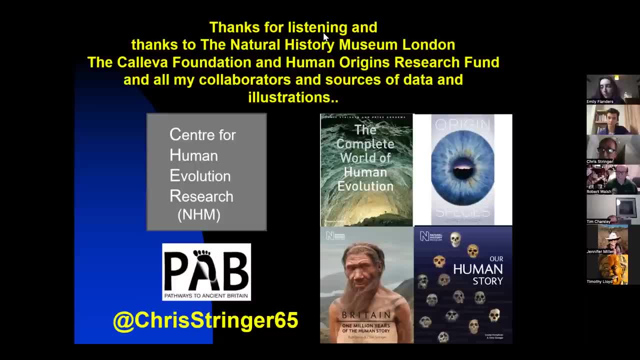 there could be. there could be into africa events as well as out of into africa events as well as out of into africa events as well as out of africa events. of course, yeah, africa events, of course yeah. africa events. of course yeah. and hillary and hillary. 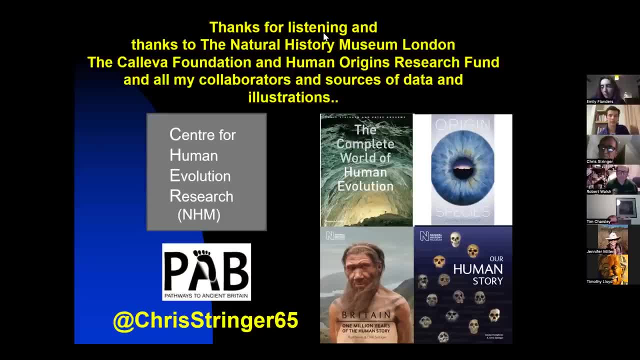 and hillary. uh is asking: what do we know about? uh is asking: what do we know about? uh is asking: what do we know about population numbers over time? population numbers over time. population numbers over time. did homo sapiens simply outnumber? did homo sapiens simply outnumber? 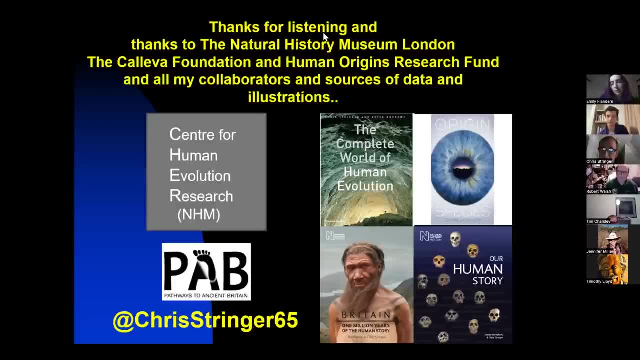 did homo sapiens simply outnumber neanderthals, for example, neanderthals, for example, neanderthals, for example, uh population numbers at times were uh population numbers, at times were uh. population numbers at times were very low, so very low, so very low. so we know neanderthals near the end of 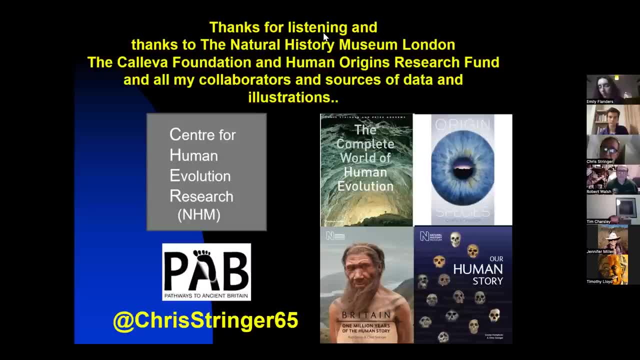 we know neanderthals near the end of. we know neanderthals near the end of their time, were their time, were their time. were. were low in diversity compared with. were low in diversity compared with. were low in diversity compared with homo sapiens- homo sapiens. homo sapiens lower than denisovans, apparently in lower than denisovans, apparently in lower than denisovans, apparently in terms of diversity, terms of diversity, terms of diversity. so they were low in numbers, um, we could. so they were low in numbers, um, we could. 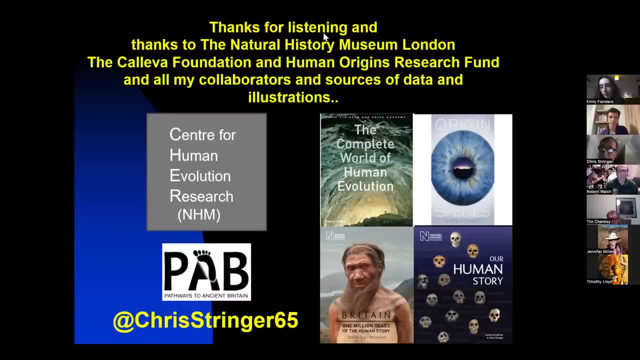 so they were low in numbers. um, we could be talking just thousands of people. be talking just thousands of people. be talking just thousands of people. population size and population density. population size and population density. population size and population density. comparing late neanderthal sites and comparing late neanderthal sites. and. 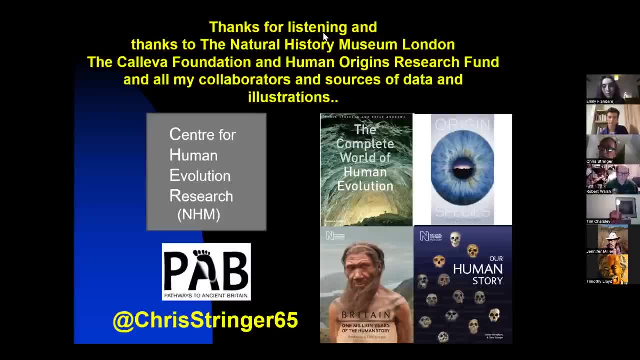 comparing late neanderthal sites and early homo sapiens sites in uh, in early homo sapiens sites in uh, in early homo sapiens sites in uh, in france, and france and france. and that paper which the conclusions have, that paper which the conclusions have, that paper which the conclusions have been questioned strongly since. but 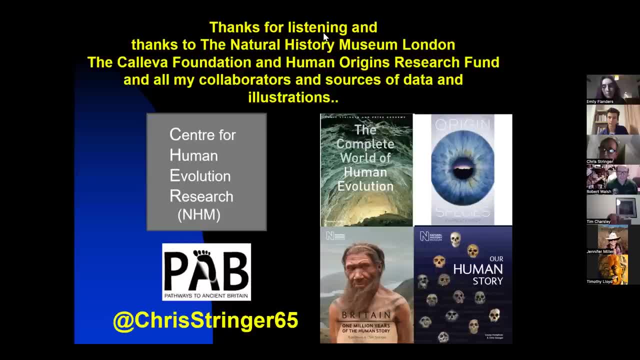 been questioned strongly since. but been questioned strongly since. but there was a suggestion there that some. there was a suggestion there that some. there was a suggestion there that some of those homo sapiens occupations of those homo sapiens occupations of those homo sapiens occupations had 10 times the number of people. uh. 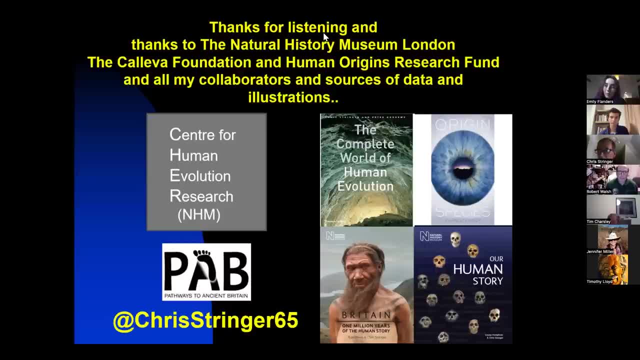 had 10 times the number of people. uh, had 10 times the number of people. uh, that the late neanderthal occupations, that the late neanderthal occupations, that the late neanderthal occupations had had had. but i know that work has been subject to. 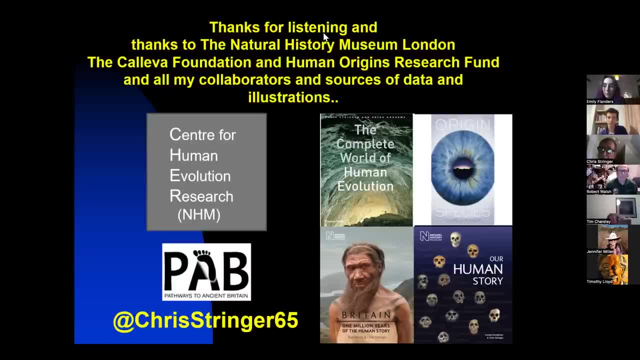 but i know that work has been subject to. but i know that work has been subject to: uh, it's a discussion afterwards, so i uh it's a discussion afterwards. so i uh it's a discussion afterwards. so i don't know if it's uh, if it's correct. 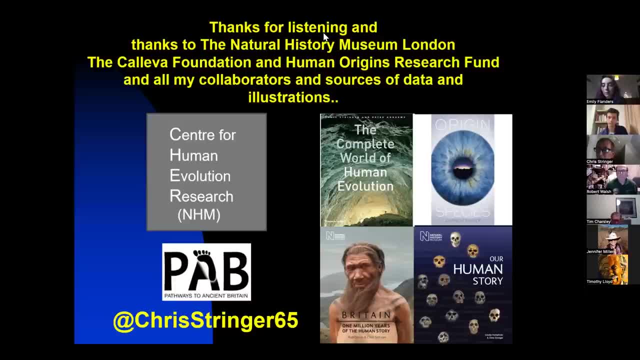 don't know if it's uh, if it's correct. don't know if it's uh, if it's correct, but certainly evidence that homo sapiens, but certainly evidence that homo sapiens. but certainly evidence that homo sapiens. numbers did grow quite quickly, numbers did grow quite quickly. 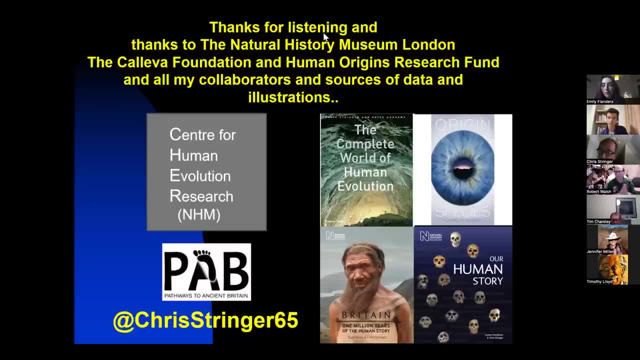 numbers did grow quite quickly: um after 40 000 years ago, um after 40 000 years ago, um after 40 000 years ago, but then they may have crashed because, but then they may have crashed because, but then they may have crashed because, when we get to something like the last, 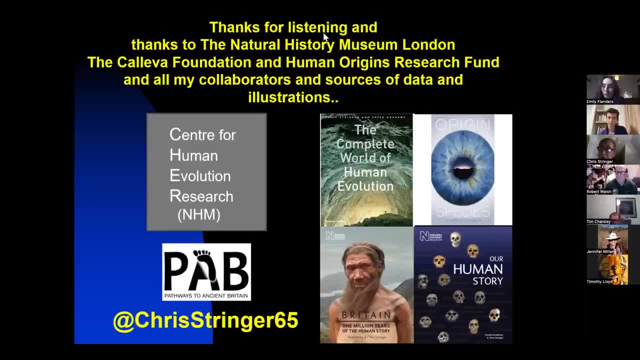 when we get to something like the last, when we get to something like the last glacial maximum- it looks like that did glacial maximum. it looks like that did glacial maximum. it looks like that did have quite a severe bottlenecking effect, have quite a severe bottlenecking effect. 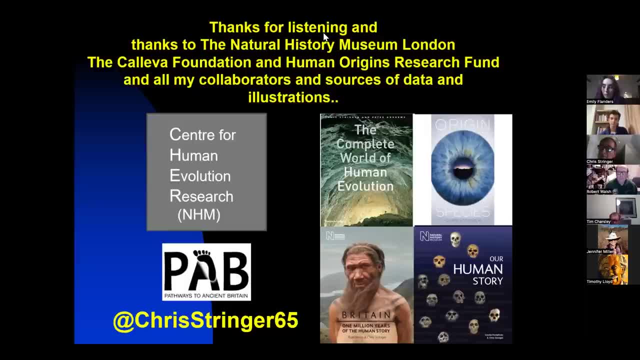 have quite a severe bottlenecking effect on the homo sapiens populations and on the homo sapiens populations and on the homo sapiens populations and they may have shrunk down in number at they may have shrunk down in number, at they may have shrunk down in number at that time. 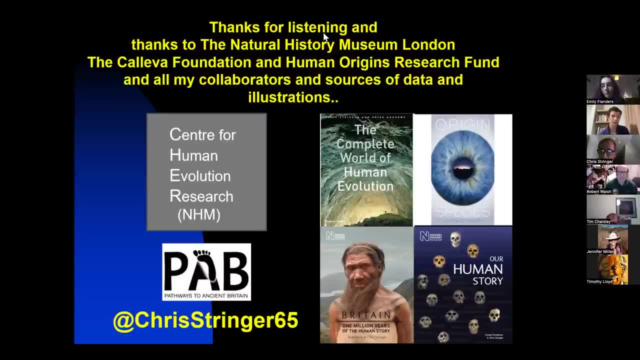 and bratislav uh has, and bratislav uh has, and bratislav uh has, quite a big question which is, uh, what is quite a big question, which is, uh, what is quite a big question, which is, uh, what is the first and most significant change in? 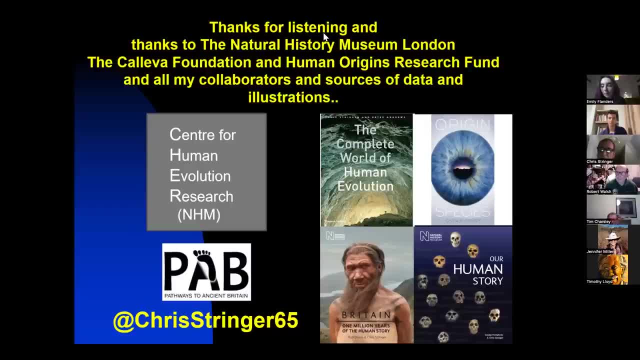 the first and most significant change in the first and most significant change in bipedalism is is one big change and we bipedalism is is one big change and we bipedalism is is one big change and we don't know, don't know. 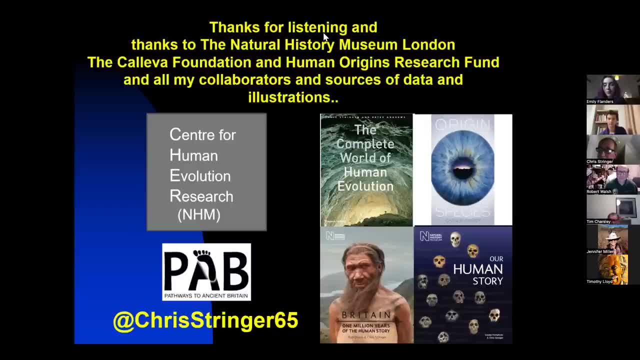 don't know for sure when that originated and for sure when that originated and for sure when that originated, and perhaps it even had. perhaps it even had, perhaps it even had independent origins in different independent origins, in different independent origins in different lineages. so we don't even know if there 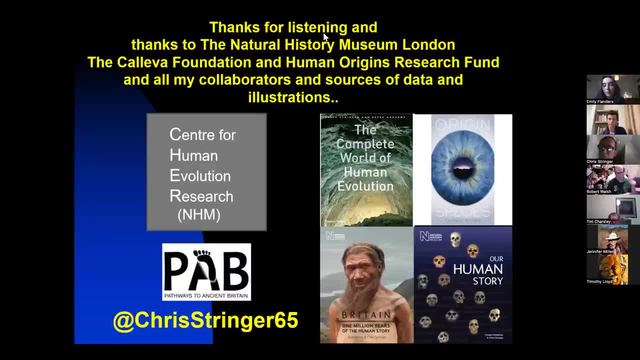 lineages, so we don't even know if there lineages. so we don't even know if there was a single origin for bipedalism. or it was a single origin for bipedalism, or it was a single origin for bipedalism or it actually evolved. you know independently. 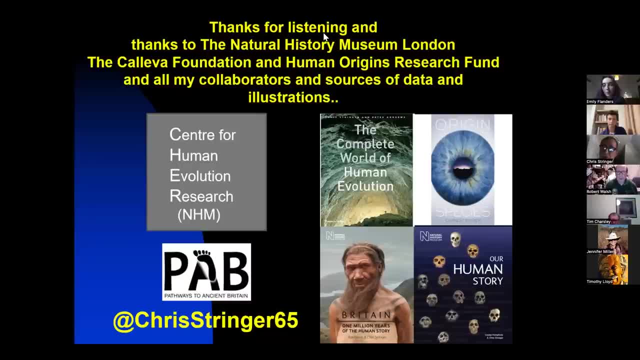 actually evolved, you know independently actually evolved, you know independently, in different lineages. so i think in different lineages. so i think in different lineages. so i think bipedism was a major change. bipedism was a major change. bipedism was a major change. but if you've looked at the discussions, 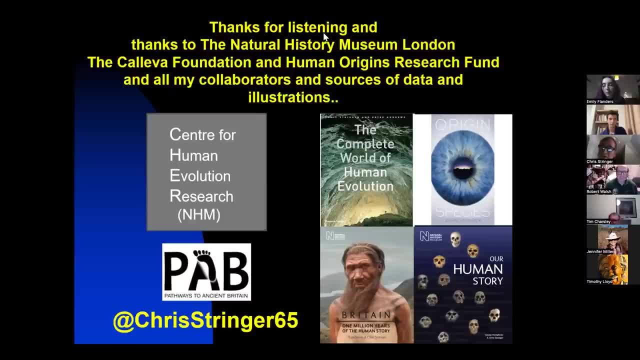 but if you've looked at the discussions, but if you've looked at the discussions around the sarholanthropus material, so around the sarholanthropus material, so around the sarholanthropus material, so you've got there, you've got there. 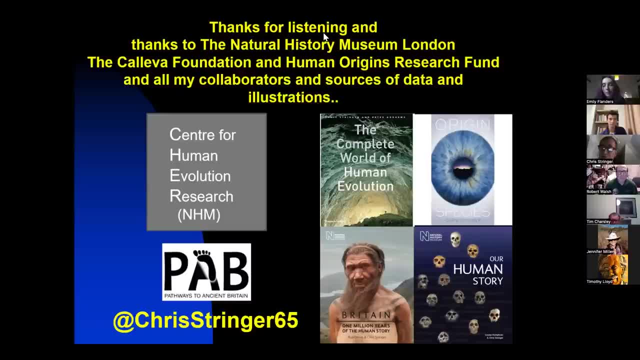 you've got there. uh, you know a femur of sarholanthropus. uh, you know a femur of sarholanthropus. uh, you know a femur of sarholanthropus. and one group of people have looked at, and one group of people have looked at. 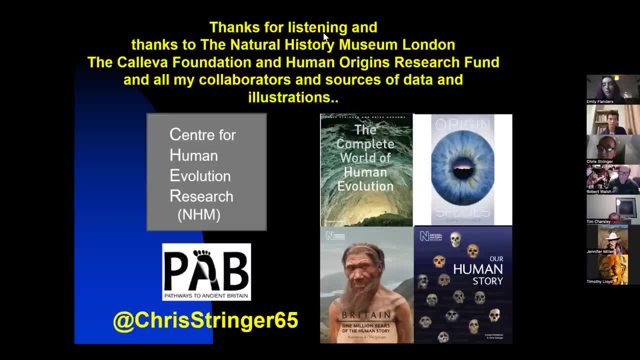 and one group of people have looked at it and concluded that it's not a biped. it and concluded that it's not a biped. it and concluded that it's not a biped. another group of people looked at it. another group of people looked at it. 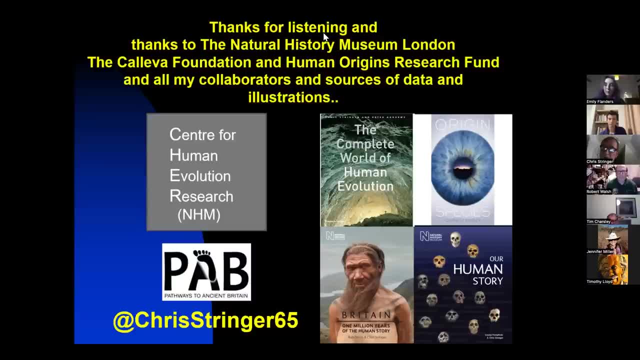 another group of people looked at it and said yes and said yes and said yes, it does show bipedal features. so i think it does show bipedal features. so i think it does show bipedal features. so i think bipedalism would be very important. 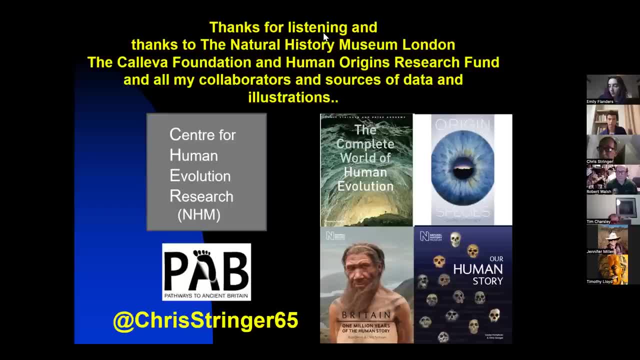 bipedalism would be very important. bipedalism would be very important, um and in terms of um later changes, um and in terms of um later changes um and in terms of um later changes. obviously, um, obviously um, obviously, um. there's this change in in skeletal shape. 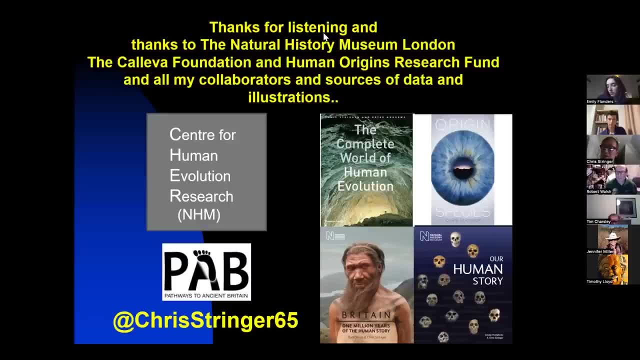 there's this change in in skeletal shape. there's this change in in skeletal shape between uh these earlier humans, such as between uh these earlier humans, such as between uh these earlier humans, such as homo erectus and neanderthals. homo erectus and neanderthals. 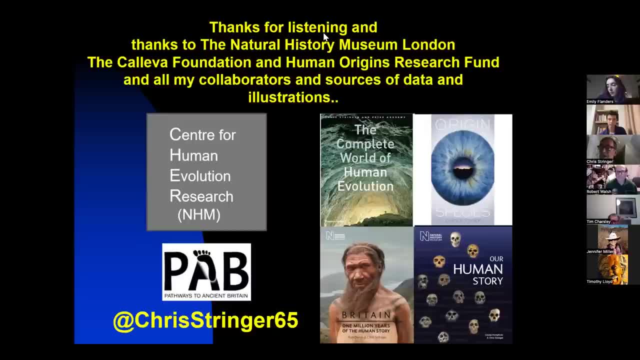 homo erectus and neanderthals, and, and us so and, and us so and and us so it's estimated that our lungs are. maybe it's estimated that our lungs are. maybe it's estimated that our lungs are maybe 20, 20, 20, smaller in capacity compared with uh. 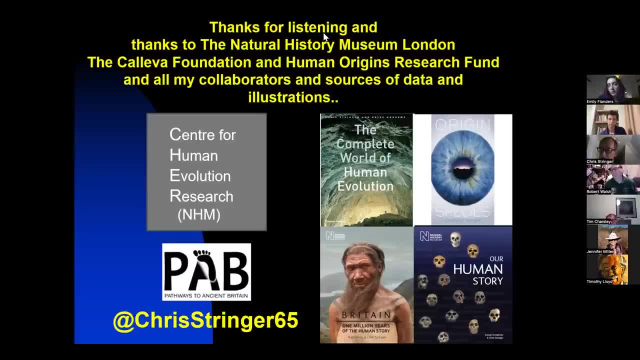 smaller in capacity compared with uh. smaller in capacity compared with uh. erectus and neanderthal lungs. erectus and neanderthal lungs. erectus and neanderthal lungs. the rib cage shows this. so there's, the rib cage shows this. so there's, the rib cage shows this. so there's something distinct there. 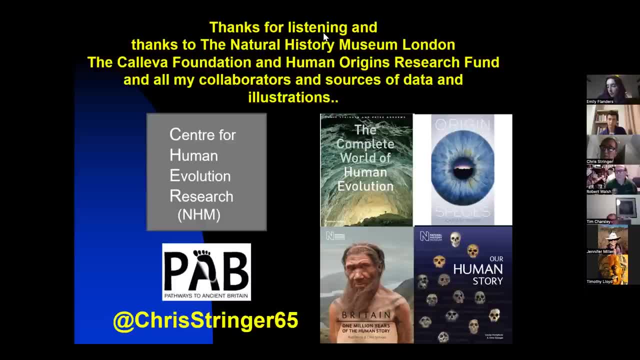 something distinct there, something distinct there physiologically. i guess that you could physiologically. i guess that you could physiologically. i guess that you could argue that, argue that, argue that maybe we're a more efficient model of. maybe we're a more efficient model of. 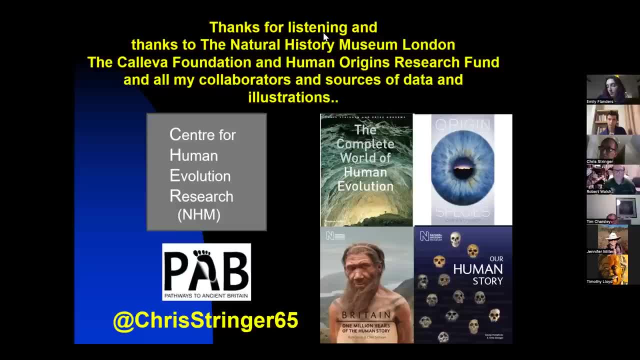 maybe we're a more efficient model of human. we're using less energy. uh, the human we're using less energy. uh, the human we're using less energy. uh, the neanderthals and neanderthals and neanderthals and people like them were having to expend. 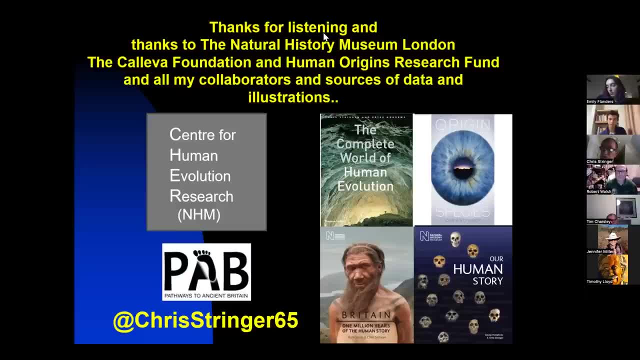 people like them were having to expend. people like them were having to expend a lot, of, a lot of a lot of energy and physical force just in their energy and physical force, just in their energy and physical force, just in their demanding, demanding, demanding everyday activities. and we somehow got. 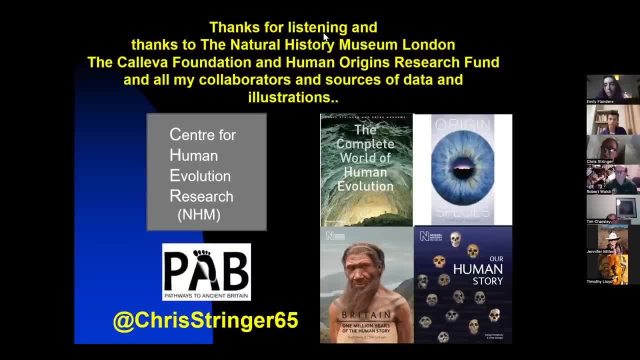 everyday activities and we somehow got everyday activities and we somehow got around this, around this, around this, maybe through our technology uh to maybe through our technology uh to maybe through our technology uh to develop a more economic physiology. and david uh says, and david uh says, and david uh says, there's clearly strong evidence of gene. there's clearly strong evidence of gene. there's clearly strong evidence of gene flow from neanderthals into homo sapiens, flow from neanderthals into homo sapiens, flow from neanderthals into homo sapiens. but can you share your thoughts about? 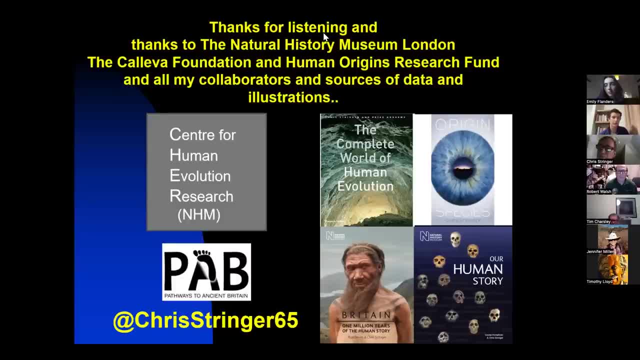 but can you share your thoughts about? but can you share your thoughts about possible gene flow from archaic humans. possible gene flow from archaic humans. possible gene flow from archaic humans into homo sapiens within africa and its. into homo sapiens within africa and its? 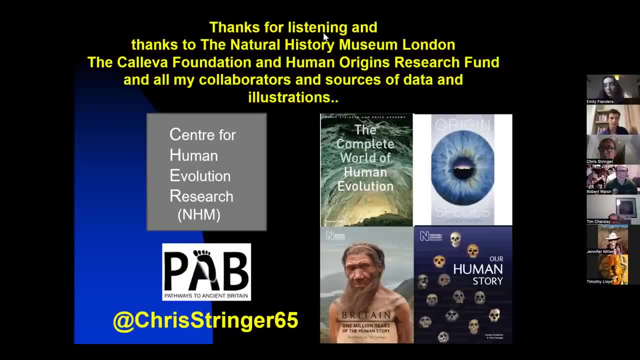 into homo sapiens within africa and its possible role in our evolution- possible role in our evolution. possible role in our evolution- yeah, so, yeah, we really need a geneticist. yeah so yeah, we really need a geneticist. yeah so yeah, we really need a geneticist to talk about that. but, yes, there are. 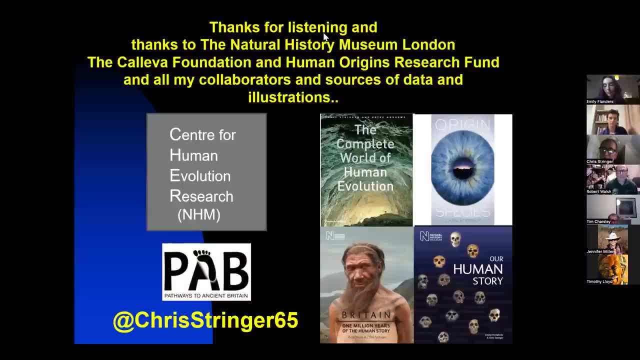 to talk about that. but yes, there are to talk about that. but yes, there are suggestions that, suggestions that, suggestions that you know a comparable time depth, or even you know a comparable time depth, or even you know a comparable time depth, or even greater time depth than greater time depth than. 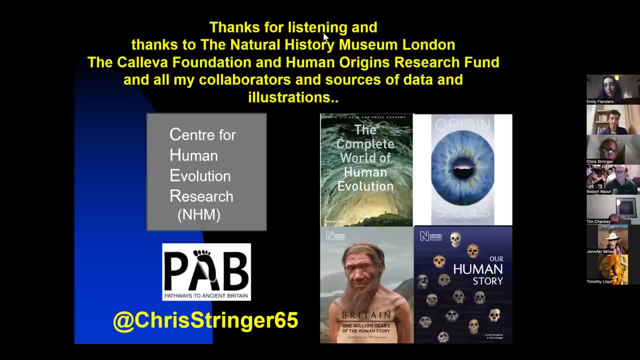 greater time depth than the neanderthal and denisovan. the neanderthal and denisovan, the neanderthal and denisovan populations, populations, populations. so could something like homo hadabagensis, so could something like homo hadabagensis, so could something like homo hadabagensis or homo rhodesiensis? 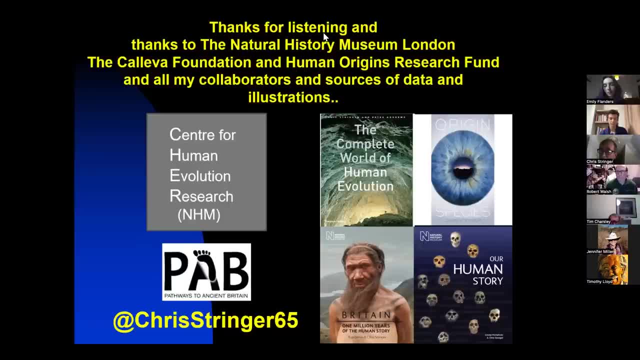 or homo rhodesiensis, or homo rhodesiensis. have survived in in africa um in one of. have survived in in africa um in one of. have survived in in africa um in one of these areas where we we've really got no, these areas where we we've really got no. 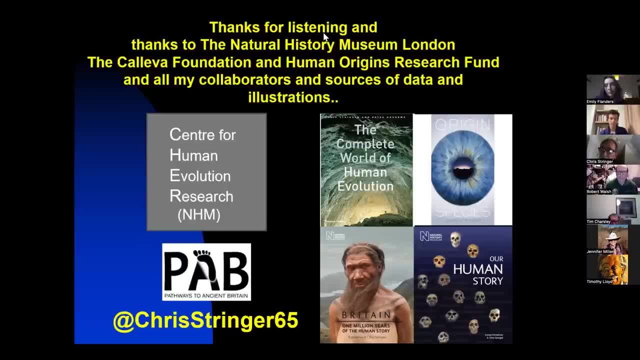 these areas where we we've really got no fossil record- fossil record because the problem is we haven't got, because the problem is we haven't got, because the problem is we haven't got that, that, that ancient genome data yet, and hopefully, ancient genome data yet and hopefully. 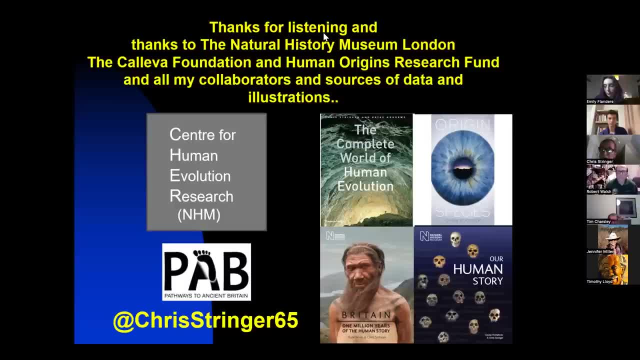 ancient genome data. yet, and hopefully within africa, we will eventually within africa, we will eventually within africa, we will eventually be able to reach to some of these more, be able to reach to some of these more, be able to reach to some of these more ancient populations in africa. 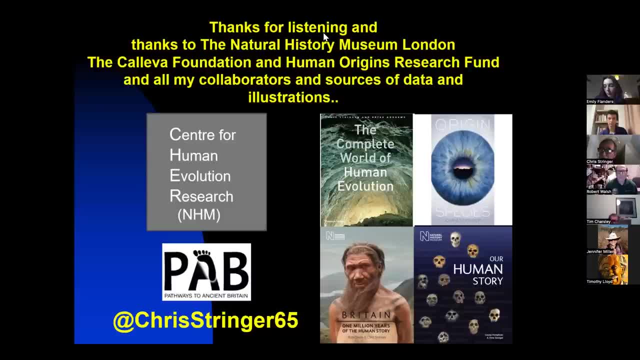 ancient populations in africa, ancient populations in africa, and at least get some genomic data and at least get some genomic data. and at least get some genomic data, maybe in, maybe in, maybe in high altitude sites or deep cave sites, high altitude sites or deep cave sites, high altitude sites or deep cave sites. there will be dna preservation because 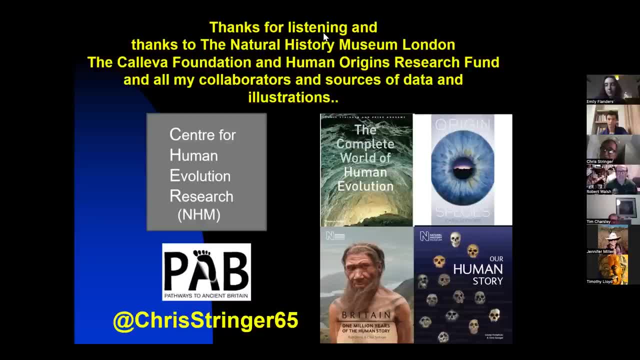 there will be dna preservation. because there will be dna preservation? because in the cement of huesos- i mentioned in the cement of huesos, i mentioned in the cement of huesos, i mentioned- there's dna from 400 000 years ago. there's dna from 400 000 years ago. 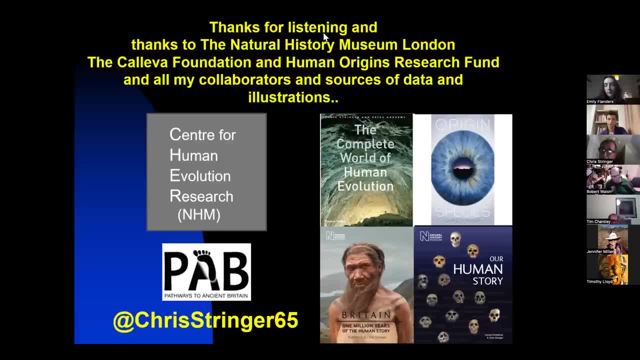 there's dna from 400 000 years ago preserved deep in a cave. maybe in africa preserved deep in a cave, maybe in africa preserved deep in a cave, maybe in africa. there are similar situations and we'll. there are similar situations and we'll. there are similar situations and we'll be able to pick up dna and once we get, 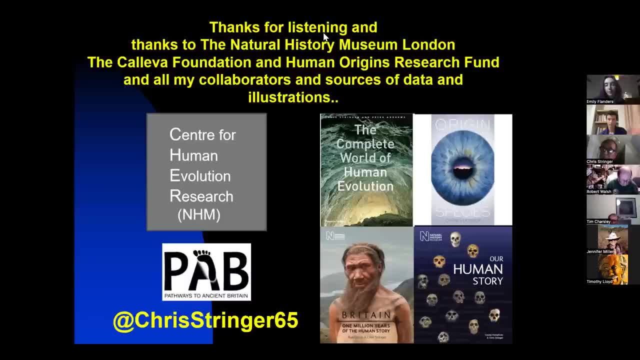 be able to pick up dna. and once we get be able to pick up dna and once we get those ancient genomes, then we'll be in a those ancient genomes, then we'll be in a those ancient genomes, then we'll be in a better position to map whether there is. 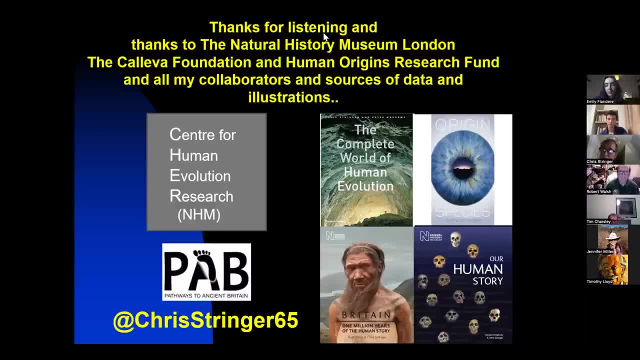 better position to map, whether there is better position to map whether there is integration into recent sub-saharan integration, into recent sub-saharan integration, into recent sub-saharan populations as well as into populations, populations as well as into populations, populations as well as into populations outside of africa. 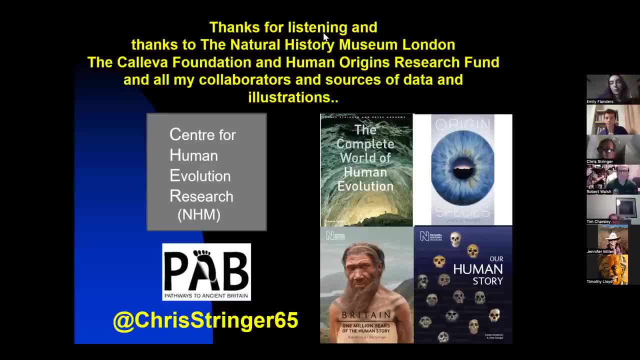 outside of africa. outside of africa, thank you, and i should mention sorry, thank you, and i should mention sorry. thank you and i should mention sorry. yeah, just follow up on that. there is of- yeah, just follow up on that. there is of- yeah, just follow up on that. there is, of course, this intriguing fossil from west. 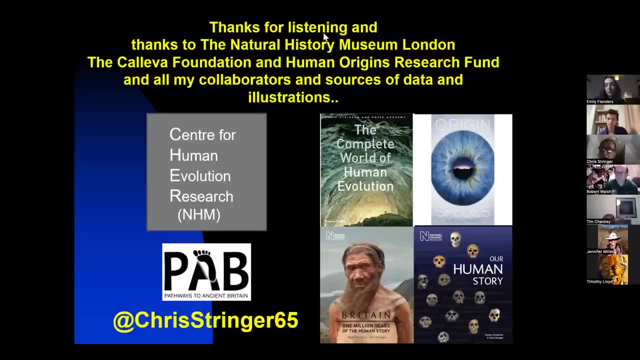 course, this intriguing fossil from west course, this intriguing fossil from west africa, from iho aleru in nigeria, africa. from iho aleru in nigeria, africa. from iho aleru in nigeria. it's maybe 13 000 years old and its. it's maybe 13 000 years old and its. 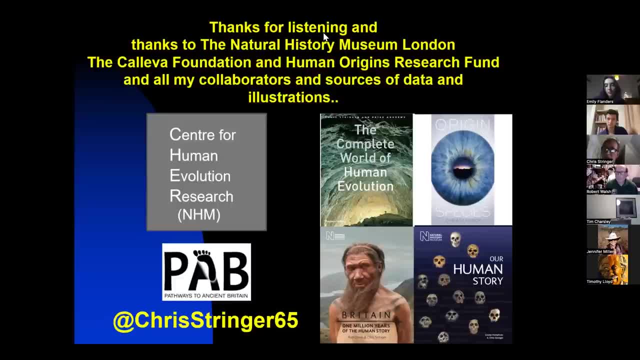 it's maybe 13 000 years old and its cranial vault shape is unlike recent cranial vault shape is unlike recent cranial vault shape is unlike recent african, african, african populations. it looks more basal to use populations. it looks more basal to use populations. it looks more basal, to use my terminology. 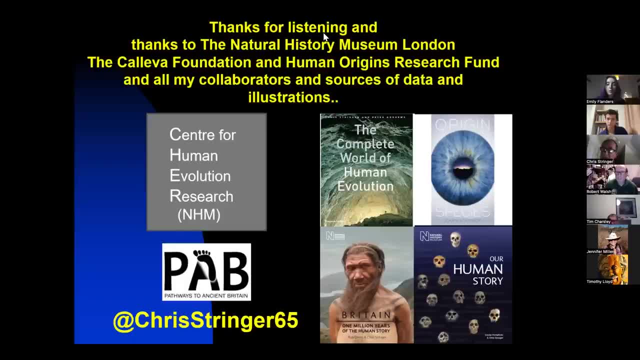 my terminology, my terminology and, and, and. is that an example of a survival of a? is that an example of a survival of a? is that an example of a survival of a basal morphology from early homo sapiens, basal morphology from early homo sapiens. basal morphology from early homo sapiens, or is it evidence, maybe, of? 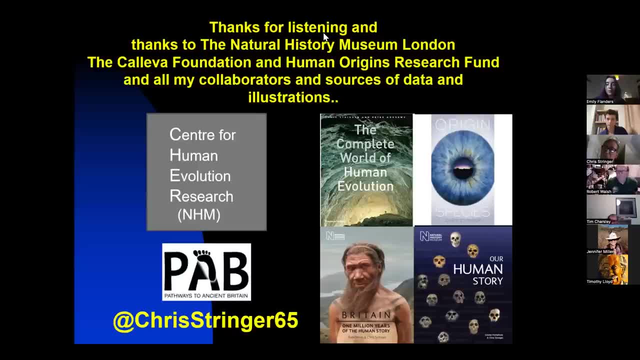 or is it evidence maybe of, or is it evidence maybe of introgression, introgression, introgression into homo sapiens producing that, more into homo sapiens producing that, more into homo sapiens producing that more basal cranial shape. so, yes, there are basal cranial shape. so, yes, there are. 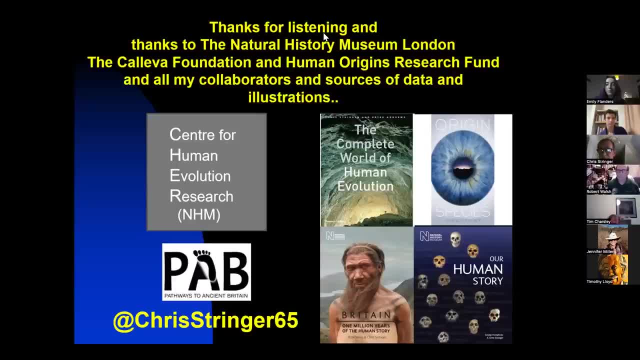 basal cranial shape. so yes, there are some hints of that even in the fossils. some hints of that even in the fossils, some hints of that even in the fossils. and i realized i skipped robert's and i realized i skipped robert's and i realized i skipped robert's question. uh, 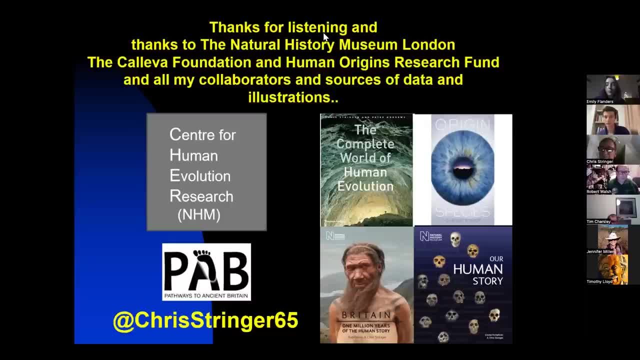 question uh, question, uh. if you'd like to to read that out, or if you'd like to to read that out, or if you'd like to to read that out, or ask out loud, ask out loud, ask out loud. yes, can you hear me? yes, can you hear me? 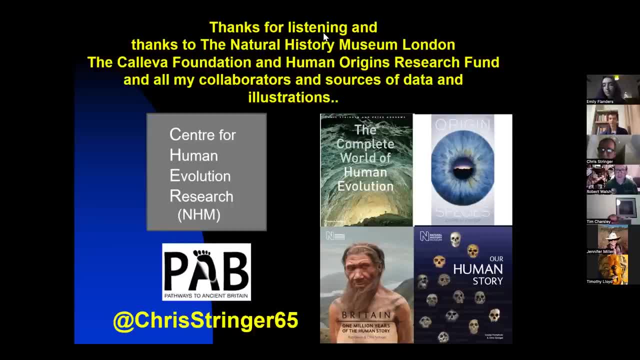 yes, can you hear me? yeah, yeah, yeah, right hi chris. uh, great talk as ever. right hi chris? uh, great talk as ever. right hi chris? uh, great talk as ever. um. i was just wondering, how do you think? um, i was just wondering, how do you think. 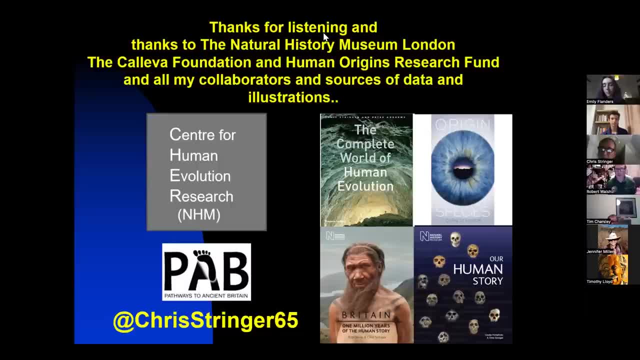 um, i was just wondering how do you think homo intercessor now fits into the human homo intercessor now fits into the human homo intercessor now fits into the human evolution pattern, evolution pattern, evolution pattern. um, um, um, this is a dead end species, or could it? 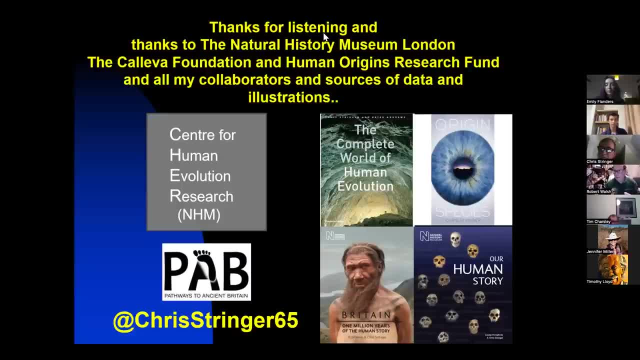 this is a dead end species, or could it? this is a dead end species, or could it have contributed towards? have contributed towards? have contributed towards? um certainly neanderthal's evolution. i um certainly neanderthal's evolution, i um certainly neanderthal's evolution, i mean. 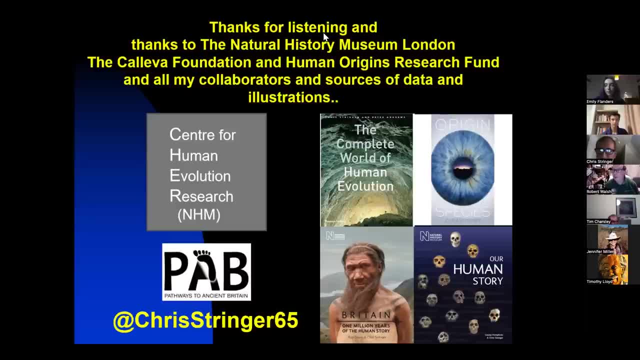 mean mean, yes, homo, which homo was that robert? uh, yes, homo, which homo was that robert? uh, yes, homo, which homo was that robert uh, homo intercessor, homo intercessor, homo intercessor, intercessor. yeah, yeah, so um. intercessor. yeah, yeah, so um. 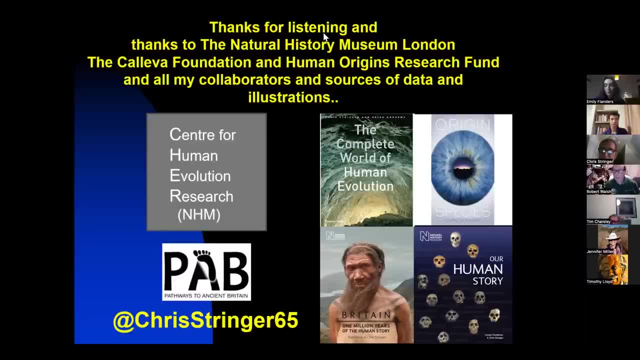 intercessor: yeah, yeah, so, um, yeah, i i think antecessor in terms of: yeah, i i think antecessor in terms of: yeah, i i think antecessor in terms of facial morphology, facial morphology, facial morphology: uh, antecessor, looks closer to the. 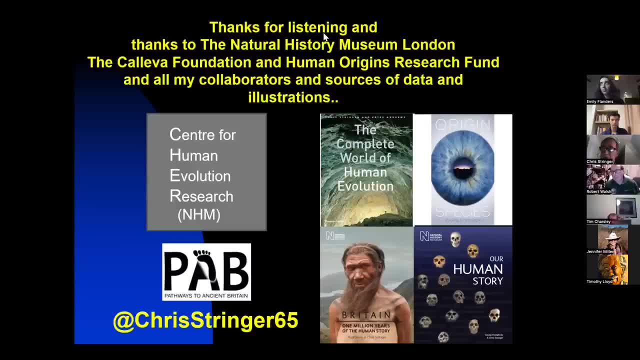 uh antecessor looks closer to the uh antecessor looks closer to the inferred common ancestor. i think now of inferred common ancestor. i think now of inferred common ancestor. i think now of us in neanderthals and denisovans, us in neanderthals and denisovans. 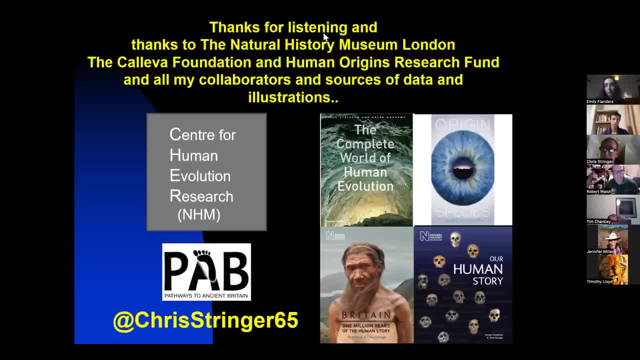 us in neanderthals and denisovans, so um, so, um, so um. it depends, it depends, it depends. you know, as i say, where we place that. you know, as i say, where we place that. you know, as i say where we place that common ancestor and where we place it in. 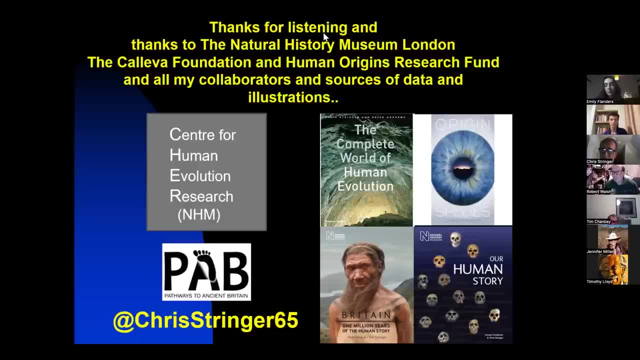 common ancestor and where we place it in. you know, as i say, where we place it in: time as well as geography. so antecessor time as well as geography. so antecessor time as well as geography. so antecessor could be close to the ancestral. 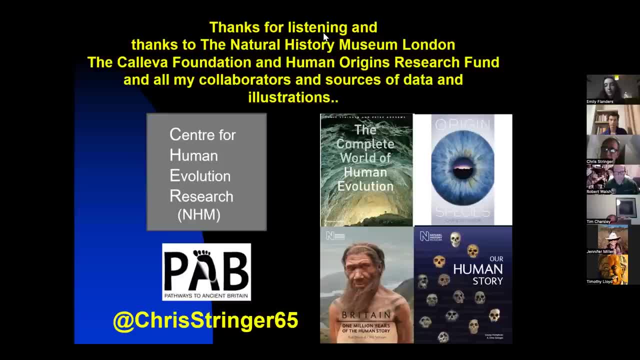 could be close to the ancestral, could be close to the ancestral: morphology, morphology, morphology- but of course we don't. but of course we don't, but of course we don't know a lot about it. it's only known from. know a lot about it. it's only known from. 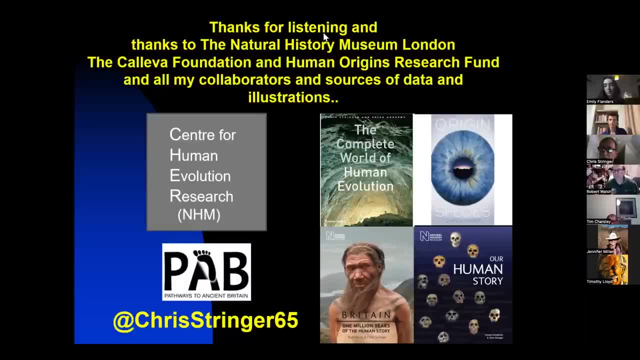 know a lot about it. it's only known from one site. one site. one site at one time period- uh, we don't know how. at one time period, uh, we don't know how. at one time period, uh, we don't know how widely it ranged- widely it ranged. 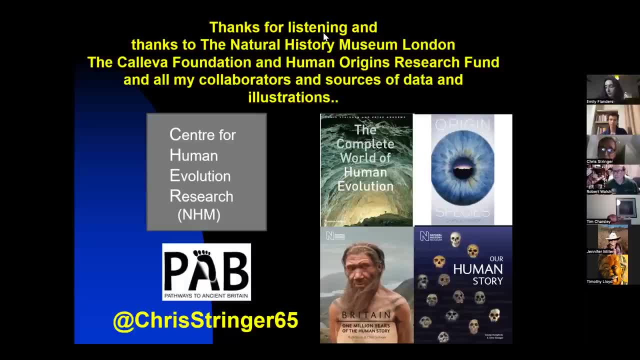 widely. it ranged uh, but i think that it it perhaps is uh, but i think that it it perhaps is uh, but i think that it it perhaps is closer to, closer to, closer to. it will come lovely. thank you, chris. it will come lovely. thank you, chris. 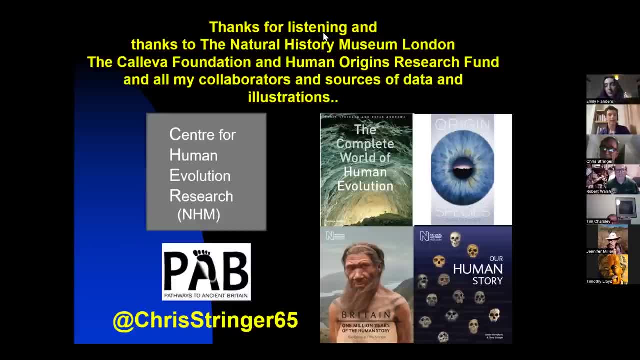 it will come lovely. thank you, chris. and so we've we've got two questions, and so we've we've got two questions, and so we've we've got two questions left, left, left. so james wants to know um he says: how do? so james wants to know um, he says: how do? 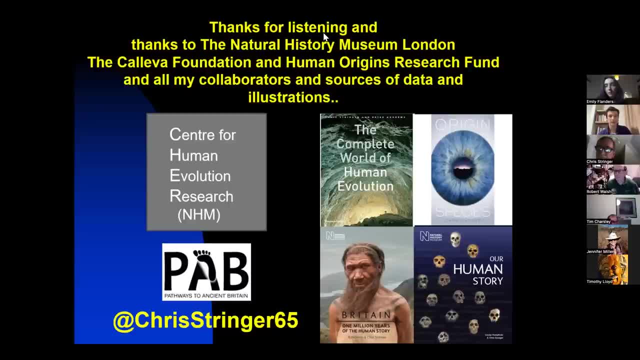 so james wants to know um. he says: how do you currently see the relationship? you currently see the relationship. you currently see the relationship between european and african specimens, between european and african specimens, between european and african specimens that fall outside of the variation on, that fall outside of the variation on. 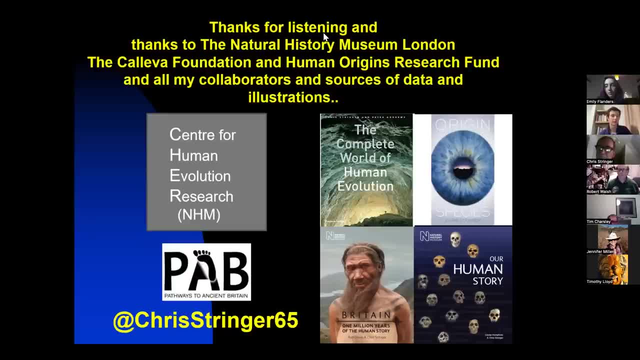 that fall outside of the variation on the neanderthal and sapiens lineage and the neanderthal and sapiens lineage and the neanderthal and sapiens lineage and that used to be grouped together as that used to be grouped together as that used to be grouped together as heel bergensis, do you think we're in a? 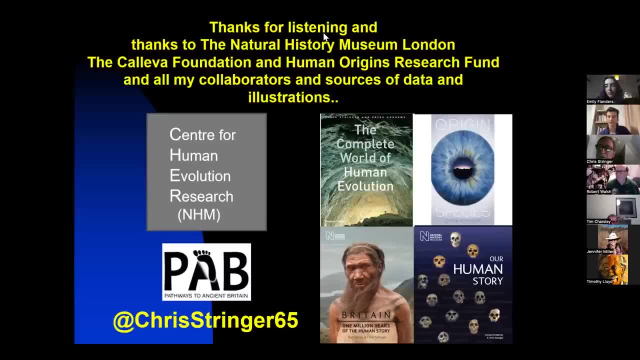 heel bergensis. do you think we're in a heel bergensis? do you think we're in a position to count them as two different position? to count them as two different position, to count them as two different species. species species- yeah, that's um. yeah, that's um. 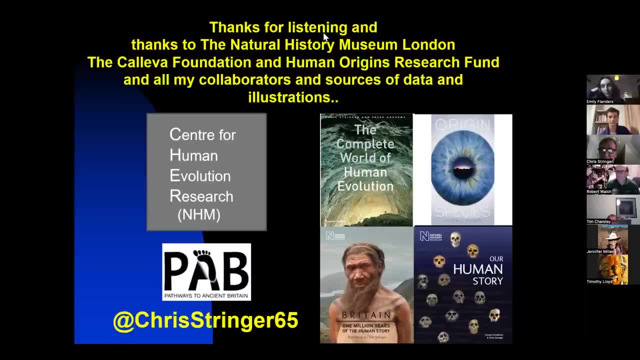 yeah, that's um, yeah, that's a tricky one. so yeah, that's a tricky one. so yeah, that's a tricky one. so i think that, i think that i think that if we look at things like petrolona, and if we look at things like petrolona and 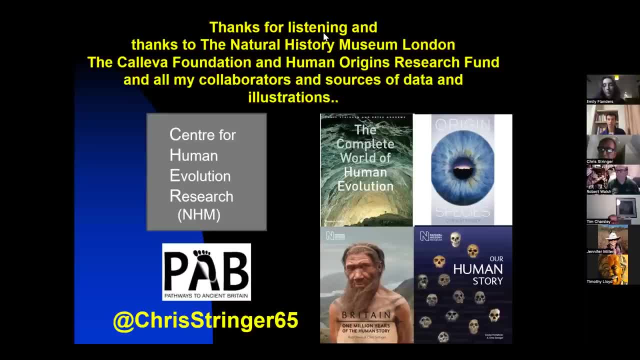 if we look at things like petrolona and broken hill, broken hill, broken hill to me. they are to me, they are to me. they are similar enough to be grouped together as a. similar enough to be grouped together as a to me, they are similar enough to be grouped together as a, as a single species, whether we 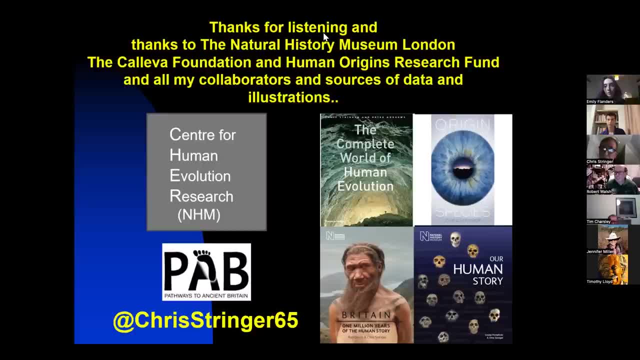 as a single species, whether we as a single species, whether we call that hydra bergensis, or call that hydra bergensis, or call that hydra bergensis or rhodesiensis and i'm tending more rhodesiensis and i'm tending more. 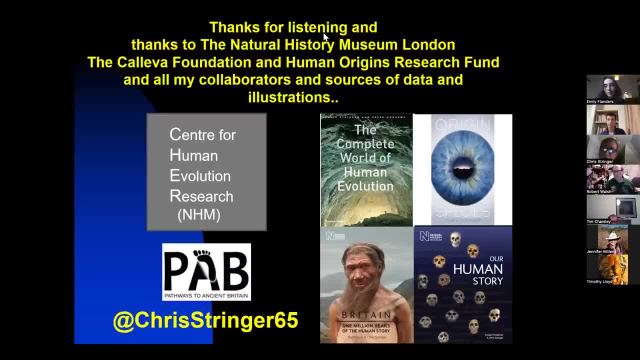 rhodesiensis, and i'm tending more towards the rhodesiensis name now, towards the rhodesiensis name now, towards the rhodesiensis name now. but there are other fossils which don't. but there are other fossils which don't. but there are other fossils which don't fit so easily or are less complete, and 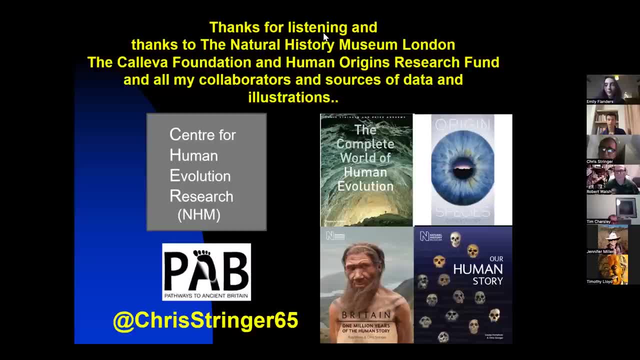 fit so easily or are less complete. and fit so easily or are less complete, and we can't place them so well. we can't place them so well, we can't place them so well. so, um, so, um, so um, i'm not sure. uh, what to do with the male. 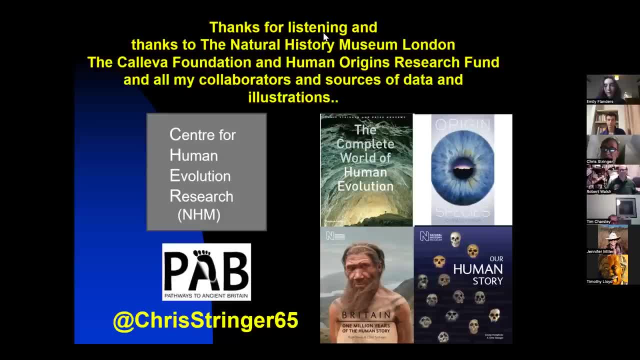 i'm not sure, uh, what to do with the male. i'm not sure, uh, what to do with the male mandible, for example. i mean it's the type mandible, for example. i mean it's the type mandible, for example, i mean it's the type of homo hydra bergensis. 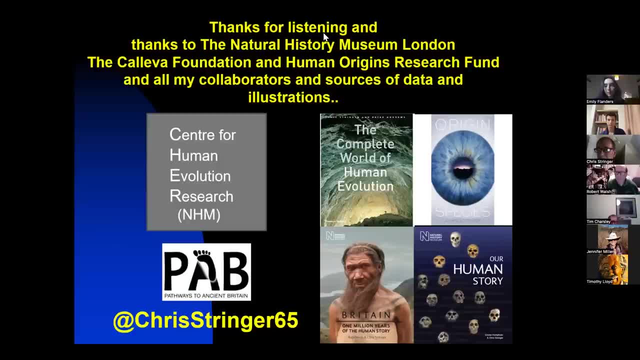 of homo hydra bergensis, of homo hydra bergensis, but it doesn't look like the sema fossils, but it doesn't look like the sema fossils, but it doesn't look like the sema fossils which, which which look like the early neanderthals, um and. 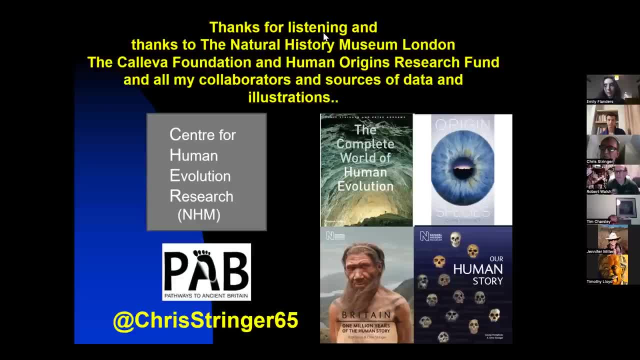 look like the early neanderthals um, and look like the early neanderthals um, and it doesn't actually. it doesn't actually, it doesn't actually match some of the other mandibles. we've match some of the other mandibles. we've match some of the other mandibles we've got from. 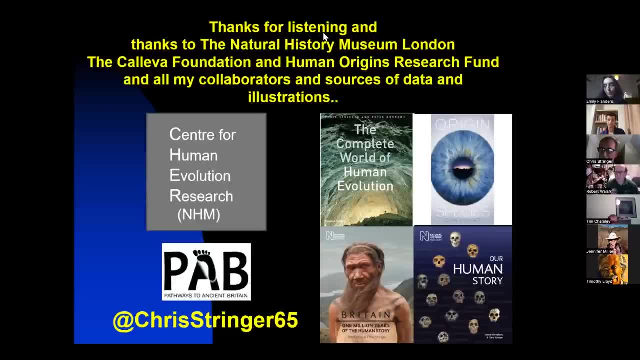 got from, got from from the middle pleistocene from other, from the middle pleistocene from other, from the middle pleistocene from other regions. so mauer regions, so mauer regions, so mauer kind of stands out, maybe the malala kind of stands out, maybe the malala. 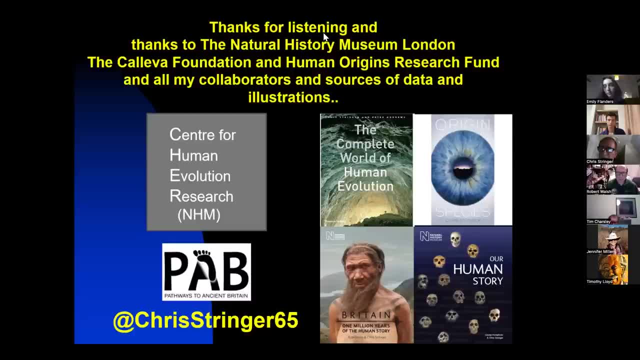 kind of stands out. maybe the malala balanica specimen, balanica specimen, balanica specimen might be related to mauer. that's a might be related to mauer. that's a might be related to mauer. that's a possibility, but that's an isolated. 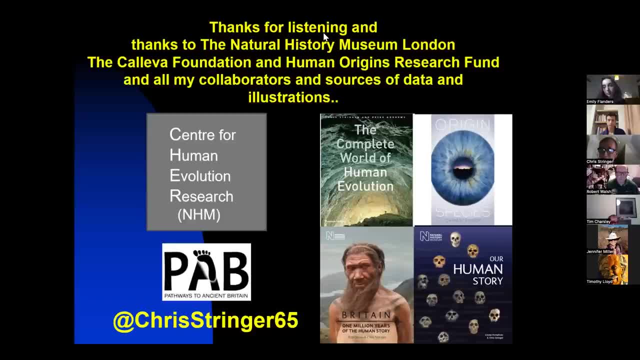 possibility, but that's an isolated possibility. but that's an isolated specimen, specimen, specimen. um cheprano is an interesting fossil. um cheprano is an interesting fossil. um cheprano is an interesting fossil, which, which, which, in some ways it looks like the, in some ways it looks like the. 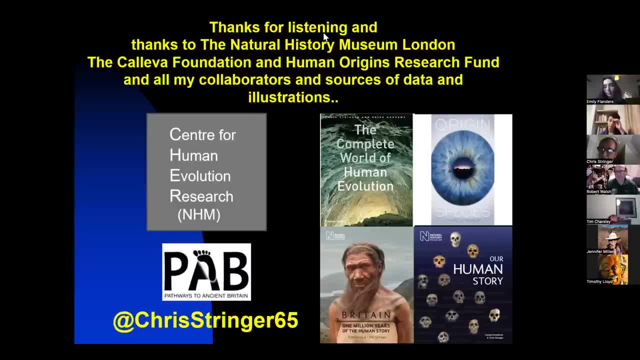 in some ways it looks like the heidelbergensis rhodesiensis, heidelbergensis rhodesiensis, heidelbergensis rhodesiensis: morphology, but morphology, but morphology, but. but in other ways doesn't fit so well it, but in other ways doesn't fit so well it. 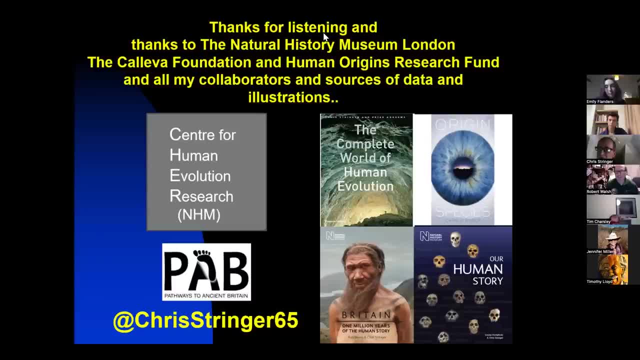 but in other ways doesn't fit so well. it seems to be, seems to be. seems to be in some ways more primitive. so, uh, even in some ways more primitive. so uh, even in some ways more primitive. so, uh, even though it's dated, though it's dated. 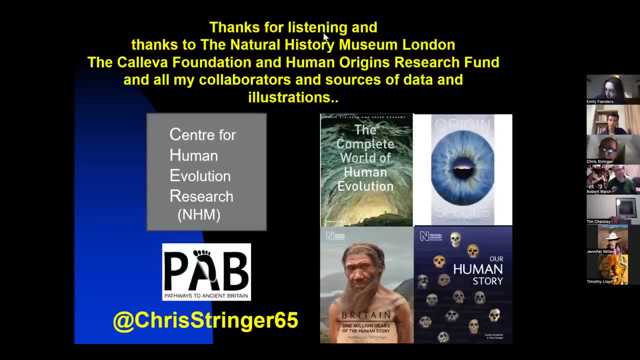 though it's dated. apparently now quite young, apparently now quite young, apparently now quite young. maybe close to 400 000 years old. so maybe close to 400 000 years old. so maybe close to 400 000 years old. so similar in age to the sema material it. 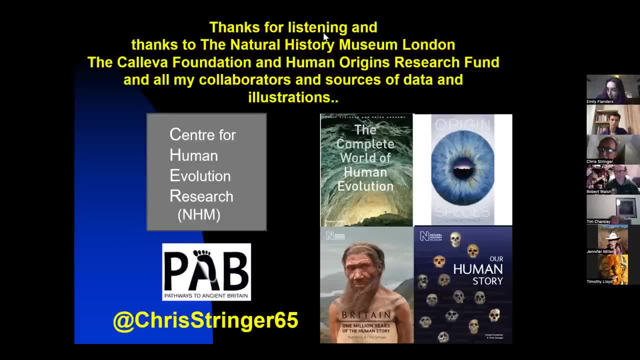 similar in age to the sema material. it similar in age to the sema material. it seems, and yet seems, and yet seems, and yet much more primitive. so i don't really much more primitive, so i don't really much more primitive, so i don't really know for sure where. 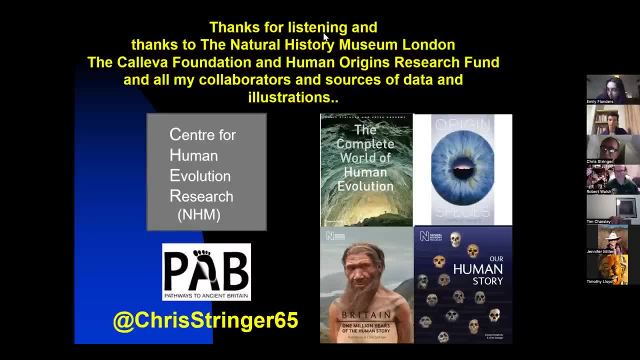 know for sure where, know for sure where chaparano fits into the pattern now. so chaparano fits into the pattern now. so chaparano fits into the pattern now. so, um, yeah, there are fossils which don't. um, yeah, there are fossils which don't. 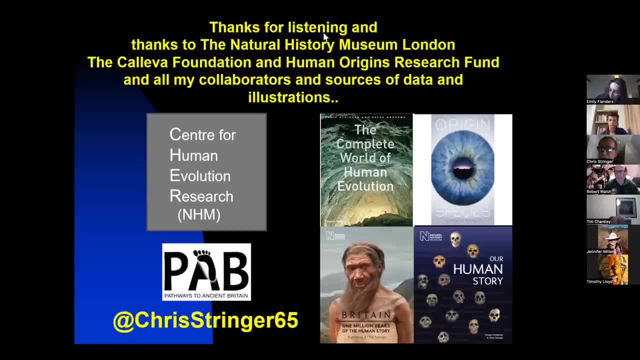 um, yeah, there are fossils which don't fit so well, fit so well, fit so well, and in africa too, of course, and in africa too, of course, and in africa too, of course. fragmentary fossils, some of the north fragmentary fossils, some of the north fragmentary fossils, some of the north african fossils, such as. 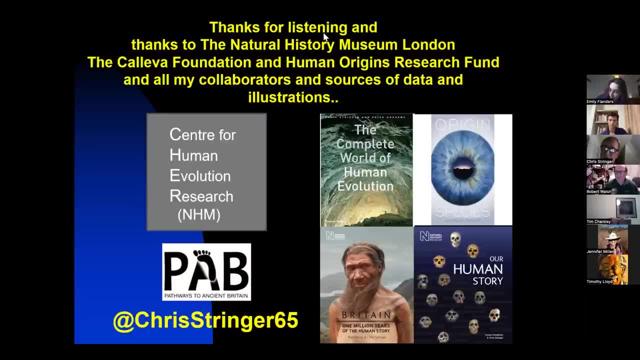 african fossils, such as african fossils such as sale, difficult to place that in the uh sale. difficult to place that in the uh, in the in the bigger picture, in the in the in the bigger picture, in the in the in the bigger picture. yeah, so still many questions remaining. 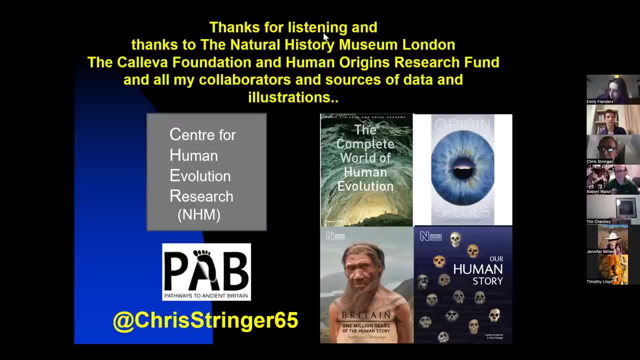 yeah, so still many questions remaining. yeah, so still many questions remaining. yeah, thank you, and uh one final question by thank you and uh one final question by thank you, and uh one final question by catherine. i'm not sure if she catherine, i'm not sure if she. 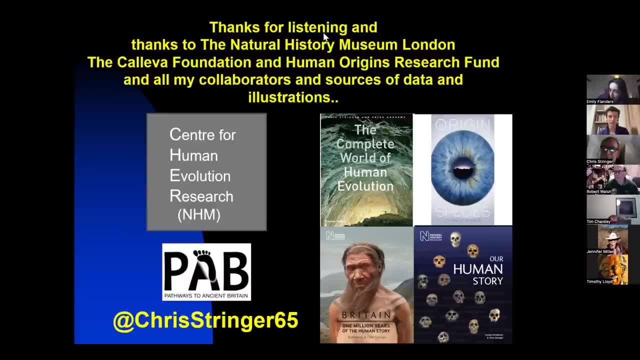 catherine, i'm not sure if she wants to read it out, or if wants to read it out, or if wants to read it out, or if i should, i should, i should. all right, i'll, i'll just read it out. all right, i'll, i'll just read it out. 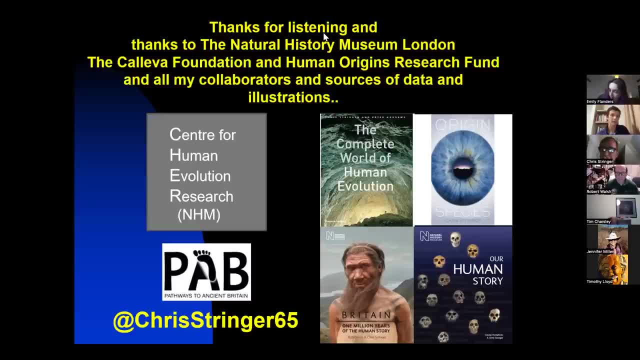 all right, i'll. i'll just read it out: um so catherine says. do you think? um so catherine says: do you think? um so catherine says: do you think? transmission of infectious disease. transmission of infectious disease. transmission of infectious disease between sapiens and neanderthals. 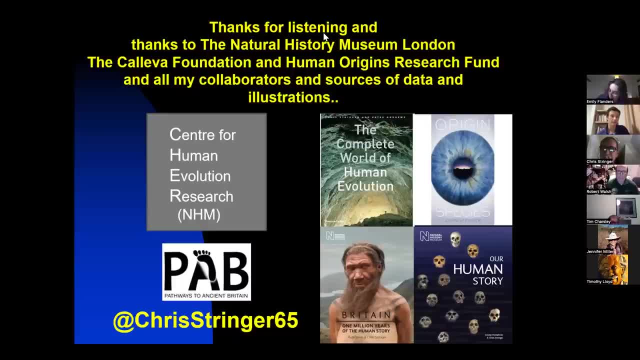 between sapiens and neanderthals- between sapiens and neanderthals- could have had a significant could have had a significant, could have had a significant contribution to neanderthal extinction. contribution to neanderthal extinction. contribution to neanderthal extinction when combined with the effects of 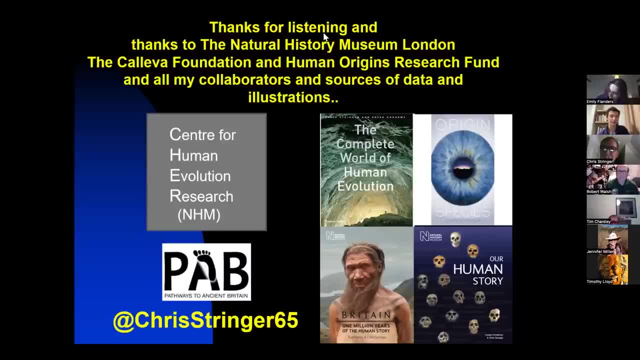 when combined with the effects of. when combined with the effects of inbreeding and small population size: inbreeding and small population size, inbreeding and small population size, genetic diversity, genetic diversity, genetic diversity. yeah, interesting question and some people. yeah, interesting question and some people. yeah, interesting question and some people have raised that. that of course have raised that, that of course have raised that, that of course we would have come from africa. possibly we would have come from africa. possibly we would have come from africa, possibly transmitting diseases, transmitting diseases, transmitting diseases which the neanderthals had no natural. which the neanderthals had no natural, which the neanderthals had no natural immunities to, immunities to, immunities to, and that could have affected them equally and that could have affected them equally and that could have affected them equally. it's been positive the other way around. 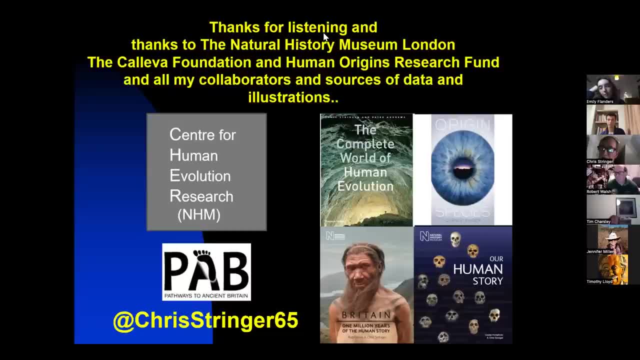 it's been positive the other way around. it's been positive the other way around. of course that we came out of africa. and of course that we came out of africa. and of course that we came out of africa and had no, had, no, had no natural immunity to the local diseases. natural immunity to the local diseases. natural immunity to the local diseases. which is why interbreeding with? which is why interbreeding with, which is why interbreeding with neanderthals was advantageous. because we neanderthals was advantageous. because we neanderthals was advantageous? because we got a quick fix to our immune systems. 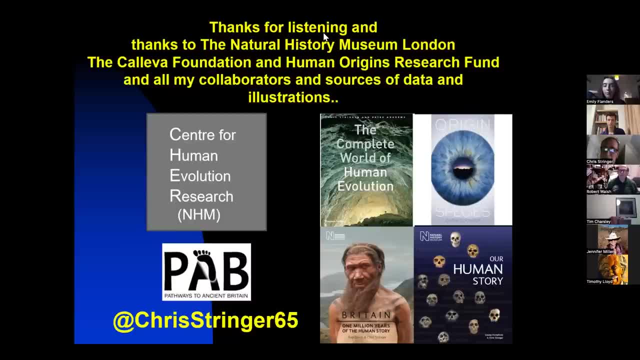 got a quick fix to our immune systems. got a quick fix to our immune systems. so the spread of infectious diseases. so the spread of infectious diseases. so the spread of infectious diseases has been suggested. it's possible that it has been suggested. it's possible that it has been suggested. it's possible that it had a role. 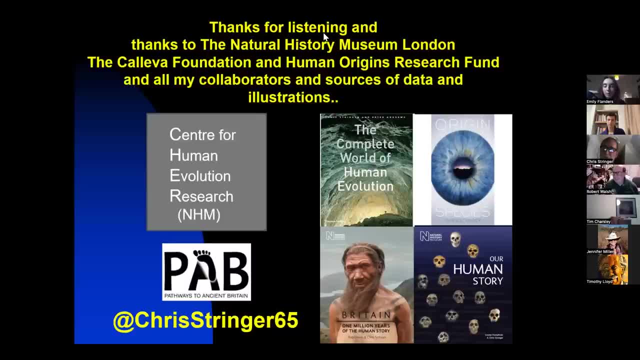 had a role, had a role. i think, when we look at examples in i think when we look at examples in i think when we look at examples in recent history, recent history, recent history, those spreads have been, those spreads have been, those spreads have been in really quite dense population areas. 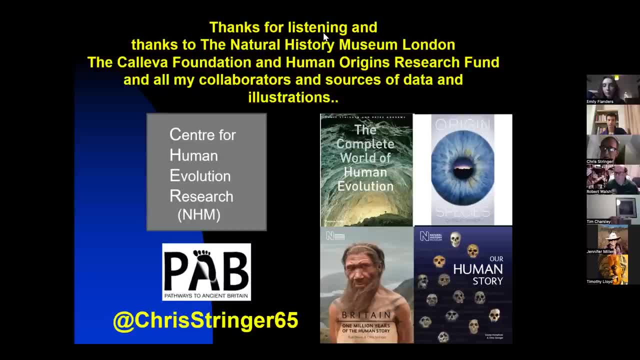 in really quite dense population areas, in really quite dense population areas. so the transmission, so the transmission, so the transmission could be high in in urban areas and could be high in in urban areas and could be high in in urban areas, and obviously neanderthals and homo sapiens. 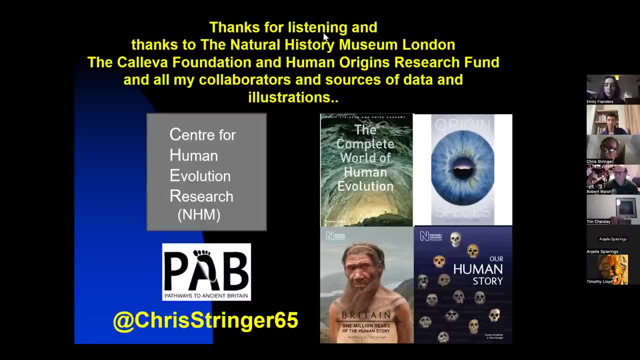 obviously neanderthals and homo sapiens. obviously neanderthals and homo sapiens 40, 50 000 years ago lived in small 40. 50 000 years ago lived in small 40. 50 000 years ago lived in small scattered groups. so i don't know whether 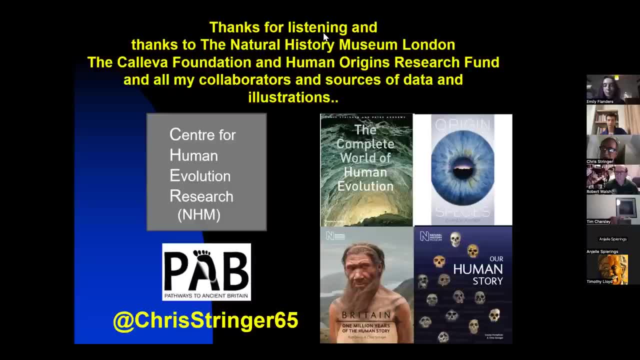 scattered groups. so i don't know whether scattered groups, so i don't know whether the transmission could have been, the transmission could have been, the transmission could have been sufficient to be that damaging, sufficient to be that damaging, sufficient to be that damaging. it's certainly a possibility. 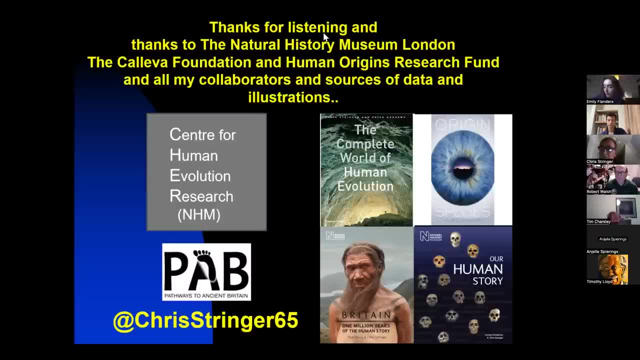 it's certainly a possibility. it's certainly a possibility, but i think the evidence you know is, but i think the evidence you know is, but i think the evidence you know is isn't there at the moment. people have isn't there at the moment. people have isn't there at the moment. people have suggested that certainly. 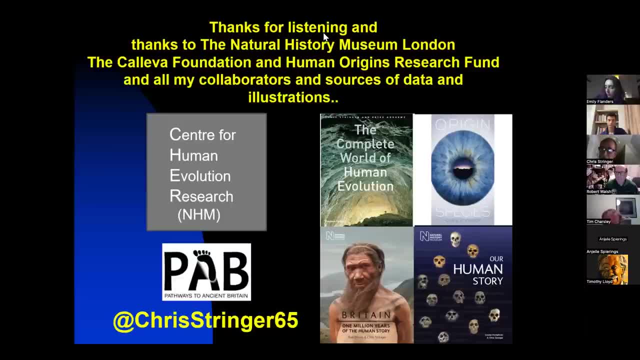 suggested that, certainly, suggested that certainly in western asia it could have been a in western asia. it could have been a in western asia. it could have been a factor there, when these populations first factor there, when these populations first factor there, when these populations first came into contact with each other.